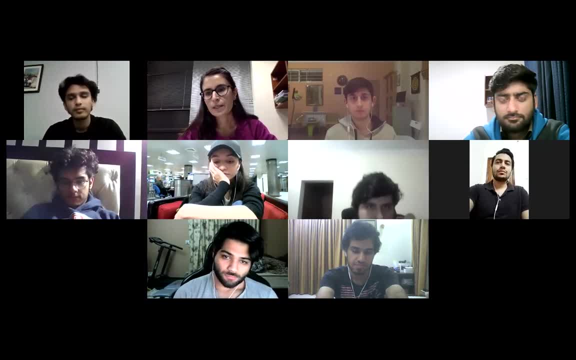 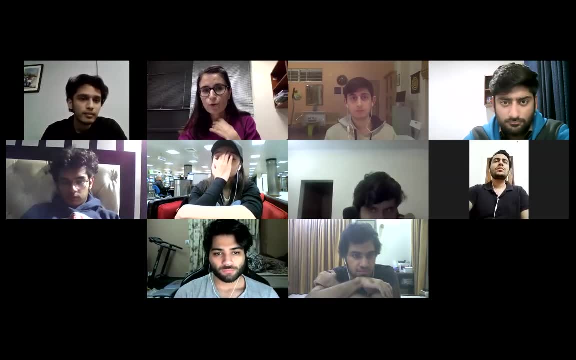 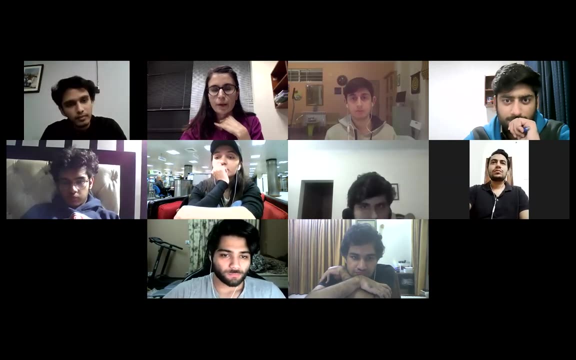 bring it back and uh, and try and learn it. all right, um, so, but but like, think out of the box, don't, don't think traditionally, and if i've missed something and you know it, and if you have any ideas, even if it's a wild idea, um, just just throw it, um in in, like raise your hand. 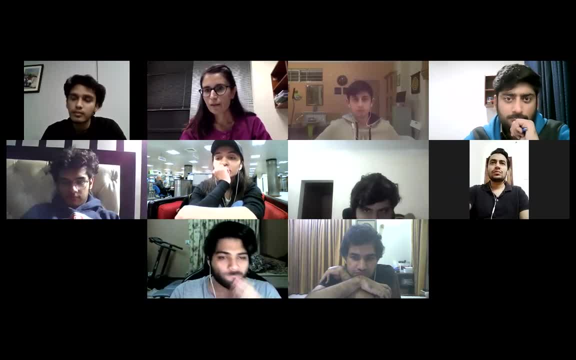 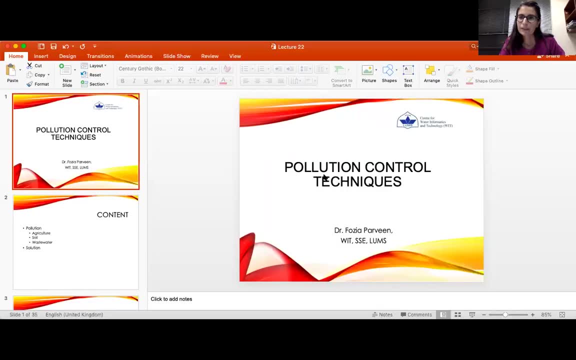 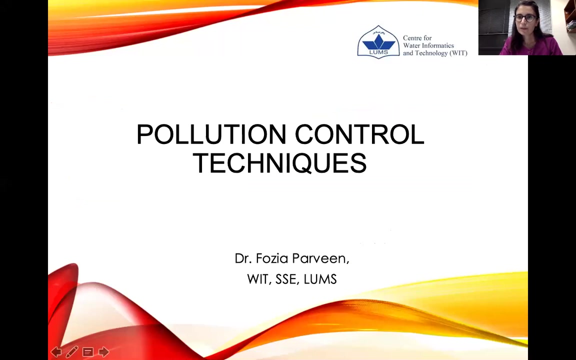 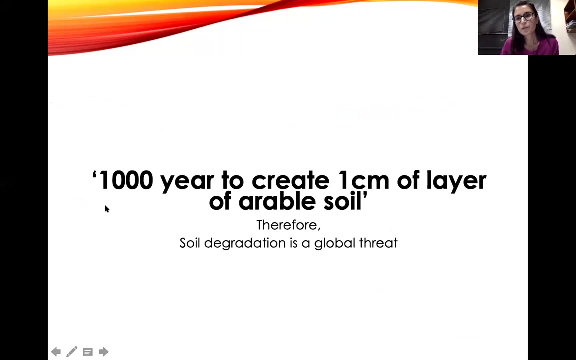 and share it with your class, and i think that'll be very, very interesting. so let's not waste any time and stop the presentation, okay, so the reason why i started with soil pollution was, or soil pollution control techniques was because we studied agriculture recently and i thought the knowledge would be a little fresh with you, and we have just. 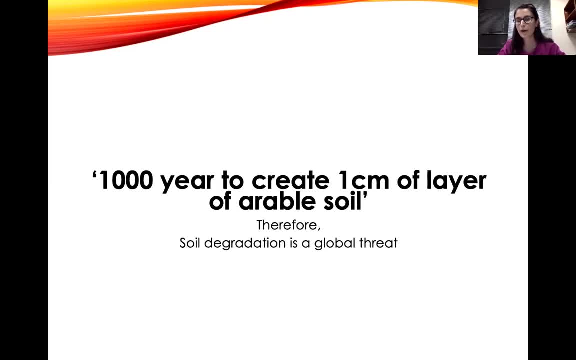 discussed them from time to time, so i thought it would be better to start with that. and again, i would expect or ask you to give me a few solutions, because we've already discussed them with reference to agriculture in our previous lectures. we care about this resource because 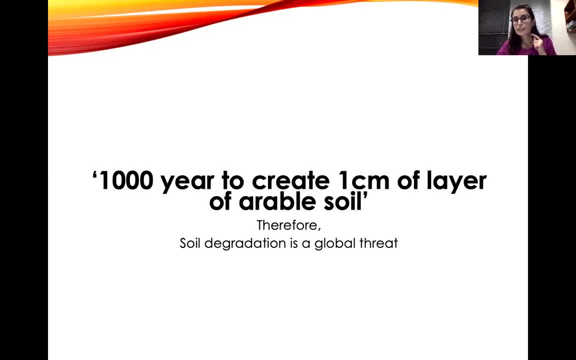 although it's renewable, it's it takes a lot of time for for a layer of soil to be formed, for a layer of edible soil to be formed, which means that if there is any oil or hydrocarbon pollution or any other form of heavy metal and industrial waste, uh contamination on the soil. 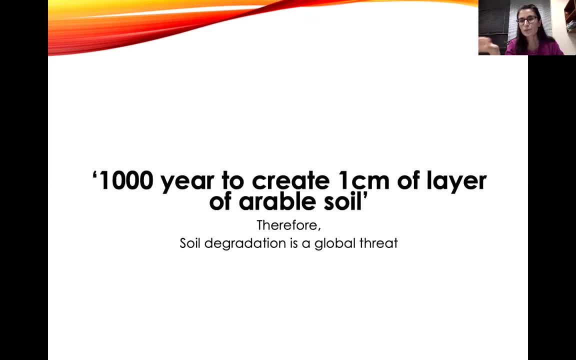 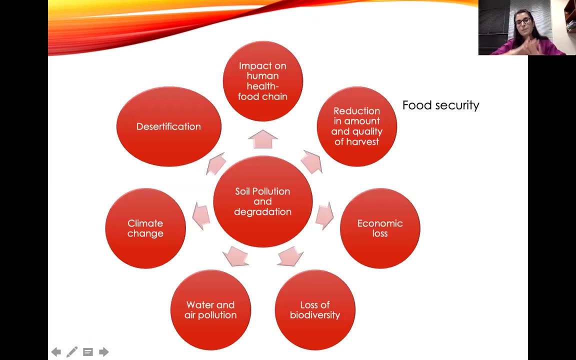 and that top soil, which is important for agriculture, is damaged. it basically hampers a lot of other things for the planet, not just for the wildlife, but also for us, because our food security depends on this natural resource and we care about it because it impacts so many other things. if the soil is degraded, if the soil is polluted- okay, why don't i throw? 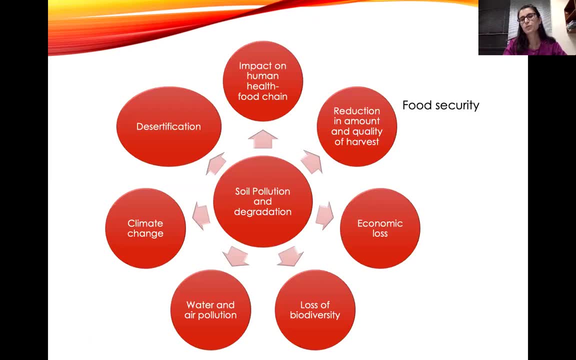 this question to you: if the soil is polluted, what kind of impact would you see around you? and you can use this information that i've put in to as a key. if you want to talk about it, just raise your hand and then discuss. daniel, we would not be able to use it for agricultural purposes if it's polluted, exactly. 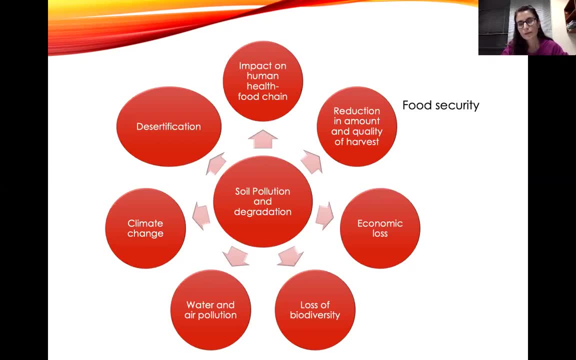 um, daniel already mentioned my point, but i'd like to go go into much more detail. so, um, i'll leave it to you, but i want to focus on the other side. so, um, so, uh, what i just said is that i would like to just give an example of our agricultural 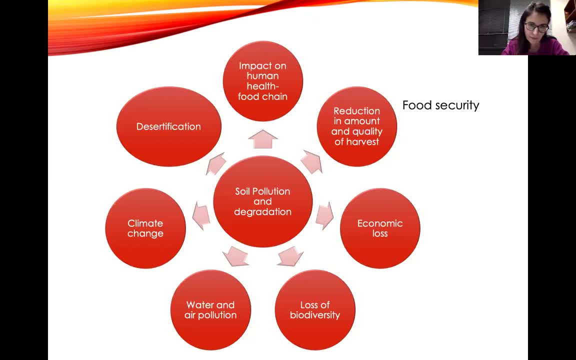 industry a little bit. what i would like to show you is a really important thing and what i've learned- and i've seen a lot of people also for a number of years. i want to give a little bit more of a context of the real world because, you can see, this is the general. 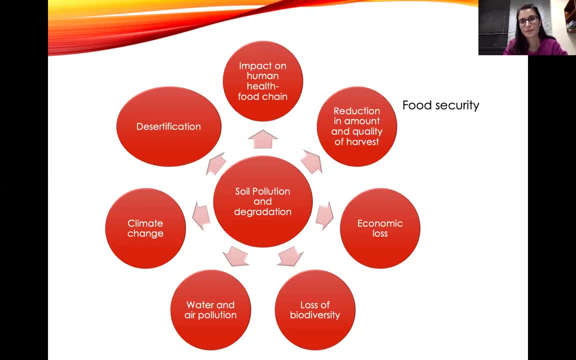 biggest exports would drop drastically. a current account deficit will rise up dramatically. absolutely, party amen. I feel, like you know, quality of nutrition would be affected and, apart from that, since we can consuming unhealthy crops right, that won't be, you know, healthy in the longer run of things, because it 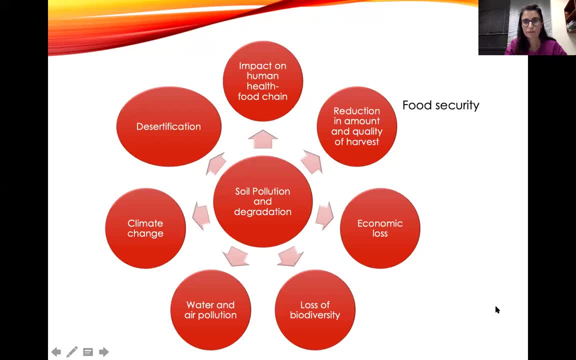 would affect our- you know, for instance, our- digestive system. so you know internal systems. yeah, yeah, so the food chain- any pollutant becoming a part of a food chain would impact all the living beings on the planet. I mean, my point was similar to what I think even talked about, so I mean I 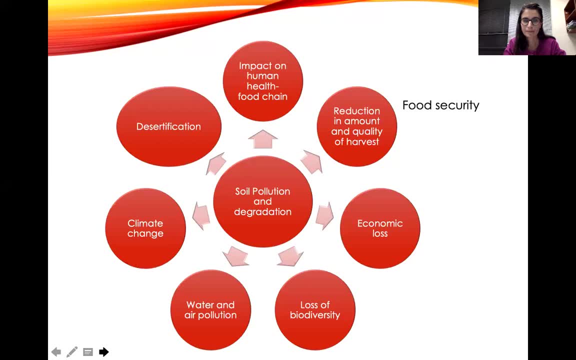 wanted to say that the pollutants in the soil, particularly they, enter into the food chain and they can result in many diseases and excess mortality in humans as well, and it can have both short-term and long-term effects. and long-term effects. may I remember reading somewhere that it can? 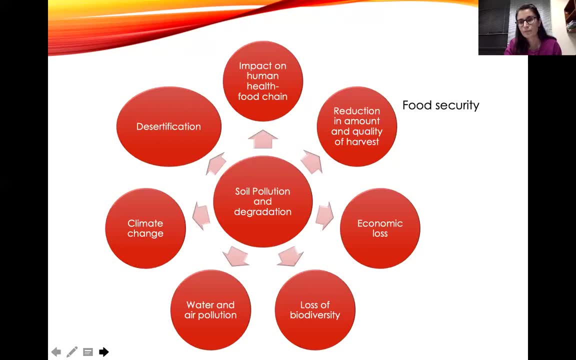 actually lead to cancer, so it's actually very harmful. absolutely female. I had a point a. degraded lands are often less able to hold the water, which can even personally flooding and increase the chances of flooding, and which can have further consequences after. yes, that is great, Hassan Shahid. I thought that from. 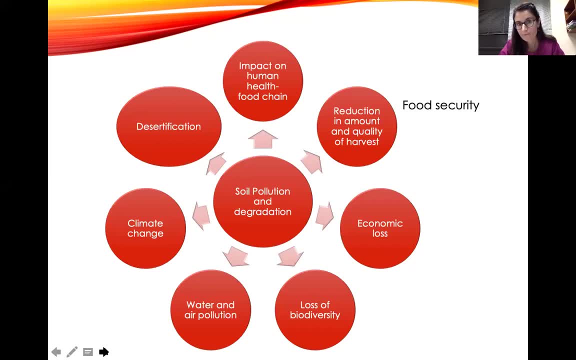 the economic point of view, that if the soil is polluted, then if we think about it from a construction point of view, that if we like construct a house, so that the house or any sort of building can they, it can like kharab wo jo hai, wo zameen ke undar ja sakti hai. toh isna ka main point tha, mera diman. 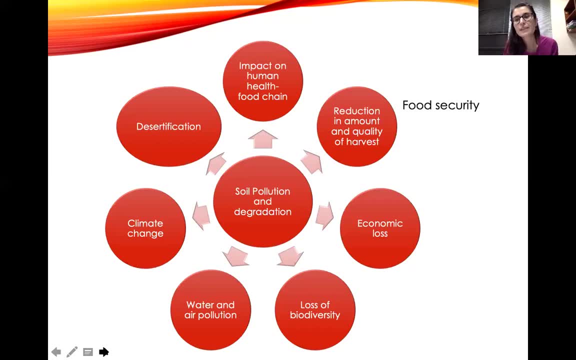 yes, yeah, yeah, yeah. so you, and then you know, there are other things that we've discussed, by the way, which is that if, for example, soil is degraded, if agriculture is not practiced properly, if the soil quality has degraded and plants cannot grow there, if our practices are not right, then what happens? is it impacts. 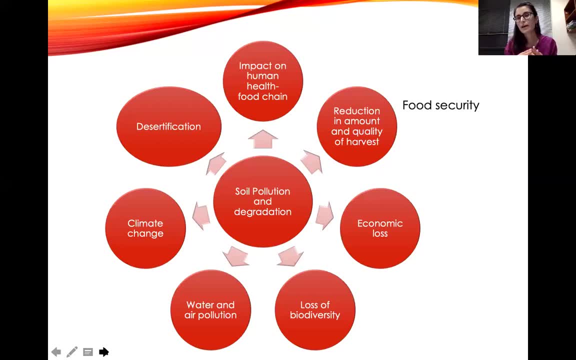 everything else right. so, for example, we said: soil are. soil is a sink for carbon dioxide, and if soil is degraded, then that sink for carbon dioxide would be lost, that ecosystem service would be lost, which means that we will be, by degrading the soil, contributing to climate change even. 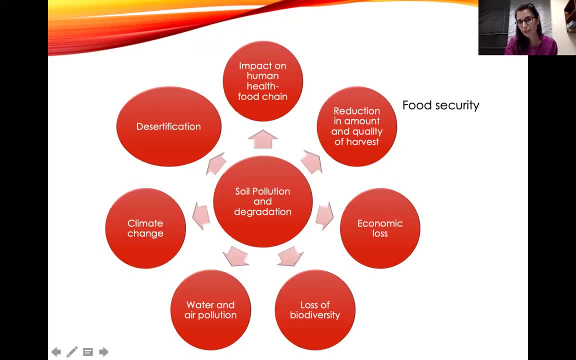 more. and- and you know the points on flooding and everything else- we are very, very correct as well. and then if soil is polluted, even though it cannot move, water and air can move those pollutants around as well, and I think I've put an example of persistent organic pollutant somewhere in the slide, so you 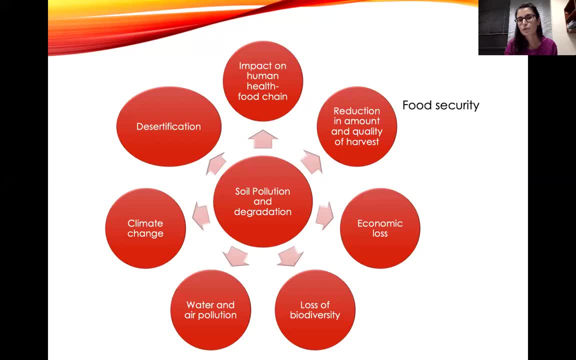 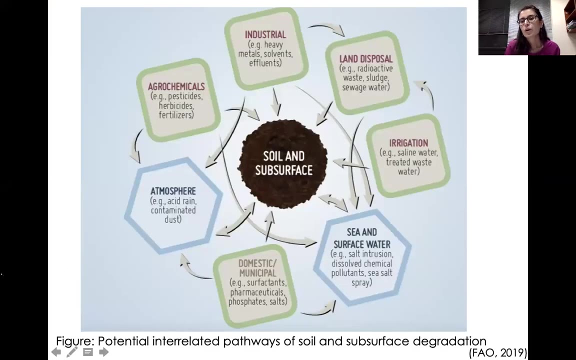 would be able to see it. but you know again that that impact on human life but loss of biodiversity because life is lost and the life that animals depend upon is lost. so everything again is is interlinked. but if we think of how is the soil disturbed or how's the soil degraded and how those degradations, then 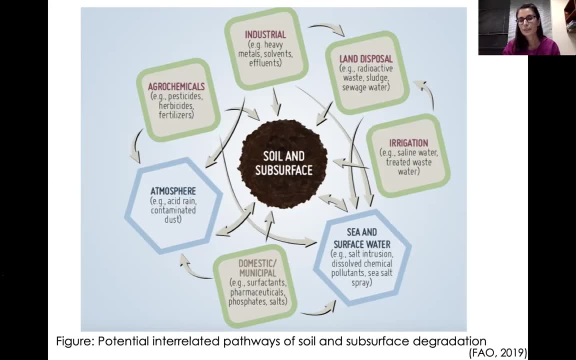 impact other areas. this, this slide and this report in particular. I feel it I had to use a lot of resource from from here, because it was updated and there was there was new information and then I also like the way they integrated things. so, if you're using pesticide, you're using herbicides. if you're using fertilizers, how does? 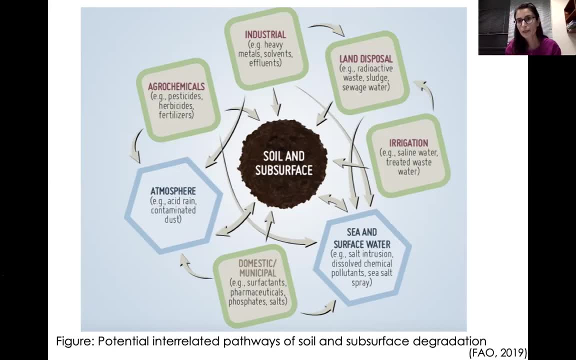 that impact the soil, but how does that also impact the water quality? because then the water takes all the nutrients with them. and you've studied eutrophication and all the other things. you've also studied acid rain and the other things. you've also studied, you know, and then how that rain kind of 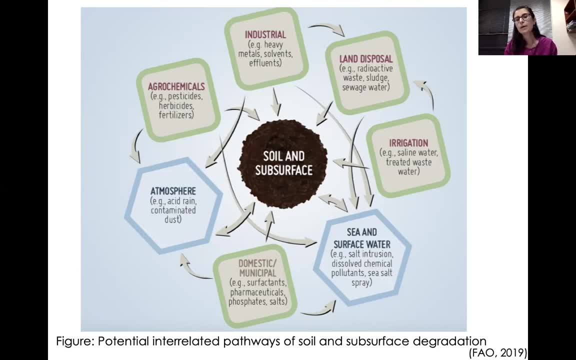 come back, comes back, degrades the soil and then all could contaminate the soil and how that could then become a part of the soil and impact life there as well. any industry, any industrial waste then also has an impact. we've studied all kinds of renewable and non-renewable resources. all of the non-renewable. 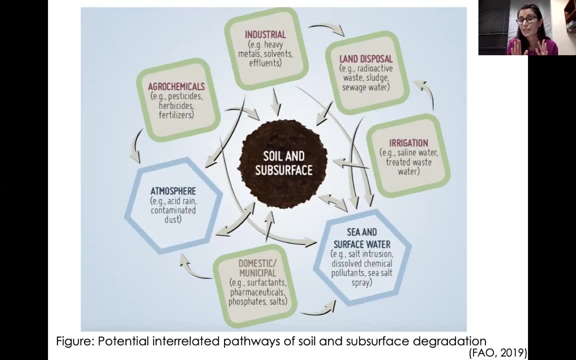 resources are extracted from the ground. that there we studied, you know. we studied packing, we studied disposal of nuclear waste, we've studied disposal of untreated wastewater. all of them impact not just irrigation but also soil quality and the entire food system, and similarly for oceans, I think the if 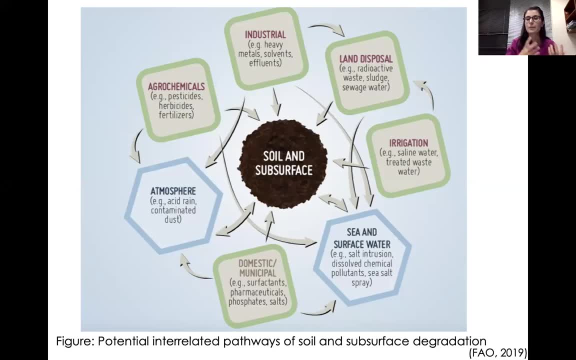 chemicals go to the ocean, or whether salt is coming back to the land. they're both degrading the land and then, in turn, changing lives. so just just for you, to make those extra connections that I hope that all the knowledge that you've taken from this course would. 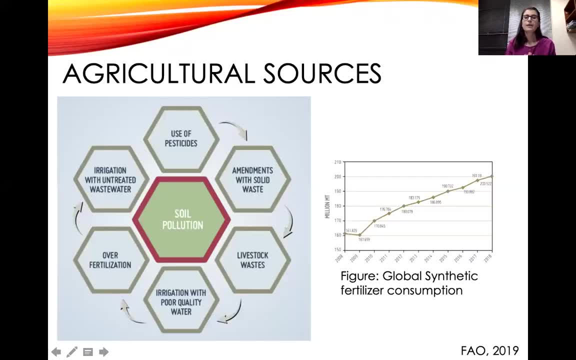 enable you to to make. but if we just focus, for example, I'm not thinking about every other industry, but just the agricultural resources. so from agriculture practices alone, how is the soil polluted? and if anyone wants to speak, they're more than welcome to raise their hand. we put livestock there we use. 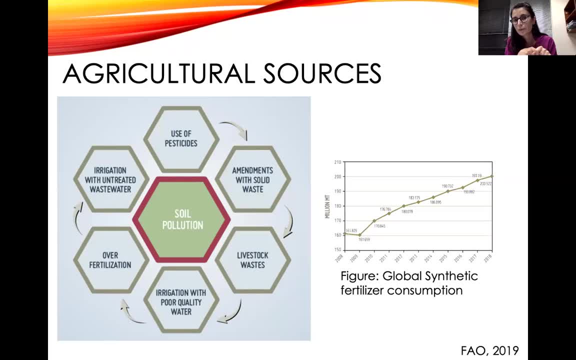 it: fertilizers, we use pesticides, we use pesticides. we use pesticides, we use herbicides. sometimes we just irrigated with wastewater, and that wastewater could come from industries and forms or municipalities, and that then results in degrading this soil quality and and also like any chemicals that are being 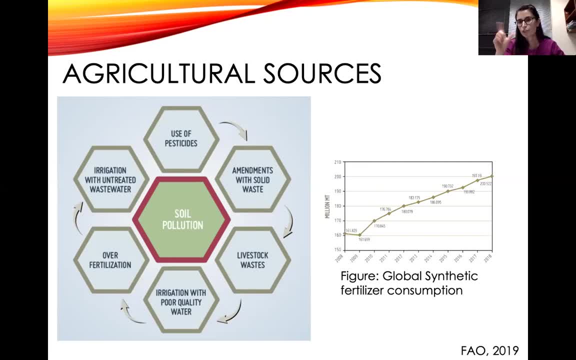 discarded there, and all that pH regime change that we have studied with heavy metals, that how, once you bring in something as something else becomes available to the plant, and then it's an available to the plant, and then it's an available to the plant, and then it's an. 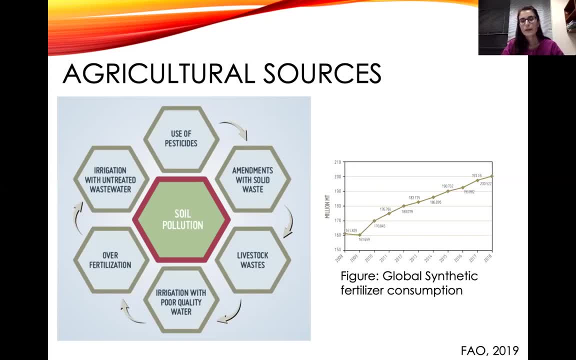 we eat that plant. we could. we could be impacted as well. the slide about um synthetic fertilizer use: i kind of put it there because in this, in the past few presentations, we've talked very much about nature-inspired agriculture or agriculture where the input is very, very low right. 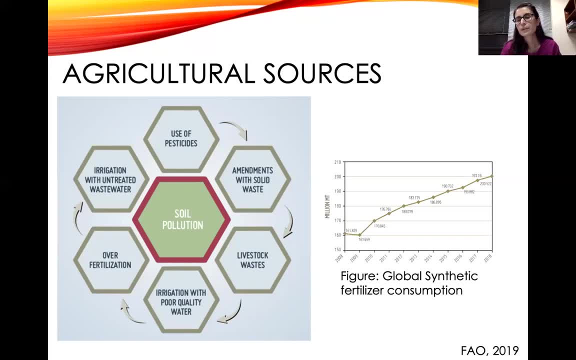 and we were saying that, okay, farmers are now educating themselves and farmers are practicing what we call conservation agriculture, and this practice, the zero till practice and everything else in any ways had started in the 1970s, past the industrial revolution. but you know it hasn't. 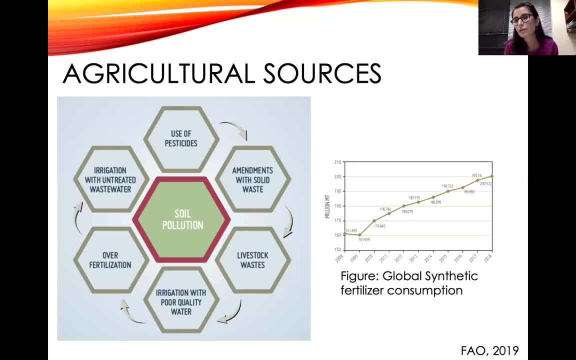 picked up yet. so, even though i taught you a lot of, i taught you all of that, and even though there's a great emphasis on that kind of nature-inspired practices with respect to agriculture, but if you look at that graph, um, it basically tells you that the use of synthetic fertilizers is still increasing, so we're still feeding junk to our soil. 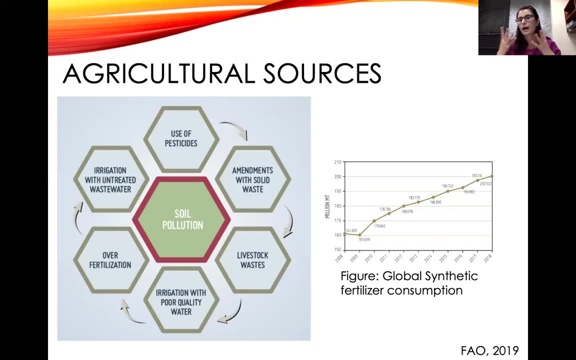 in terms of food, and we're not utilizing the natural biogeochemical cycles or the ability of microbes to fix a lot of things for the plants, um, and we're manipulating it and we're continuously making them dependent on synthetic fertilizers and and the use of synthetic fertilizers, if you start. 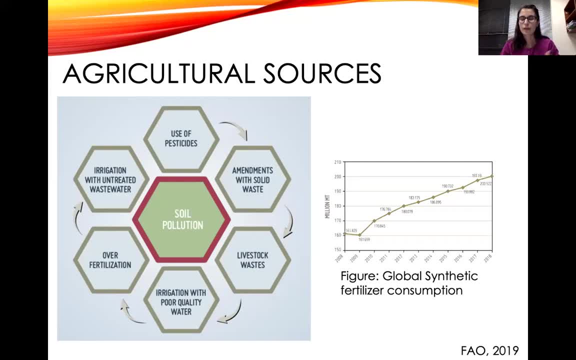 using it on the land. you have to kind of increase the quantity every year- and anyone who's practiced farming would know that- that with each year if you stop organic farming and if you switch to synthetic fertilizers, the quantity is simply going to increase because the soil quality 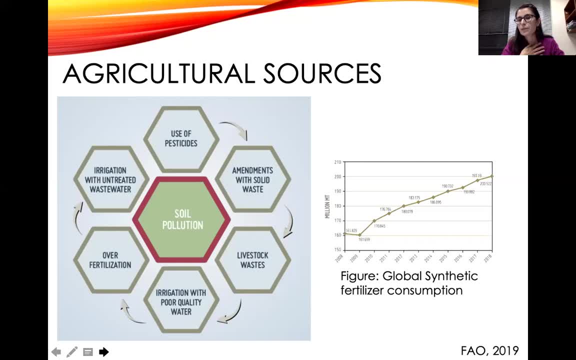 has degraded. so just just a heads up that we are going towards the right direction, but it's difficult, as dr mahmoud had mentioned in his presentation, to fight against these- uh, these corporations that are still selling um practices that are against the environment. now again, i'm going to ask you to speak about the solutions for agriculture and soil pollution. 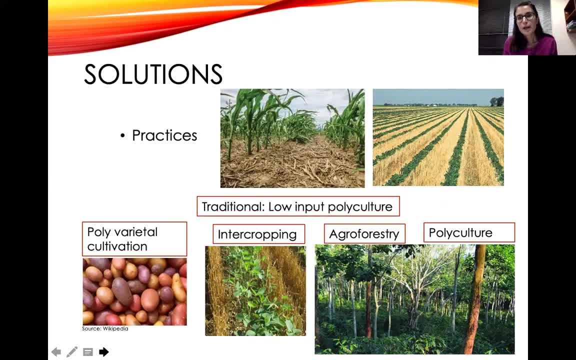 um, and we may have discussed it in the last class, but i just wanted um one of you to to re-emphasize how can we stop degrading our soil, how can we stop soil pollution and what should we do to to keep it safe? hassan. 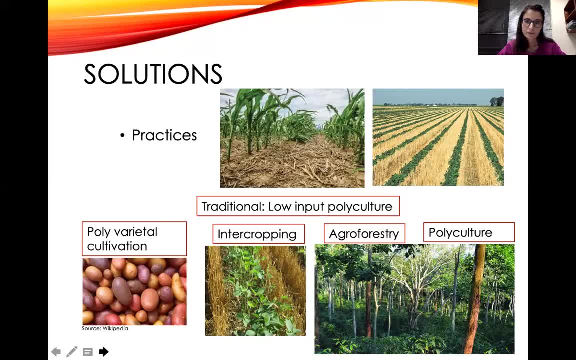 so one of the most important questions that we get is: how can we stop soil pollution? so one of the most important questions that we get is: how can we stop soil pollution? ways mentioned over here is intercropping and if i remember correctly, that was basically planting. 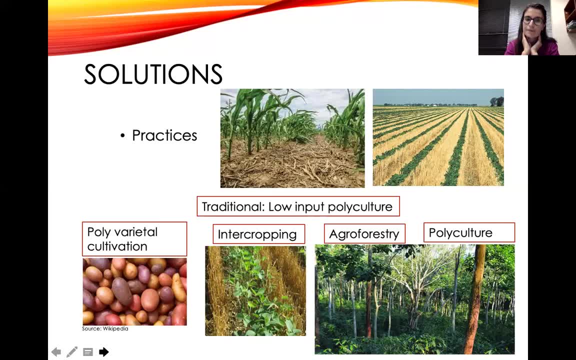 different kinds of crops, each of which have a different function, like one of them can hold on to soil nutrients or the soil component composition better and others have, like, water, regulating capabilities or nitrogen fixing capabilities. so basically, just different types of crops, each having their own function to help the yield. absolutely does. anyone else who hasn't. 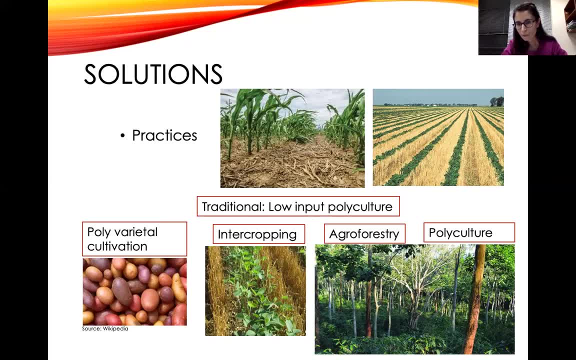 spoken before, wants to speak rapid. um, you know, like how we discussed that one thing where you churned uh after, after uh. there, you used the land, you turn it and you've turned the ground upside down and then you use this movement- i forgot the name- uh, tilling, yeah, or tillage yeah. 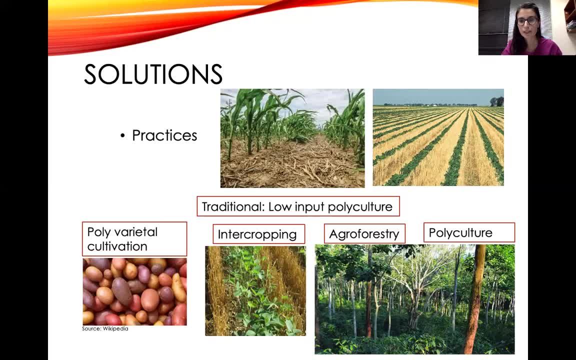 so basically, yes, the ideal practice would be zero tillage. hassan's asked about the units, so basically it's in amounts. so when you use zero tillage means that when you use zero tillage, очень amount of soil is promise. so how do you grow home? how do you- could, you could, grow your plants, and i'm 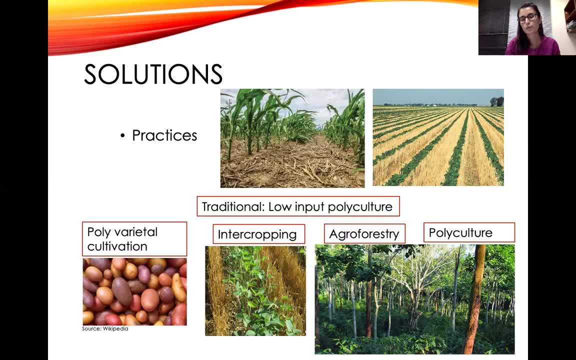 use fertilizers. you're kindly just using it in kilograms, right, so it for global scale. it would probably be metric tons or million metric tons or whatever amount you use, but i think it was million tons for the graph that i'd shown you. um, yeah, and then iman's also saying that we should stop. 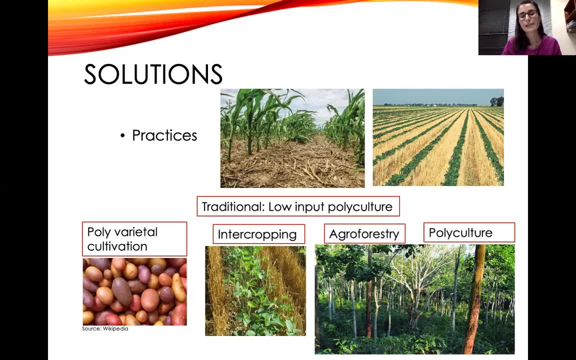 monocropping, absolutely, but i think the key is the um- no tillage or zero tillage- because, as i mentioned in the previous class, that is, that's the carbon sequestration that we all want. that's the kind of service that we want for the soil to have for more and more carbon to be captured. 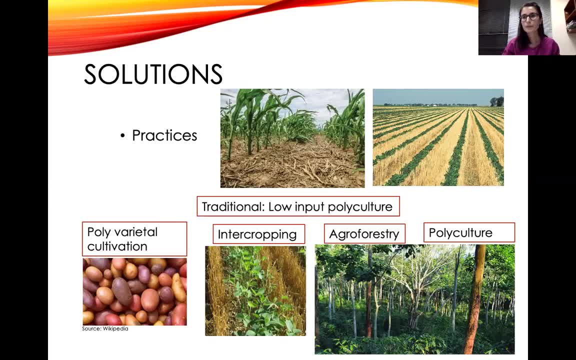 via the plant into the soil and when that happens- so, for example, even if it's organic in the organic form and it stays there in the soil- degrades itself. um, it's there, it's kind of a carbon sink. but when we make it there, when we topple it up, when we till. 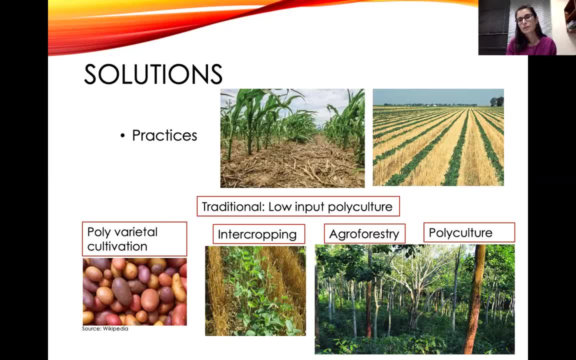 we disturb it and we disturb the life there and that's why it's a practice that's discouraged. but the farmer who had, who we had met um the organization called pedawar who we work with at the center, they're all encouraging farmers to practice this, which is zero till. 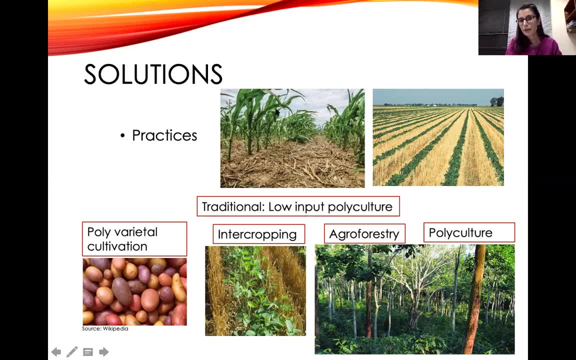 um, and also what i was saying about not burning rice, um, before you crop the next. it's like you use those, you've created that kind of machinery that helps you, uh, crop without kind of disturbing the soil too much, um, so minimum till or zero till, without changing the landscape too. 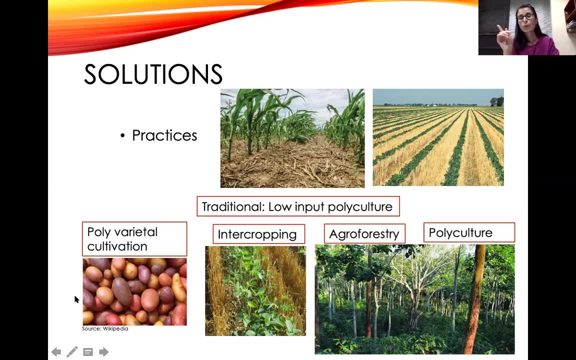 much and whatever you do, take inspiration from nature. think about how this could happen in the forest, think about how this could happen in a natural setting, and then just do it there without too much disturbance. and why is soil important? because a lot of soil chemicals can reach down to. 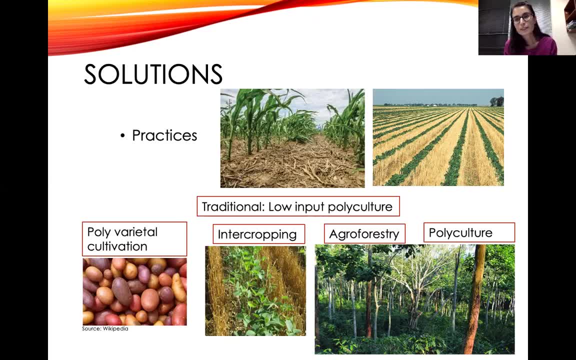 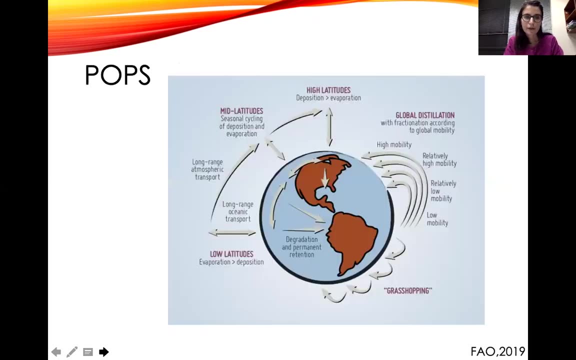 is polluted, and if there are chemicals that can leach heavy metals into groundwater, then soil pollution and soil remediation, or treating soil, also means groundwater pollution and groundwater remediation. so just just think of that as well. don't think that we're only talking soil right now. 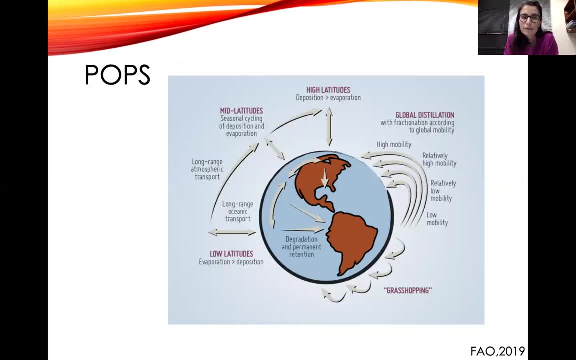 and and people have been interested in, interested in, in finding out. you know what's going on with the, with certain pollutants, with persistent organic pollutants. i i often told you that they are persistent. they they stay in the, these kinds of dioxins that we've used. 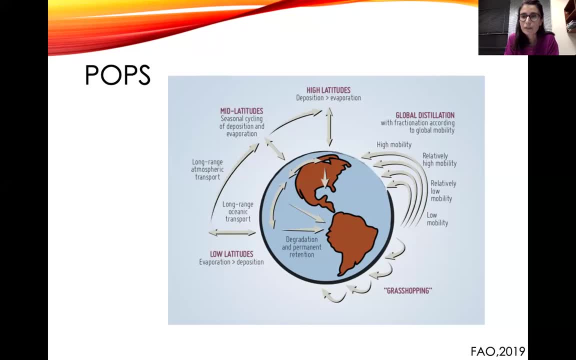 in agriculture a lot. they stay in the environment for a very, very long time and most of you- whether we talked about microplastics or ozone or anything else- wanted to know how it was able to travel so much, and- and i had taught you the weather patterns at some point- 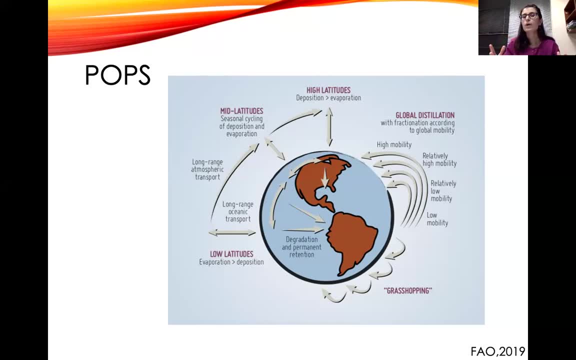 because i wanted you to be able to make that connection about how certain weather patterns or wind and all of those could could impact it, but also when it comes to control. so, for example, if the wind is blowing it, then you know, you can think of what kind of agricultural practice would. 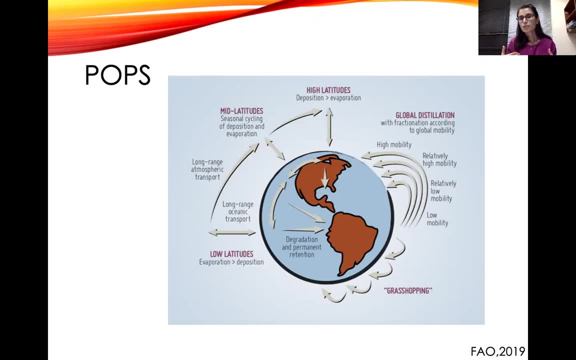 stop it. so i would say something like agroforestry, where you're putting a boundary line of trees for for a certain land, could, could probably stop it. so just think about those. but also it won't be possible to contain everything. there are, as, as han and paul will know, there are many, many, many uh, chemical pollutants that 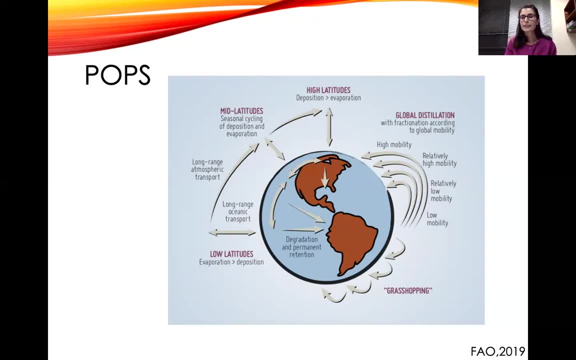 are volatile in nature, uh, and that means that they they can't stay on the ground, so they just evaporate, and then they go to the atmosphere, and then it's difficult to contain them, and and then the approaches that you take, for example, in terms of life, whether it's bacteria or or other kind of 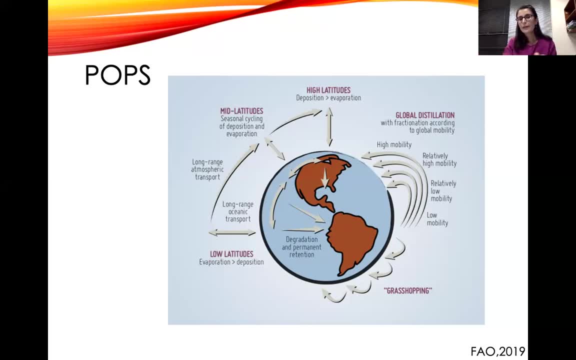 is to hold it there, is to stop it from from moving. but, um, i i just wanted to share this with you for you to look at. you know what? how could it stop? for example, if the deposition rate is increased, then the evaporation length, then how can you, how could you stop it at a certain point? and 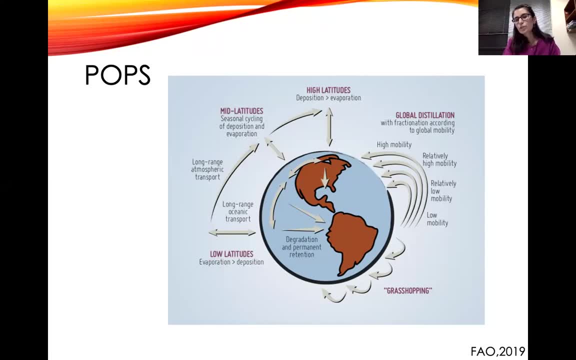 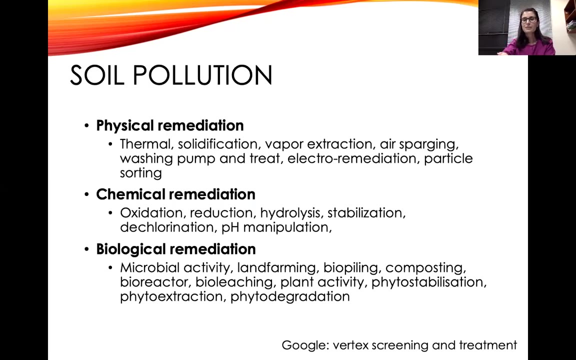 stop it from spreading further. and that's, you know, not not just an information for for scientists, but also for policy makers as well. yes, and this one so last time, because i introduced different terms to you and i was explaining it to you in great detail. this time i've just put it in different compartments and i want 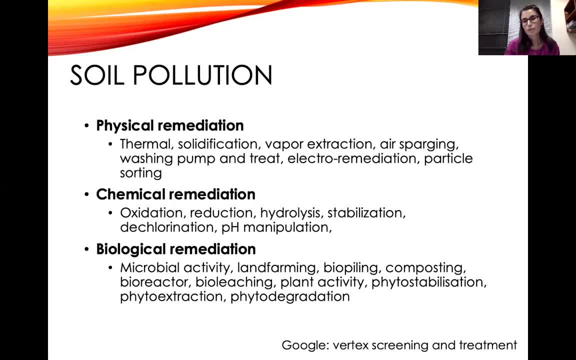 to be explaining everything because we'll be jumping to the case studies and uh and and. but there are different kinds of uh, ways in which you can treat soil pollution and um, and they can be physical. so, for example, you just use a simple thing to to contain it um, or an electromagnetic plate to just be there and and take that hydrocarbon out, or it. 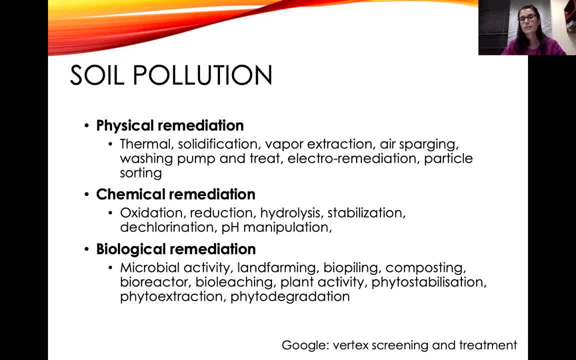 could be chemical, where you're using certain kind of chemicals or certain kind of conditions for reactions to take place chemically, or you're manipulating the ph, as as we had studied before. or it could be biological, where you're either putting a plant or it could be an extensive 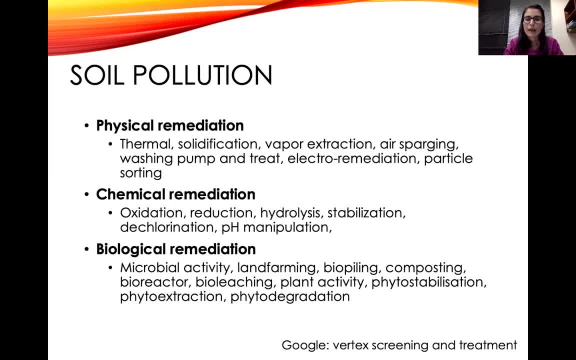 bioremediation technique, for example, land forming or biopiling. they're all techniques where you literally take that site as a bioremediation site. and what? do you have a question? um? yeah, i, i'm just wondering, i'm a little confused, um about something. um, it might be fairly simple, but 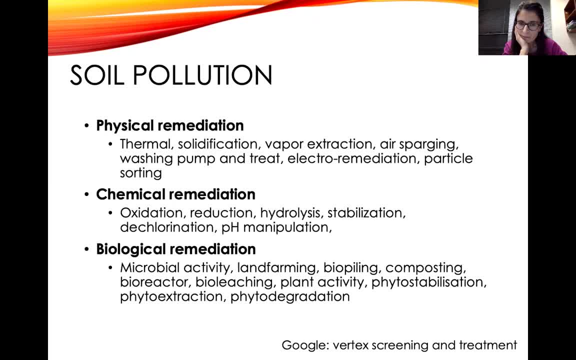 how do we distinguish um soil degradation from land degradation? so it's like it's it's the same thing. yeah, because um, okay, all right, but why would you think? why would you think they're different? because maybe you have, i don't know- no um with land degradation. i've always referred um like. 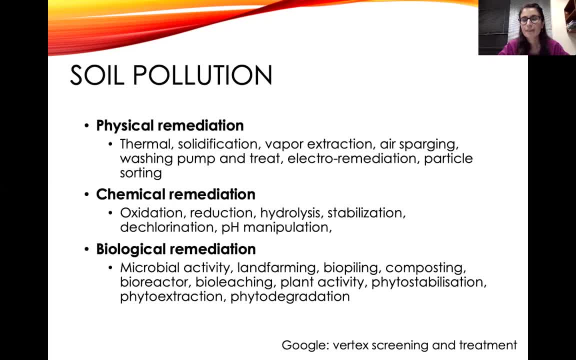 i've always linked deforestation for some reason, like that's the first thing that comes to my mind when i think of it. so it's me, since we haven't really like i don't know. so i was thinking maybe it's sort of different from that, um, in some ways or the other, because this is more related to what? 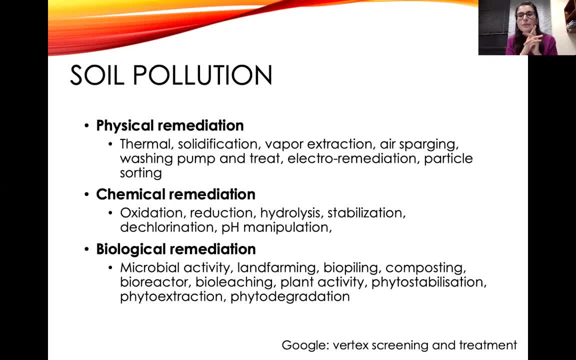 is agriculture. yeah, um, yeah, yeah, that's what. what we can do is um. just for your understanding, let's put soil as um, as a medium where food is grown, and let's refer to everything else's land, right, so that way it would be easy for you to think um, because we are manipulating this. 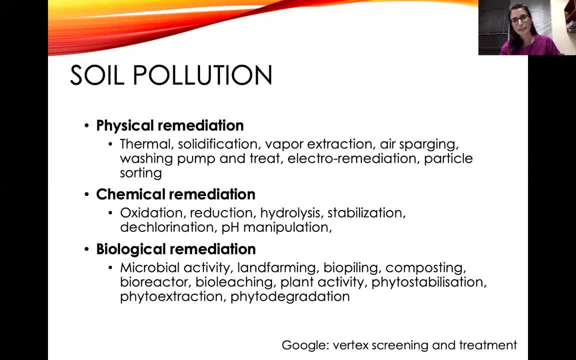 particular resource for the reason that we're growing crops for ourselves, we are just referring to this as soil and everything else everywhere else in the world we just refer to as um land. okay, so yeah, like in a way, if you want to, you can, you can distinguish them, but i would like to keep. 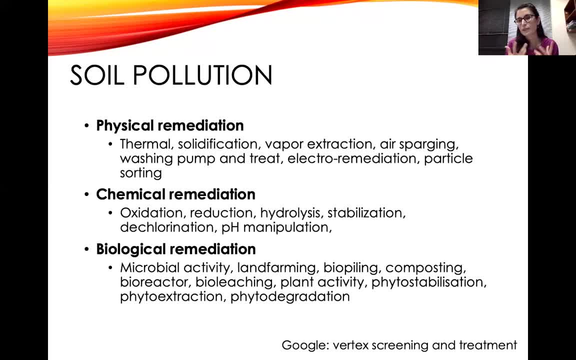 the entire lithosphere, um, as as one thing, as one sphere of the environment, but, but i think you're also right, depending on what you want to do, you could compartmentalize them into different areas as well. okay, okay, thank you, you're welcome. so these, these terms, do you want me to go through them one by one, or are you okay if we just jump? 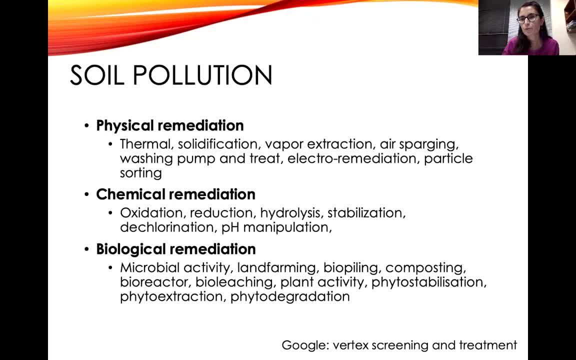 to the slides, or would you like to add on to to one of the points because you've read something somewhere and it excites you? okay, maybe i'll just take one. so, for example, um, air sparging is when you create a vacuum, take pressured air into the soil or into the groundwater and make the hydrocarbons. 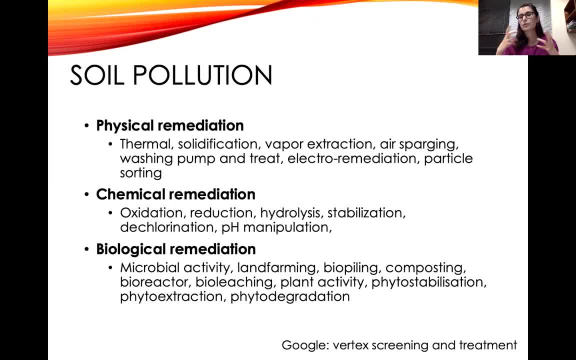 to escape. so they are. if the hydrocarbons or if the oil or let's say petroleum or diesel, has become leached into the, or if there's been a crack and it has gone into the groundwater or into the soil, then you kind of create that way that vacuum and then sparge it with air and with pressure, take it. 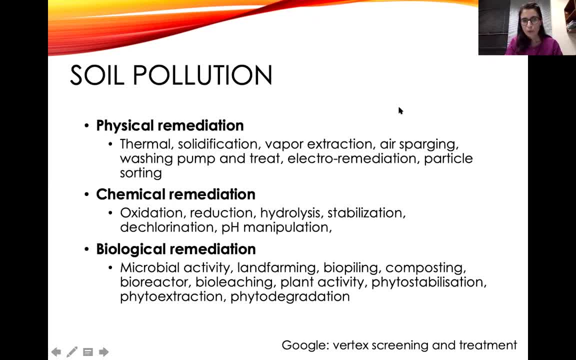 out, excuse me, from the ground right. so that's that's one: washing and pumping, pumping and treating simply. is that because it's difficult to treat ground water under the soil and therefore the soil around the groundwater, you would just extract it, pump it out, treat it on the surface and then maybe use it or or put. 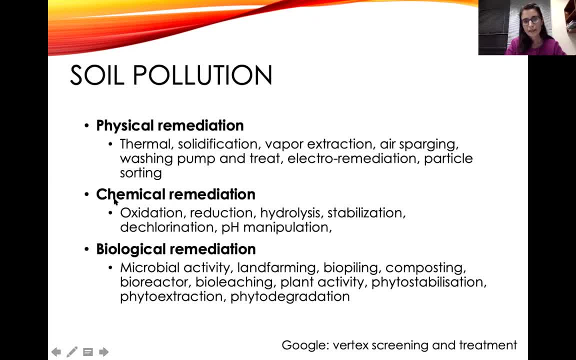 it back into the soil and hydrolysis is basically simply degrading something in the presence of water. so you- you use water, make something interact. so maybe you can use complex hydrocarbons, bigger hydrocarbons which have longer chains. you interact them with water and then they degrade into smaller hydrocarbons. 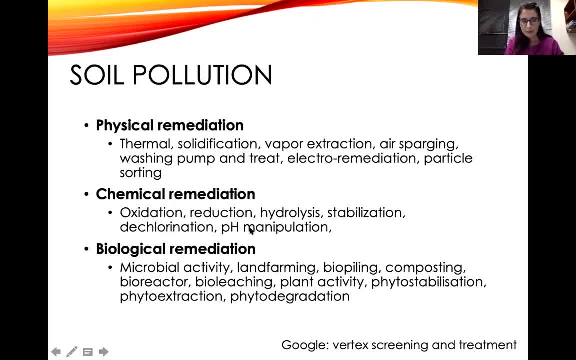 that are easy to degrade. ph manipulation. you sort of have an idea um. land forming is when you, for example, take a land, it's completely contaminated site. now what you do is you create a lining. so let's say you use a very thick plastic lining where you're making sure that the 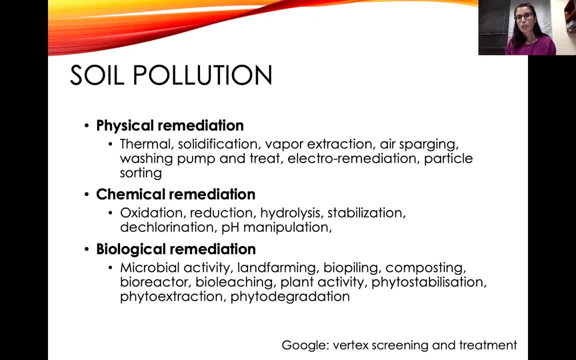 contaminated soil that you put on doesn't leach anything into the soil further and you are treating that as a as a land where you are doing a lot of activities, where you're farming or treating or exposing it to oxygen and light to treat that contaminated soil and turn it into better clean. 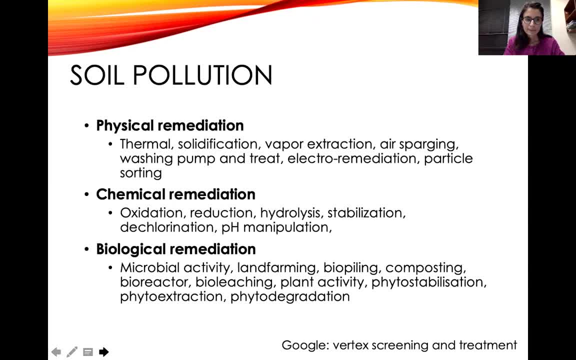 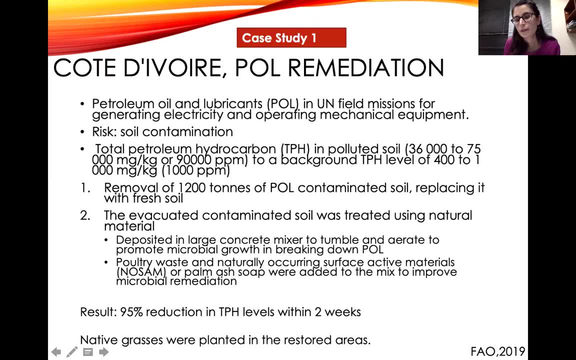 soil and what else. some of them will will study in the slides further, so i'll just leave it. does anybody have a question? up until this point, i can see that as hands expanding the boundaries of science and technology, which is good. yeah, organic fertilizers, thank you. any questions? no, okay, so now we'll look. 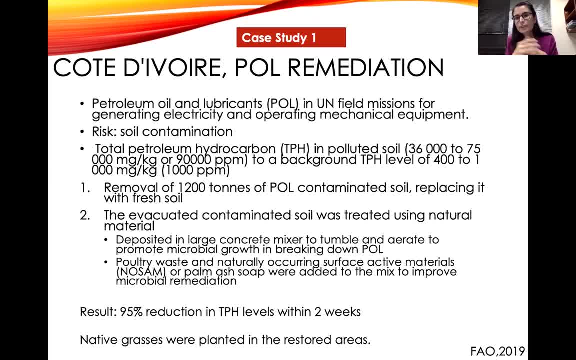 at three case studies, and all of these case studies of first examples of soil being contaminated by a certain contaminant, mostly hydrocarbons, and then how they treated that particular soil. so, um, let's take this chat box away. so this code deva, if i'm pronouncing it right, is uh? 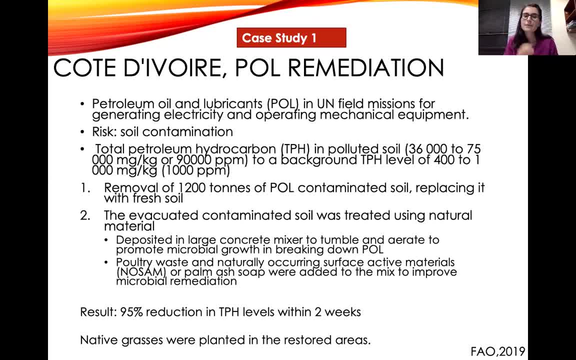 had, it's in africa. somewhere in africa they had petroleum oil and lubricant problem and the reason- major reason- for that was, of course, it was the un was always there. they have a lot of beef stability and therefore un peace mission goes there and they're working there all the time. 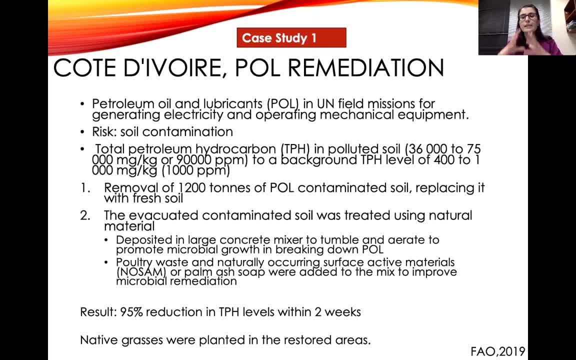 which means that they take a lot of mechanical stuff with them or they need those temporary residences where electricity is required and mechanical operations are required. but when you use such operations, that means that a lot of oil and lubricants are also transported, because you're generating electricity or any other thing that you need for a cam and that then results. 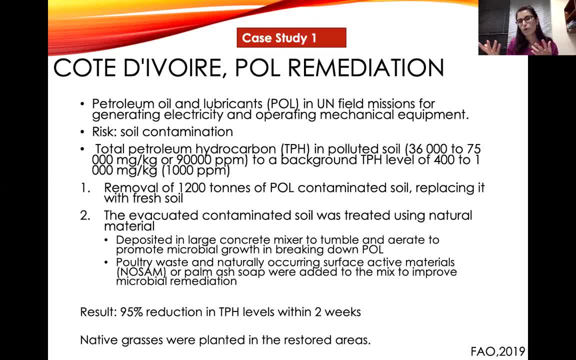 in contamination of the soil. so that's one of the things that we're going to look at in the next slide. so let's talk about the pollution of the soil, because oftentimes, when you're leaving, you're leaving all things behind, or sometimes, when you're operating it, you're not really operating it. 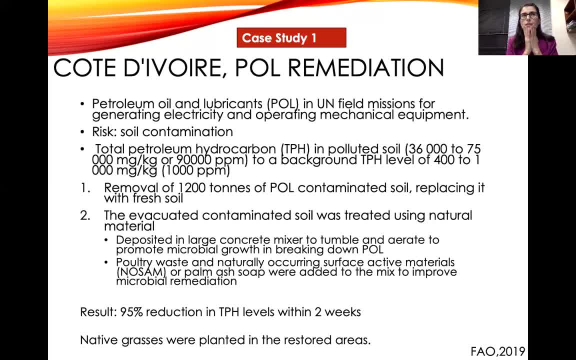 carefully and then that puts a risk of polluting the soil. so what happened was that this particular area or this particular region had a lot of petroleum oil and lubricant in the soil. so let's say, if we use an easy, relatively easy medium, they had ninety thousand ppm of ball and then 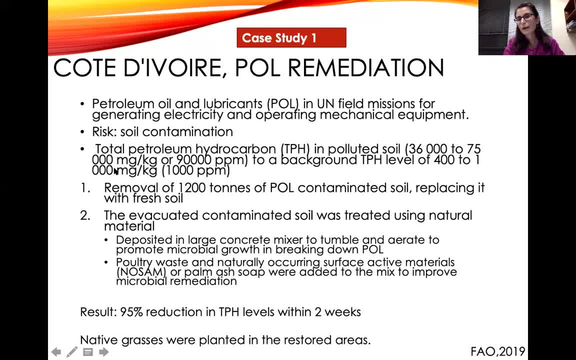 by. after treating it they brought it down to thousand ppm. but how was that possible? like ninety thousand ppm is this huge amount? it's like ninety thousand milligrams per liter, basically, of these uh, petroleum hydrocarbon in the soil and they had to bring it down to a very low lower. 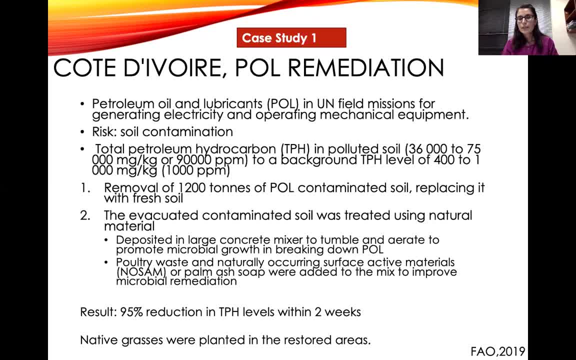 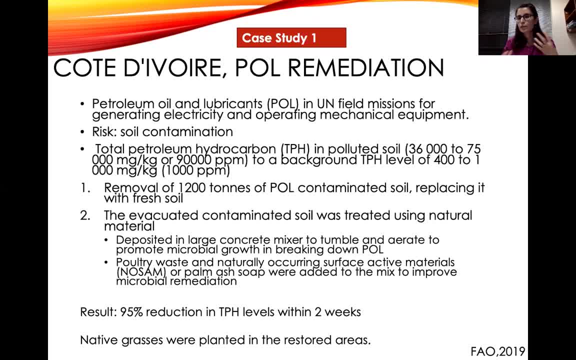 there. then again, we have that problem of the, during the treatment process, for things, for chemicals to leach down, which we do not want, because we don't want the surrounding soil to be contaminated as well. so the first thing, what that they did, was that they removed 1200 tons. 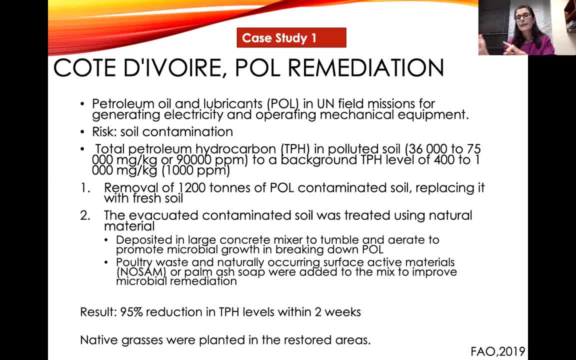 of um- all contaminated soil- and then they replaced that particular soil with a fresh soil, took this soil, and then they used it in a different way, and then they used it in a different way, and then they used it in a different way, and then they used these concrete mixers because um in biology. 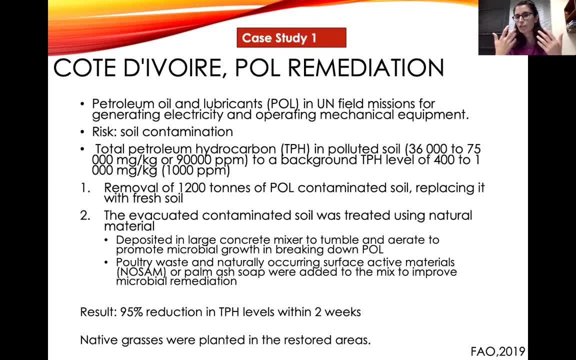 um, i think summer and others who are from biology would know- you're always using oxygen and mixing to increase the degradation activity. um, and i'm sure this is true for chemistry as well- but so what they did was that they used these concrete mixers because they could continuously mix this. 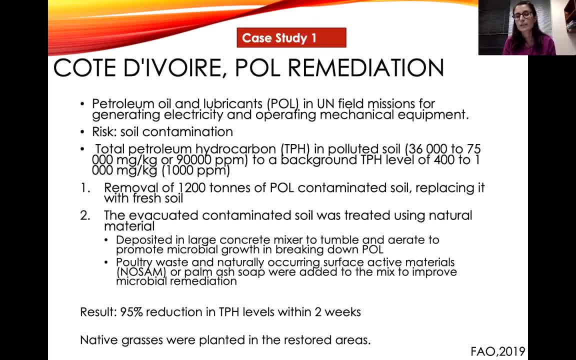 contaminated soil and the activity inside, whether it's using microorganisms or other manure, could increase. so the top soil was removed, put in a concrete mixture and then the next thing that that you do is you give food to whatever's degrading it. so let's say, if the chemical is able to degrade in. 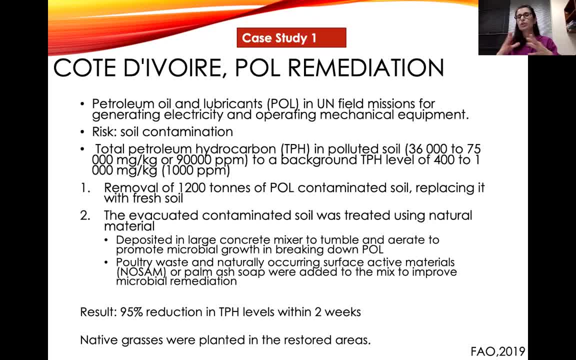 the oxidizing, the presence of oxygen- you would just expose it to oil- but in this particular case, microorganisms. so to increase the concentration of microorganisms, you need to give them good food, right. so phosphorus and nitrogen and carbon and all of that. so what they then used, was they used? 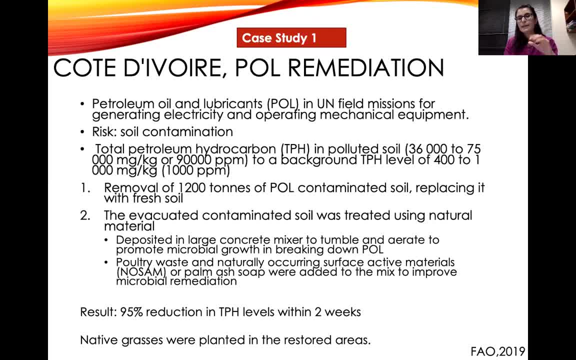 natural material, which is the poultry waste, and surface active materials. natural surface active materials. so poultry waste was used as a growth medium or as food for microorganisms that were present in that concrete mixture, and by mixing it they allowed for them to be just, to remain active and to be able to degrade the contaminated soil and within two weeks they 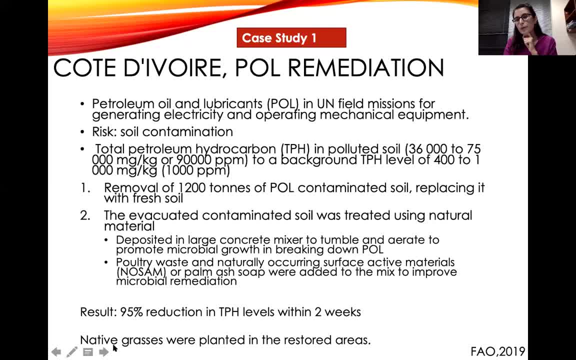 were able to reduce the tph, or the total petroleum hydrocarbon level, down to 95 and after that, like once you know that the soil is relatively better, then you start growing crops on it, and the best way for soil remediation, or soil reclamation generally, is to use crops that are local or 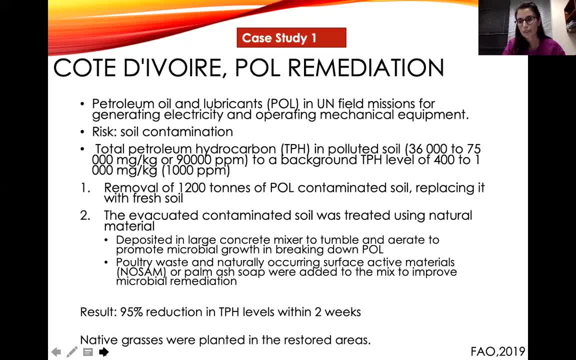 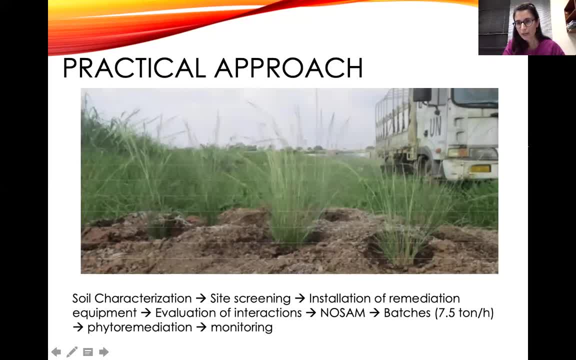 natural, because then you know, it comes back to its natural state or its natural habitat. what is that i'm saying, ashan, you can, you can just say it out loud. so, ma'am, basically, i want to say that, uh, it depends upon the leach, at least. principle. 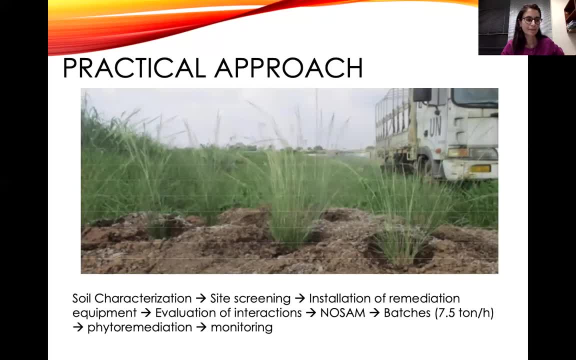 which is basically, uh, talks about dynamic, achieving the dynamic equilibrium, like by disturbing the change in the condition. the position of behavior moves depending upon the initial concentration of the reactants in the products. right, so how? how would this so? if you think of this particular environment, how would it happen here? 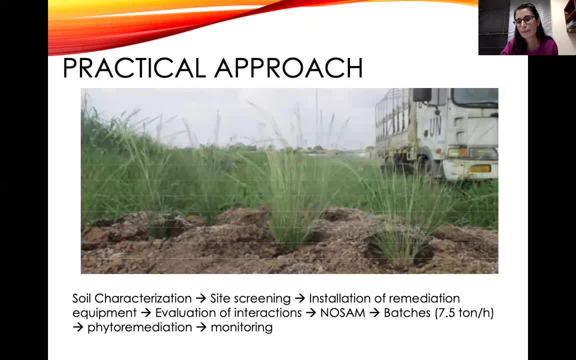 if you could apply the same principle here. so, uh, there's the main concern right now for me, like i was, like it depends upon the condition of the soil, uh, and the contamination, contamination that it already has. uh, for some contamination, i believe it will be. uh, a direction will definitely move forward, but it's not necessary. i just want to say this. 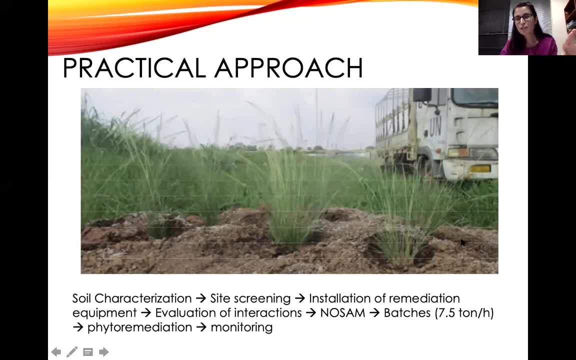 yeah, so, yeah. so even reduction is a treatment process in soil remediation asan. so it's not necessary that only oxidation is used to remediate the soil. reduction can also be used to remediate the soil. so sometimes you know, as we read um in the last last lecture, that sometimes when you are 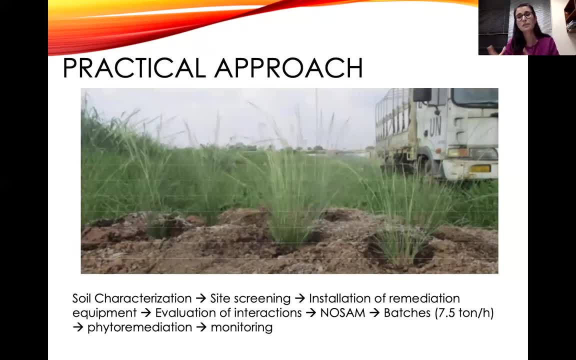 reacting these different chemicals, they can become something very difficult as well, so more difficult than what your parent compound was or the parent pollutant was. so of course, you have to be very, very knowledgeable to know, to know that as well. like, whatever you're doing, you have to do it. 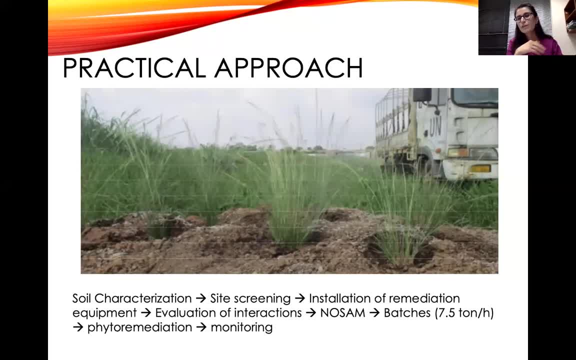 consciously, and you have to be educated enough to do that. generally, i um because for microorganisms, you require air, you require aeration. it's a general practice that you would expect for for the environment to be- you know more um oxygen friendly, but for certain reactions to take place, 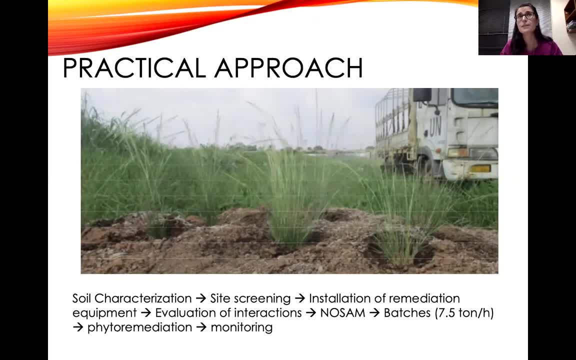 so, for example, if, if it's being reduced or if it's being, if it is being oxidized. so, for example, if fe2 plus is becoming fe plus three, so ferrous to ferric, right, if i'm not wrong- then you know. if that's good for the environment or bad for the environment is a decision that someone sits and 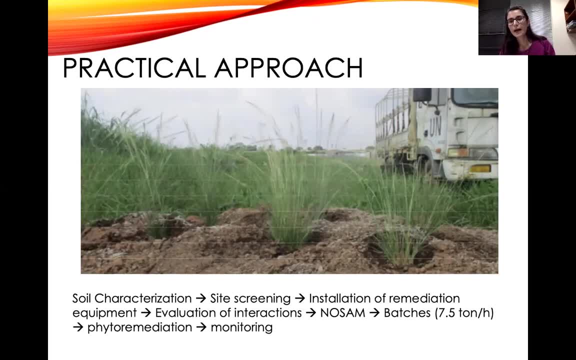 and makes at a particular point. so we're oxidizing iron from one form to the other to achieve what? we're oxidizing uh, mercury from one form to the other to do what? so, for example, we could oxidize mercury and make it, or reduce mercury and make it, you know, zero in in its zero valence state. we 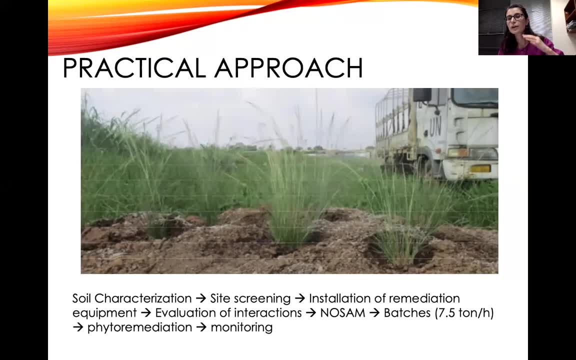 could just release it to the air, but if the objective is to not let it escape into the air, then we probably would need to oxidize it instead. so i think those kind of decisions need to be made, and you're absolutely right, there's no set principle that this is where i 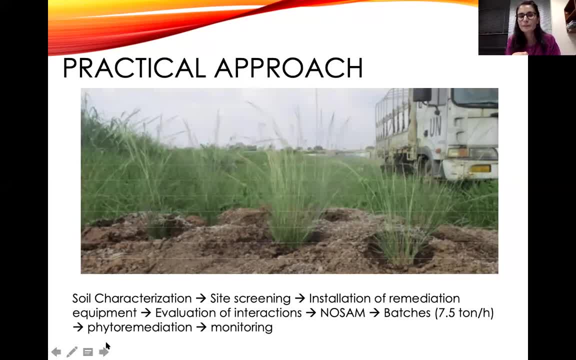 think and again, even for those equations, um to happen, the environmental conditions need to be right: the, the ph, the temperature, the, the quantity, the equilibrium and whatever you're talking about. they all need to be there. so, yeah, thanks for putting in some chemistry for your customers. okay, so now that soil is contaminated, the approach that they took was that they took the soil. 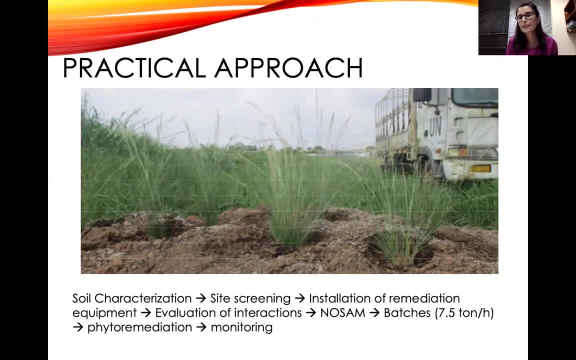 they characterized it, they screened the site, they looked at it, they used a certain kind of equipment to remediate it. they looked at the interactions. they used certain kind of food for the microorganism and the protozoans, or whatever that we're using the, the nutrients, to degrade. 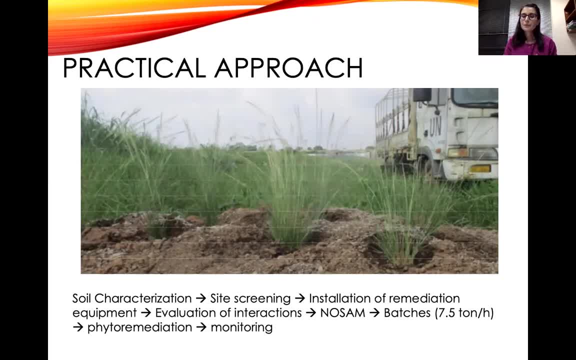 the hydrocarbons or the petroleum in the soil and then they did it in batches. so of course the concrete mixer could only take certain amounts that they did it in batches and then they used the microorganisms that was acclimatized to in in the batches to follow and then recovered the soil. 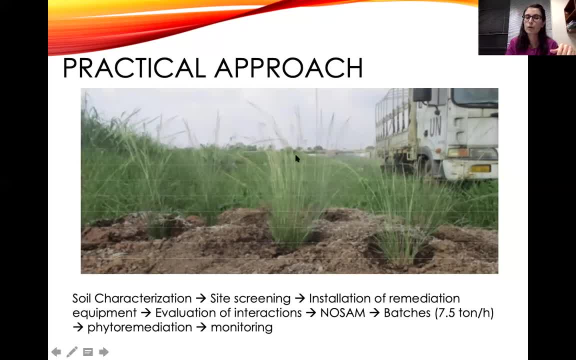 and after that they practiced vital remediation, where they put the local grass onto the soil and then they had to monitor it for several, several years. so when we pollute the environment, when we contaminate the soil, when we do something, we think that it's very. 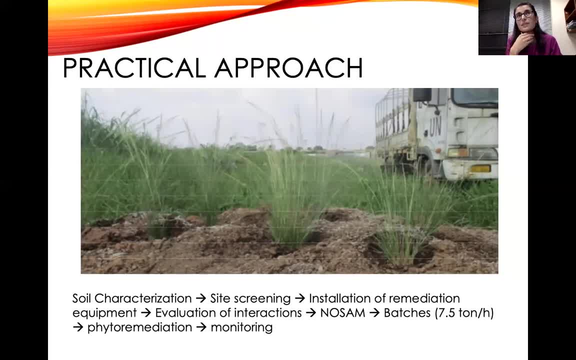 you know, we think that someone's going to take care of it. sometimes these practices take 10, 20, 30 years because you have to continuously monitor it to see that everything has been remediated. Just because plant is growing there doesn't mean that the soil is healthy. 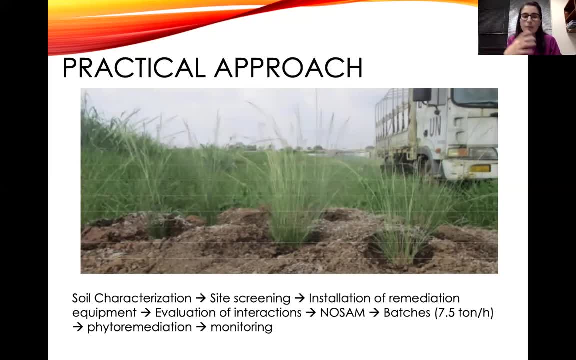 because some plants have the ability to grow in toxic conditions and some plants have the ability to grow in very, very toxic conditions. So that's why there needs to be a monitoring, and that would be the practical approach to remediating the soil, not just bringing populations here. 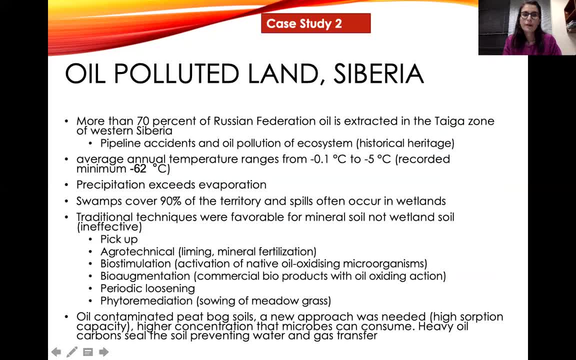 and telling it's now safe to live here. And the second case study is of an oil polluted site in Siberia And the reason why I chose this again was, for example, to tell you to make that kind of environmental connection about. 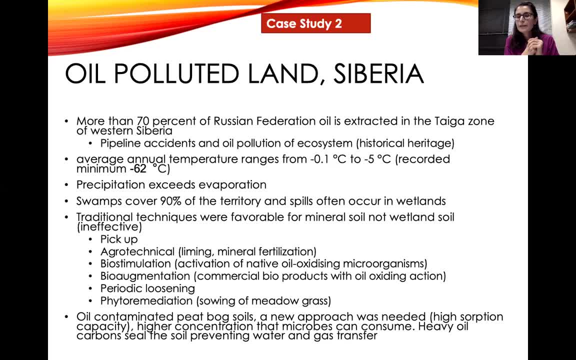 okay, a particular treatment mechanism has been found out. a chemist or a biologist has, in the lab, found out that you can use this equipment and you can use these plants, and you can use these bacterias and you can grow them and they would be able to take care of the soil. 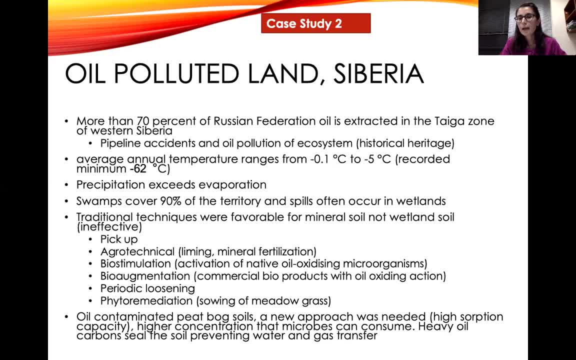 But suddenly there is a land polluted site in Siberia and it's very, very cold, Or even, let's say, to many regions in the north of Pakistan, For example, the biogas plant that we had seen in one of the villages in Hunza. 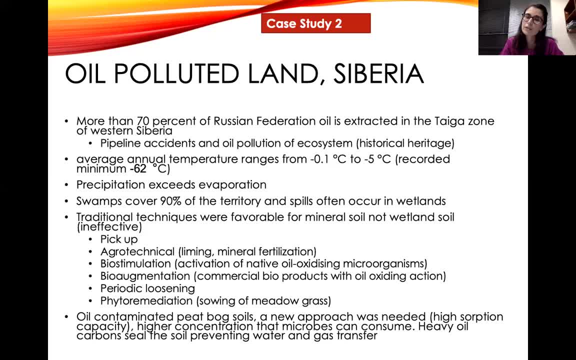 it didn't operate in the winter because it's very cold there in winter. So if you are designing something thinking this could happen around the year in Hunza or Savat or anywhere else, that's not going to be the case, So those conditions very much depend. 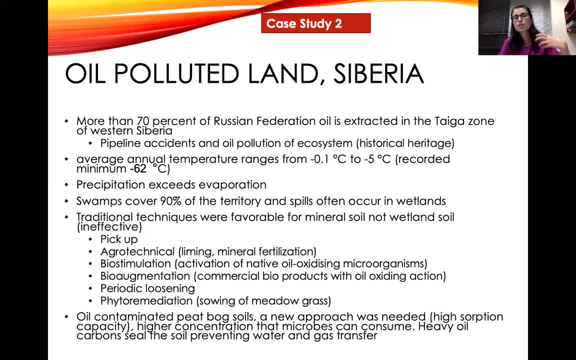 on the environmental conditions and how you achieved remediation of land in the previous case study does not necessarily apply to a similar kind of land in Siberia, because the environmental conditions in both areas are very, very different. That's perhaps a warmer region. This is a relatively warmer region. 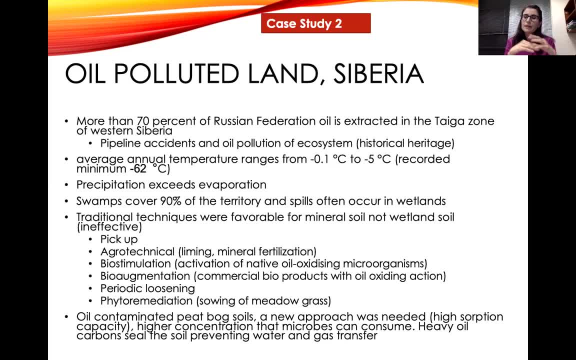 This is a relatively colder region. So now what happens is that this particular region, the tiger zone in Siberia, is where Russians extract the oils from, And which means that, because all the oil is going from here, a lot of pipes are originating from here as well. 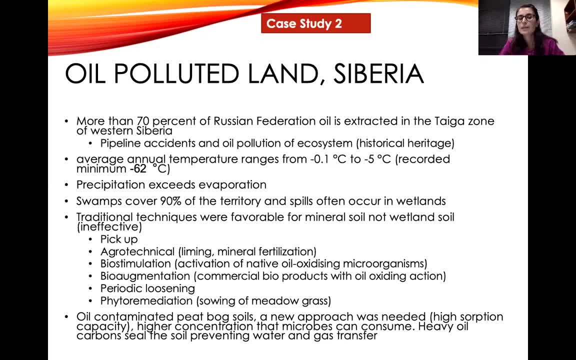 And I taught you laws and policies and limits, for the same reason that, when those laws did not exist, people did not care. when there were accidents, People did not care when the pipes exploded somewhere or if there were leaks somewhere, If the leak was so tiny, so minute. 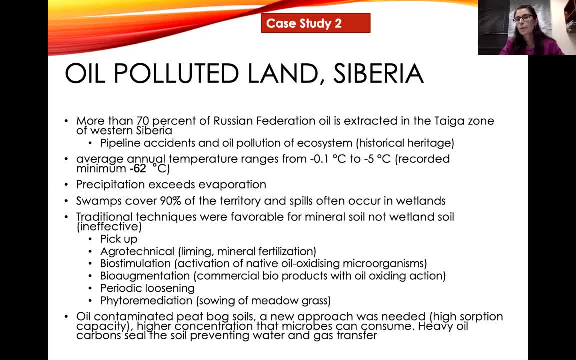 they wouldn't care much, depending on how big their resources were. So that's what happened, And I think Fatih would like this term. historical heritage was something that I learned, For example, if I'm a new oil digging company or a company that's there to explore more oil sites. 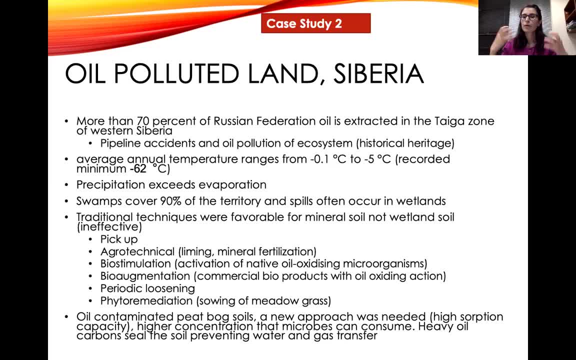 If a company before me that was operated there has used or extracted something and then wasted or discarded some oil or the initial thick mixture, if they've discarded it on the soil, if they leave it there and I'm the next person coming in and using the same site. 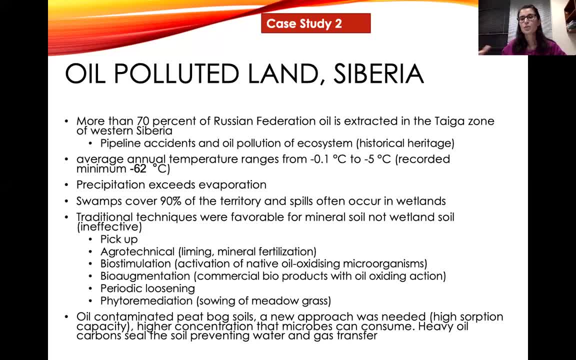 now the soil was already contaminated by somebody else. So the kind of pollution that exists there in this particular language is called historical heritage. because they've left that heritage for me, for someone who's just come in in a relatively stricter conditions, in a relatively tight actions on consequences. 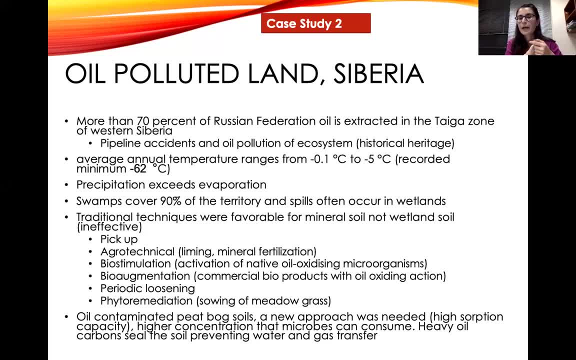 For example, I might have to pay for polluting. I might need to remediate the soil before I leave the site. They did not have to, but because they're passing it on to me, it's a historical heritage of pollution, So a lot of ecosystems were polluted. 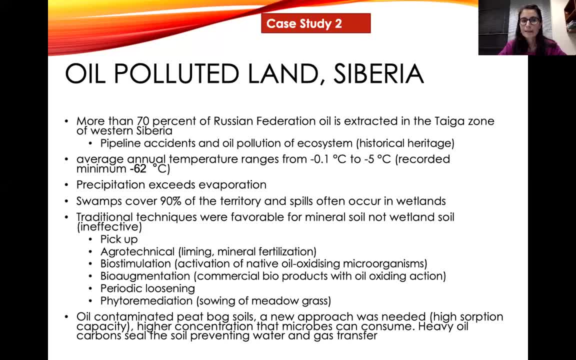 There was no action taken. and then, when it started degrading life- because this region has a lot of swamps and wetlands, And when it started degrading life, when the number of species just started disappearing, they got concerned. but then there was an issue. 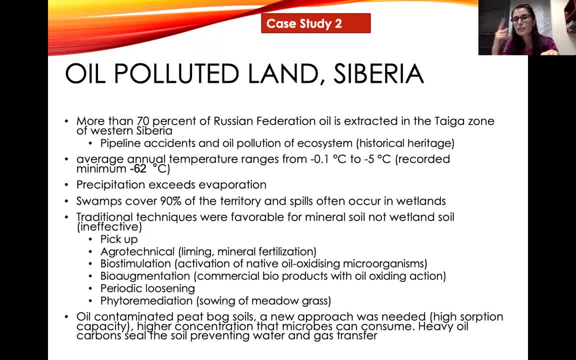 Like I said, the traditional pick up the soil, use that technical machine to treat it, because microorganisms need a certain temperature. to ensure that temperature, they might've needed more power, power supply or something else, And that would have made it expensive, or to use certain chemicals. 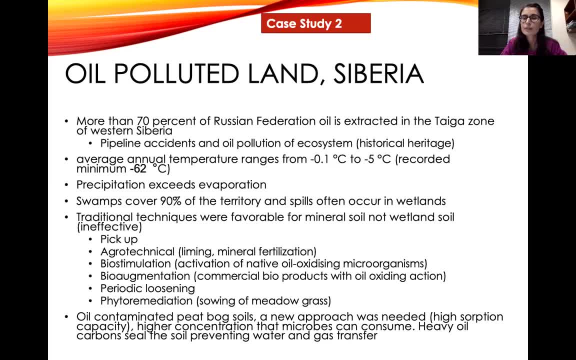 It might have become an expensive process, because I'm thinking this probably is a remote area. So what they did then was they used the natural environment. So, for example, the natural conditions were used to treat the soil. And the second reason why it had become so difficult was 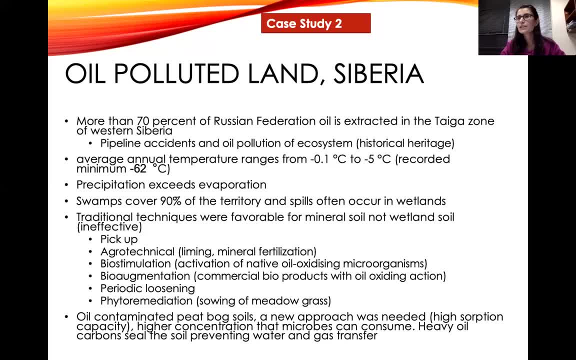 the second reason why it had become so difficult was the ability of those wetlands, So those soils that are loose. they contain organic content, They quickly absorb this oil, They quickly absorb these pollution And it was difficult to extract it then. 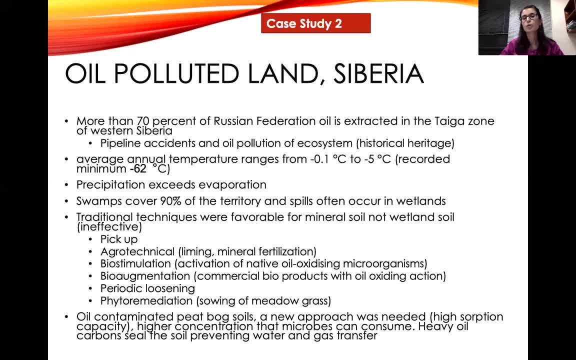 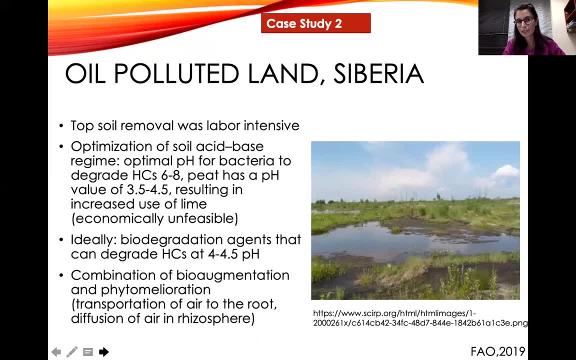 because, as you know, to extract it you probably need another chemical or you would probably need more water to kind of pressure it, And then everything just makes it more difficult to remediate the soil. So taking soil out was labor intensive. That was a difficulty. 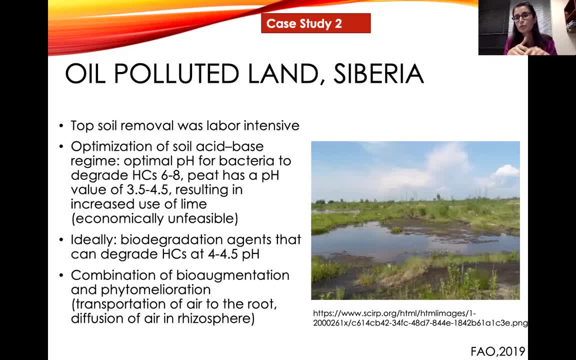 Using all the other conditions that had previously been used in all the other regions was difficult. It was economically not efficient. The soil or the kind of conditions that were there, which was peat. it had a pH which was more acidic, And we know that in acidic pH. 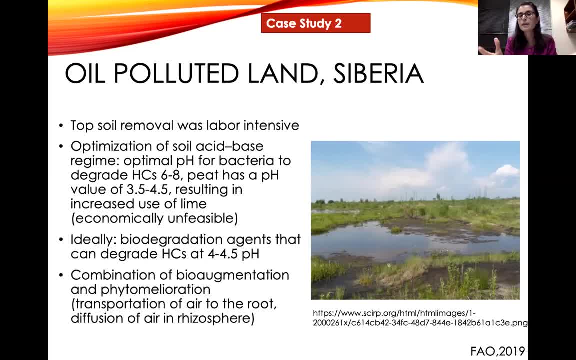 heavy metals become bioavailable, And sometimes heavy metals are toxic to microorganisms. So that also was another problem. But what they did was they used the. they used the acid base regime, So something that we studied with the pH, and I know now why I taught it to you then. 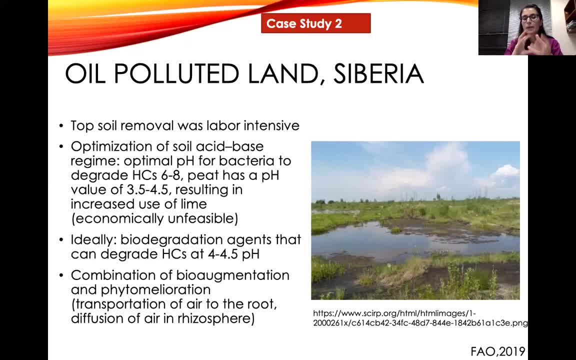 So when you change the pH then you can manipulate it a little bit. But if it's a huge site and if it's scattered in certain swamps, would it be again economically feasible to put so much lime So to neutralize acid you put in a base right? 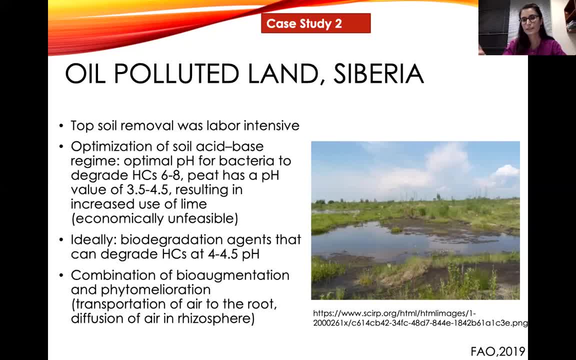 So would it be worth putting a lot of base in there to neutralize it? So all of those questions surrounded this problem. So what they did was they bio-augmented the pollution and they phytomeliorated it. So, basically, so the concepts that we used. 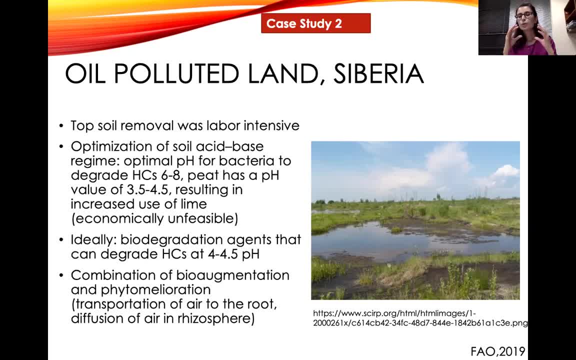 in the previous slide, where you stabilize a pollutant, you kind of force the pollutant to not leave a certain environment. So these pollutants were forced by the plants that were native, that were in the soil, and they were polluted, They were natural to not leave the surrounding. 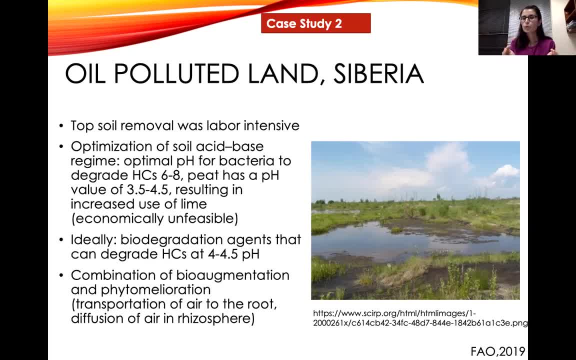 and were augmented or brought in close to the roots of the plants And then they were used to phytomeliorate. So they also provided because there's anoxic conditions. so those roots acted as pathways for oxygen, allowed for those oxygen molecules. 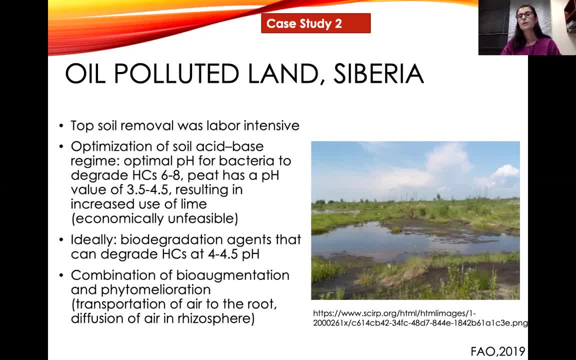 to manipulate the hydrocarbons a little bit, but also allowed for the microorganisms present in the root zone or in the rhizosphere to be able to degrade it, because now they have the oxygen that they needed to degrade it. So all of that thinking had to take place there. 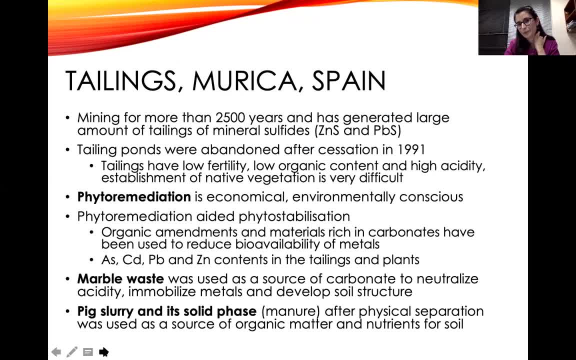 And it was, of course, successful. And that's case study number two. Any questions or comments? so far, Nope, okay, So I will just continue, because this one's the last case study and I don't want to waste a lot of time. 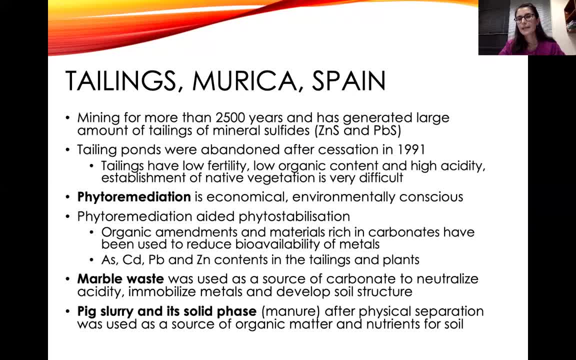 So, basically, this is another site And this site is a mining site and it's in Spain And again, it's also a site that has been used for mining for so many years. But with mining you take what you want. 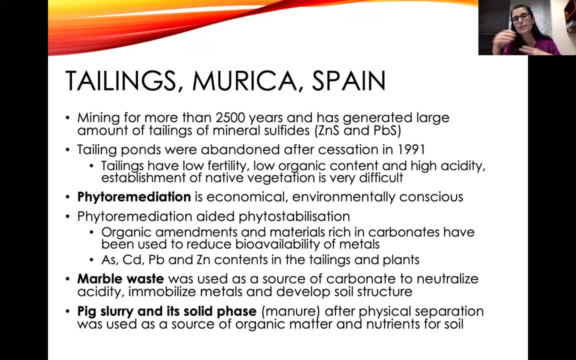 and you use all of these mineral sulfides and other minerals that you don't need behind and they are called tailings And those tailings have no nutritional value, very little fertility, Vegetation, using vegetation to get rid of it. because in the previous two 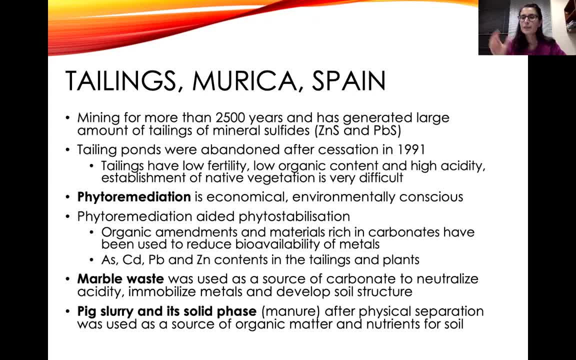 we saw how vegetation had a part to play, But here the vegetation had little part to play because the kind of pollutant that remained, which is zinc sulfide and lead sulfide, or PBS, was, you know, plants couldn't grow in their presence. 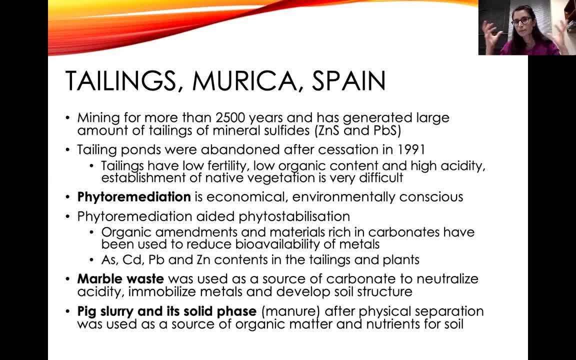 So phytoremediation would have been economical, but how do we bring the conditions down to such that plants are then able to grow in there? So they'd used marble waste, as you know, as a material, And then they'd used carbonate to neutralize the pH. 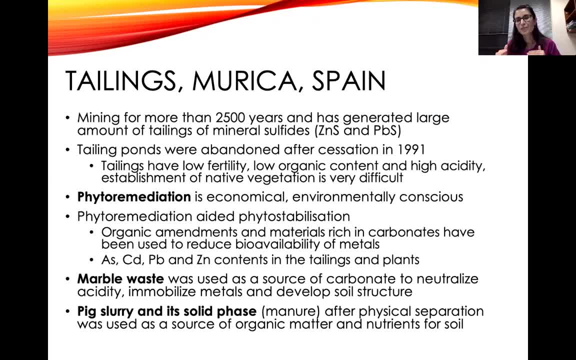 because we know that acid mine drains are mine drains are acidic in nature, So they used marble waste carbonates to neutralize the acidity And then the metals were sort of made immobile And then a pig slurry and solid-faced pig was. 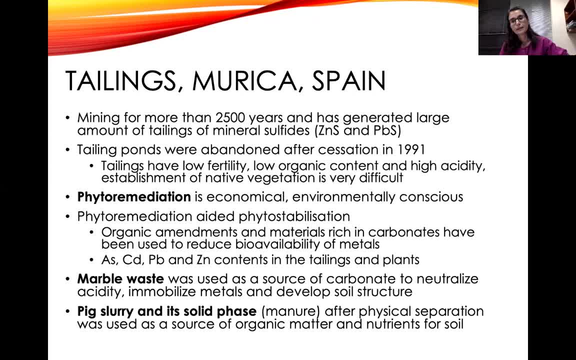 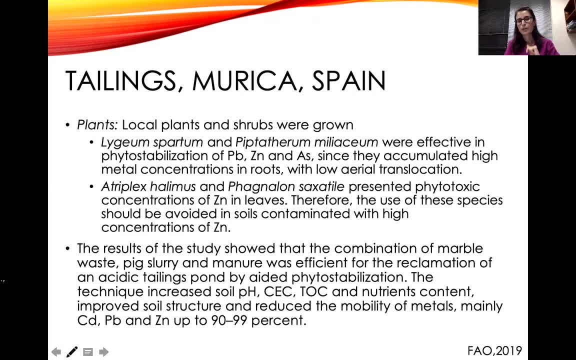 or the manure was used as a food for the microorganisms of plants that were residing there, And then that was used to treat the wastewater. So the local plants, because last time I hadn't mentioned the plants and I think Eamonn had asked what they would be. 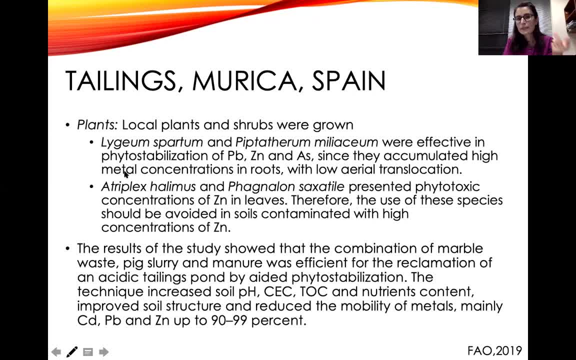 So the local plants were used, and then it was found that some of them were more efficient in removing them, in keeping them, in stabilizing them around their roots and then removing them from the soil. So you continuously, you know, take them out and grow them. 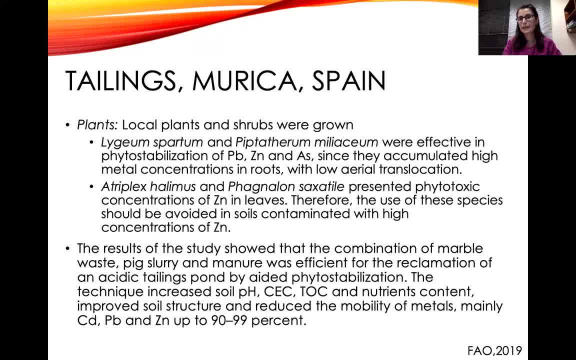 or just cut the shoots and make sure they continuously grow to take that zinc and lead out of the environment, to make the environment clean again. And that combination of marble waste along with the pig slurry or the pig manure worked really well for Spain. 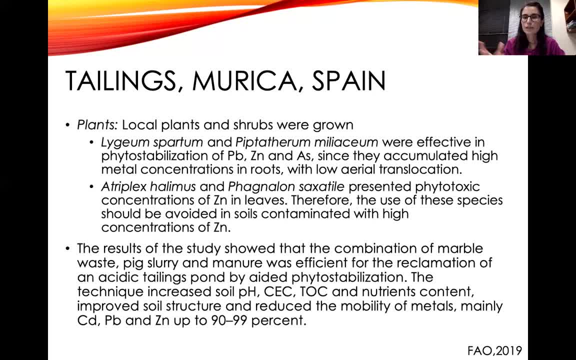 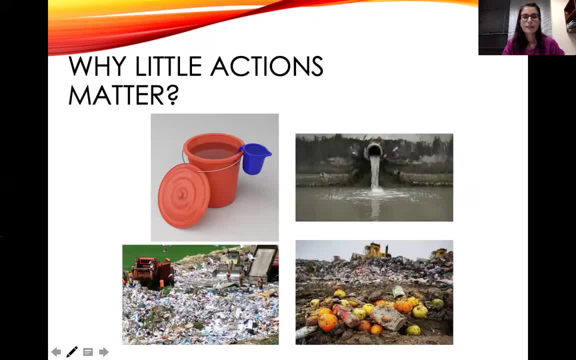 where again, the temperatures could have been different or the conditions, the environmental conditions would have been different compared to the Siberia. So why do little actions matter? Because if I just have a bucket of wastewater and if I put that bucket of wastewater into, 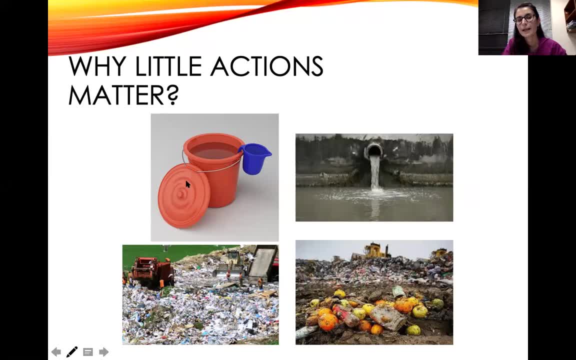 if I have a mug of wastewater and I put that into a bucket of wastewater, I'm basically turning this whole thing into wastewater, And that's why it's important that I make sure that I don't put this mug of wastewater into the bucket of wastewater. 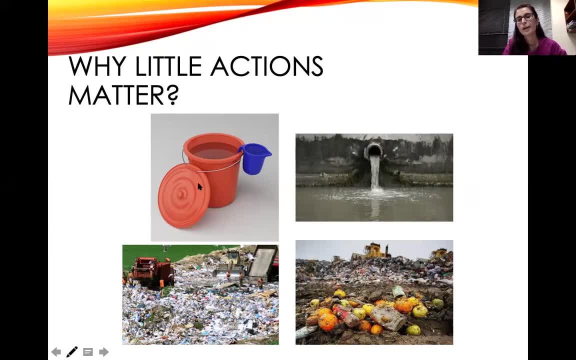 because then now the wastewater has just increased in volume. And that's exactly what we are doing with all the practices You know, for example, us throwing all of our municipal waste into this bucket, this Nala that is passing by us. we are turning a Nala into an, you know. 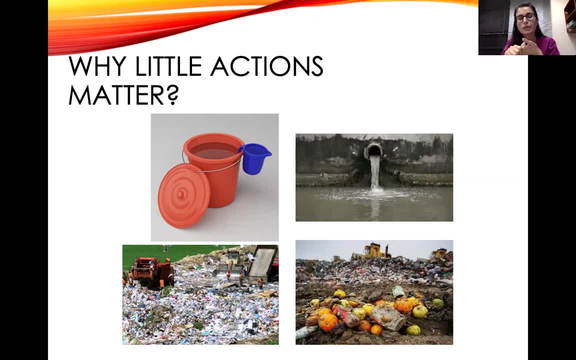 let's say, if it was just a river and it was taking away clean water, by putting our wastewater in and eventually dumping it into Ravi, we are turning Ravi into a wastewater river, you know, And the same could be said for example. 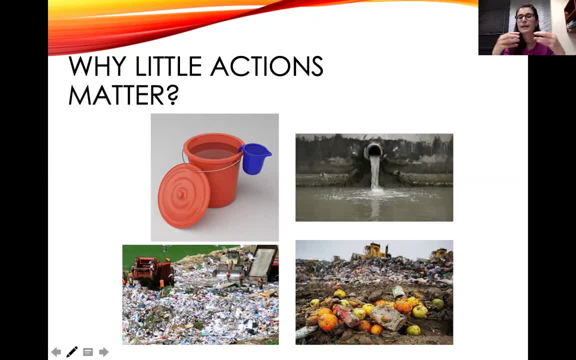 for dump sites as well. A lot of waste that can be harvested, specifically municipal waste that we studied and municipal waste management. The food waste can be reused or, you know, used to make compost. But if we send it there in certain quantities, we need it there, by the way. 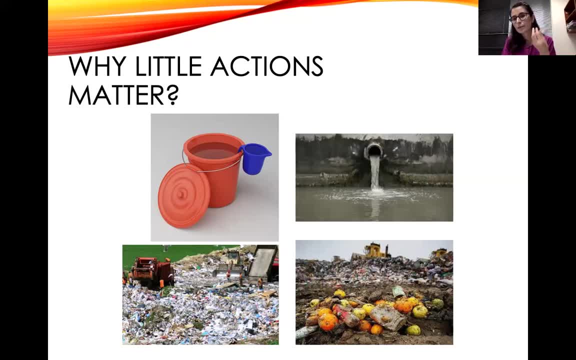 for the same reasons that we studied in the previous slides. The microorganisms need food, and these are good source of food for, and easy to degrade for, microorganisms in the landfill area as well. But excess food and food in combination with, let's say, toxic waste- 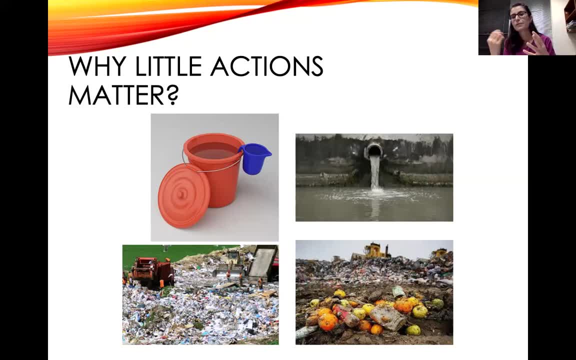 if it's industrial waste that's coming to the landfill and we are taking our food waste and combining them together. now it's a food waste that contains lead or mercury or arsenic, just because we've given them the opportunity to interact with each other. 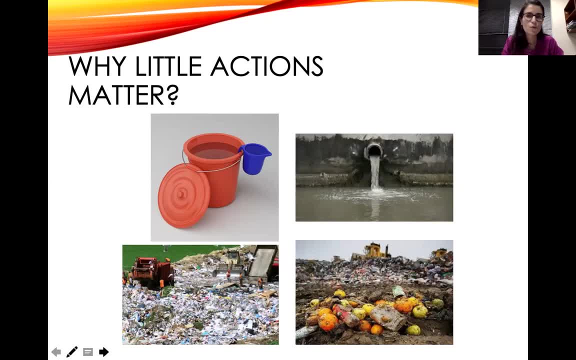 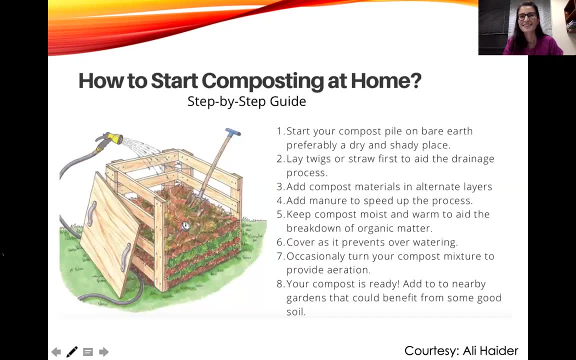 So this is why all the little things that we do at home, at industrial level, in institutions, really really matter. Hassan's using other compliments as well. Okay, is Ali in the class today? Ali Heather, Ali, Ali, you better be in the class today. 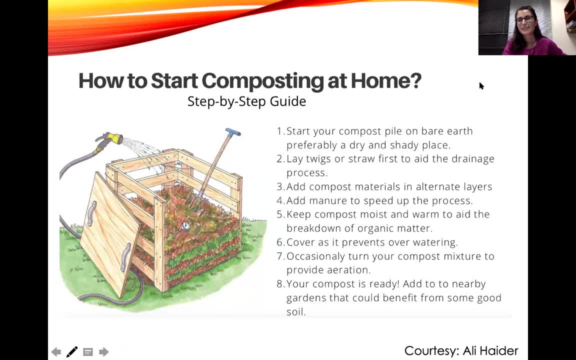 No, you're not Okay If Ali is not in the class today. that just doesn't serve the purpose. Does anybody remember? because I also had given you a reading on how to make compost. So basically, Ali had done this assignment where he told how to make compost at home. 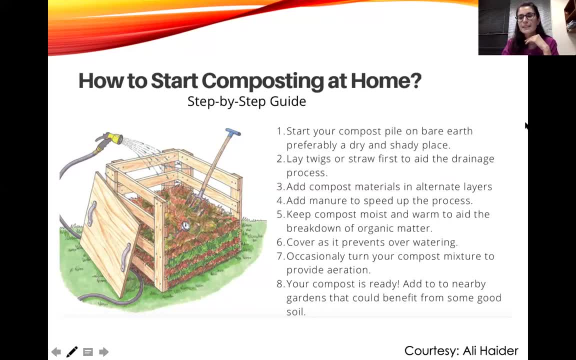 so I put his slides to make sure he explains it to you. But since I've given you a reading, if anyone remembers what you do with composting at home, then please raise your hand and let me know. Even if it's a guess, don't worry about it. 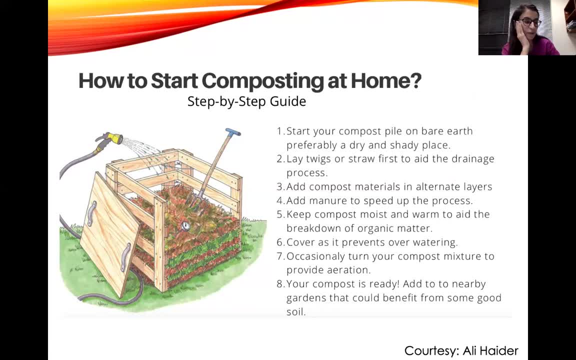 And this time I'm not going to speak until someone raises their hand to explain it. Have you guys decided that you will not talk today? Okay, right. So basically you just use the food waste from home and you give it. it basically needs the moisture. 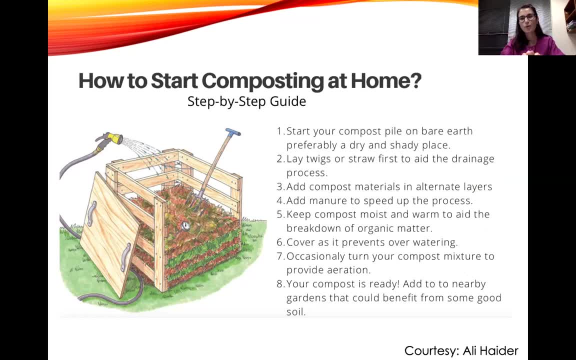 So you would use the food waste? You'd make certain Aadheen go ahead. Yes, ma'am, I just remembered it when you started like telling about it. So it is like these are like waste foods which are then broken down into inorganic compounds. 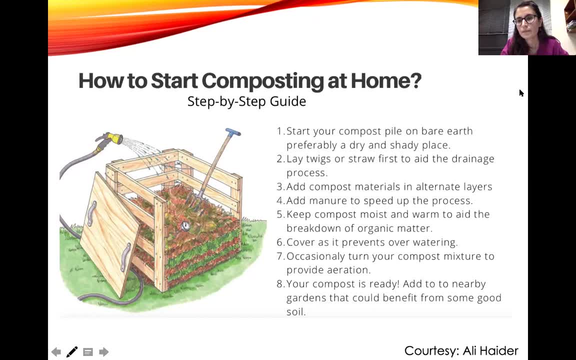 And these compounds serve as nutrients for the soil. Okay, that's great. Does anyone want to? Tai Baba? why don't you elaborate further? Yes, but that's right. again, Ma'am, I was going to say the same thing. 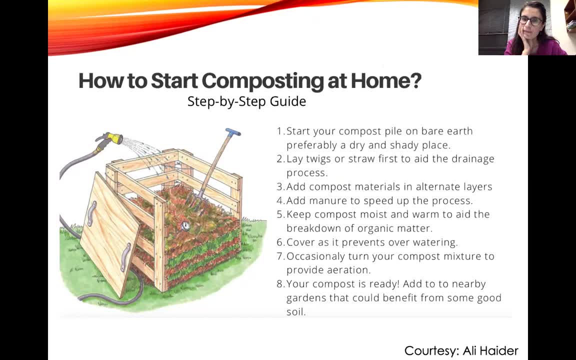 Like we make compost at home and we basically use things like banana peels and then we kind of leave it, And then, you know, we leave it for a while and then we kind of deposit it outside And I think it really helps absorb the nutrients and stuff. 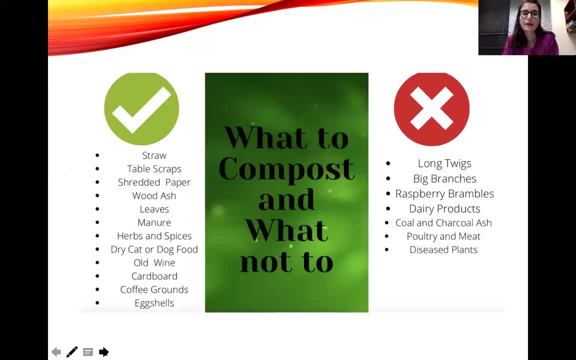 So I think that's basically all I wanted to add. Yeah, so you're basically using all the waste. So kitchen waste, organic waste, waste that can be degraded or biodegraded- So this food waste. if you just leave it outside, it biodegrades, right. 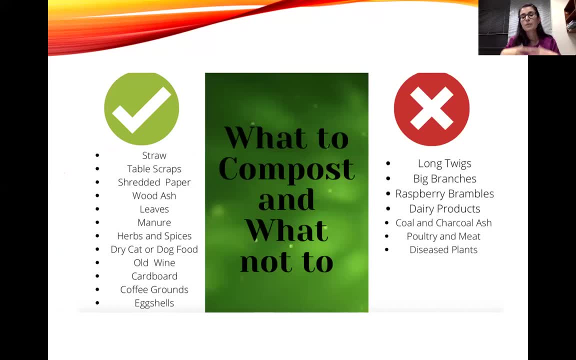 As it loses moisture, as it also some of it will evaporate Sometimes, you know, it just shrinks in volume. So if you leave your apple peel somewhere, it would just shrink in volume. So that's what we want to do when we're composting. 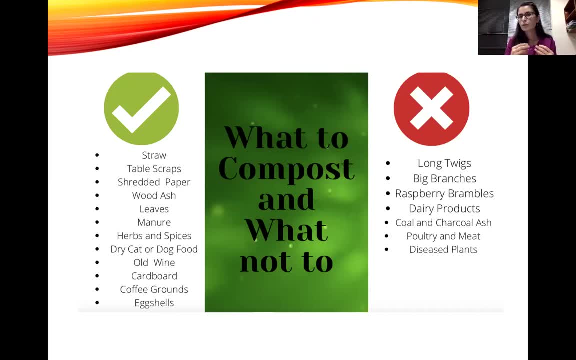 We are converting it into, you know, the soil basically. So we're converting it into organic matter that can be made a part of the soil for plants to be able to utilize it again. And by doing that, Okay, Okay. 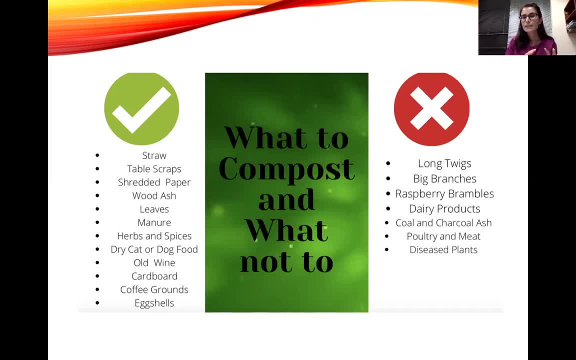 Okay, And by doing that we are reducing the pressure that waste, that is put on the waste collectors. So if I have, let's say if we are, 10 people living in the house and we make all kinds of food, and there's a lot of food waste. 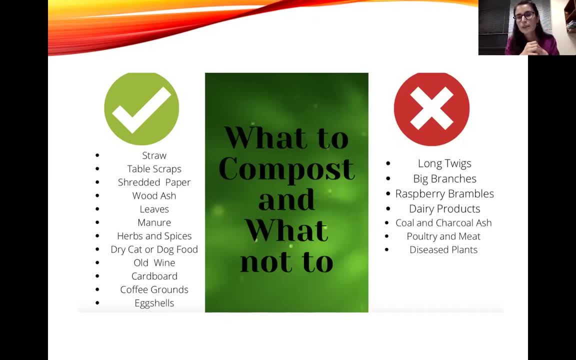 And every day, the waste collector who comes to my house thinks: what are these guys doing inside? If I have, even if I have- a small garden, if I don't have a small garden either, I think you can just do it and then reduce it in volume. 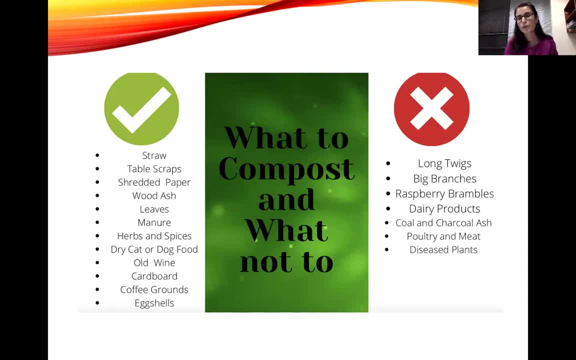 And then maybe give it to someone, maybe give it to the central garden in your, In your housing authority. There are a lot of organizations, by the way, in Pakistan that give you the tools to do it. So, for example, I think Trash It is a company that gives you a packet where you can just put. 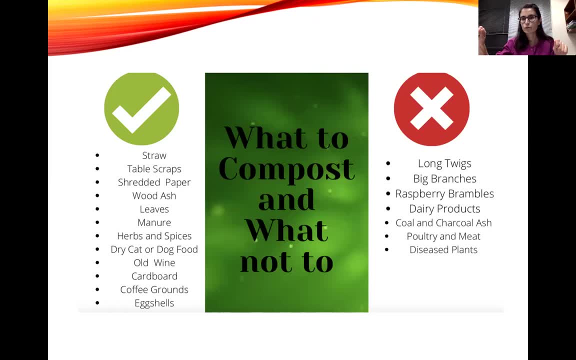 It tells you the recipe as well, So they will tell you what to put in, and then you have to close it and then it gives that condition to the things that are inside, And then it's composted and it shrinks in volume and can be applied to the soil as food. 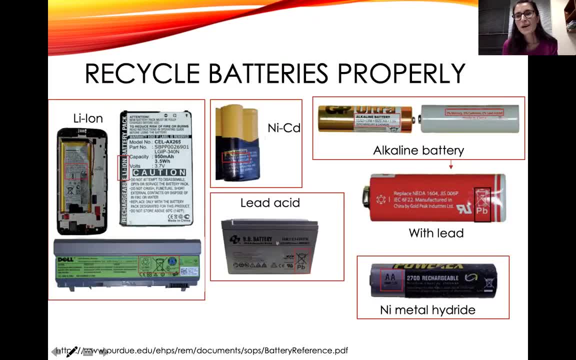 So yes, you're both right. Thank you very much, Aman. you did an assignment on e-waste, So how does e-waste find its way to soil and why should we take care of it? Do you want to speak? 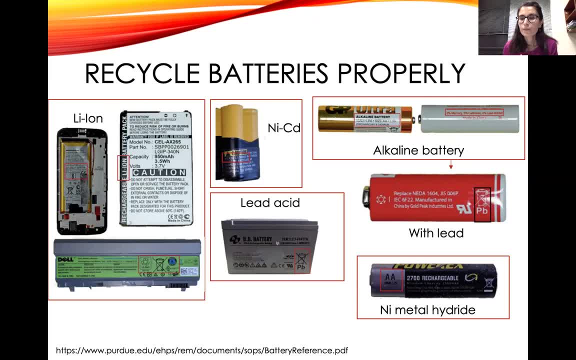 Yeah, ma'am, when we are using something like this, for example a battery, it can be used as lead or mercury, But the electronics are different, For example the monitoring of the computer. There are monitors, and different kinds of materials are being used in the monitors. 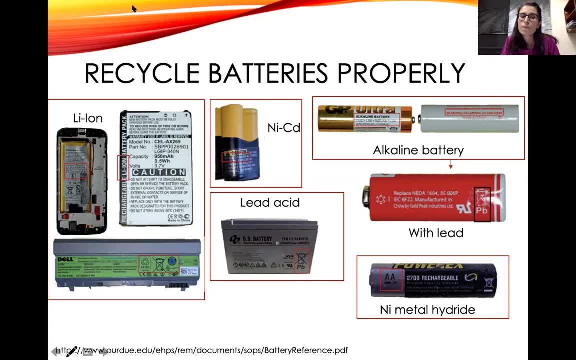 So when we throw them without a proper mechanism, the substance will eventually fall on the land or on the soil, And secondly, when we bury them in the land. what we learned earlier was that when there are harmful substances in the landfills, 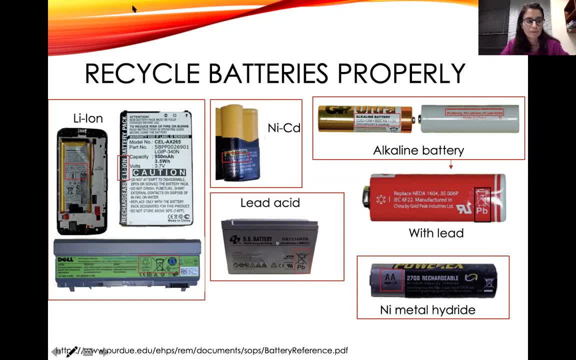 they mix with groundwater. So when we bury them in the land, what we learned earlier was that when there are harmful substances in the landfills, they mix with groundwater. That's why, for them, what we need is not only a proper mechanism. 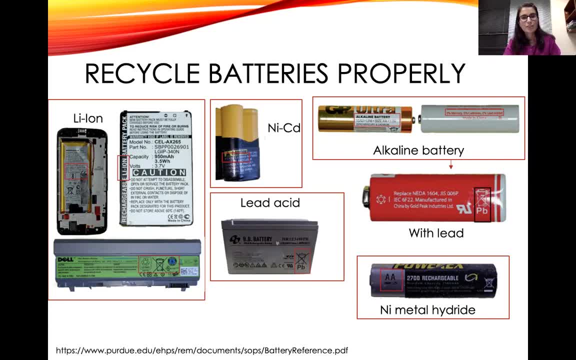 Suggesting a proper mechanism and making sure this material isukefool to now be thrilled. We need to keep this material apart and afterwards be able to discard it Exactly So. we know lead is toxic, you know, we know that there are various changes in electricity. Juan. 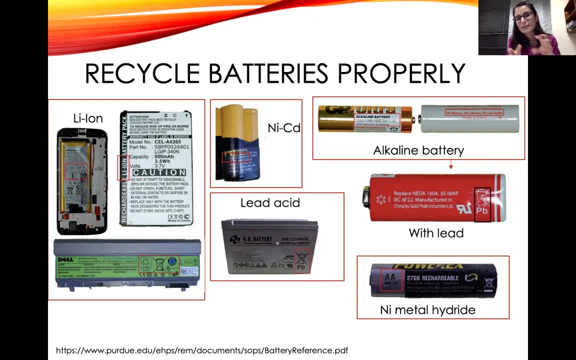 We know lead is toxic. you know. we know that if they have acid or base in them, if it goes into the soil, then we know how pH manipulates the soil qualities. Now there is lead in it. so if you take this lead acid battery which is in your UPS, 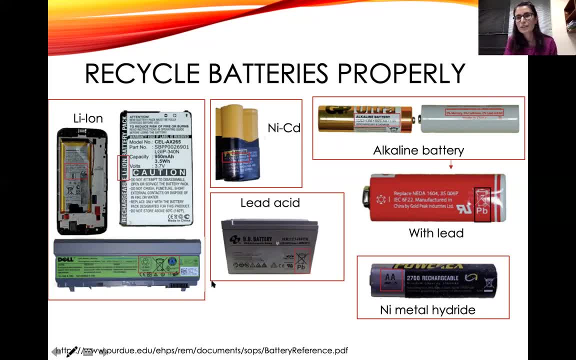 the first thing is that I think all of you, whatever devices you are using, just go and see what kind of batteries are in there, Because up until I had to sort of work out to find out what kind of batteries are there, I wasn't aware of how many kinds of batteries are available around me in the devices that we use at home. 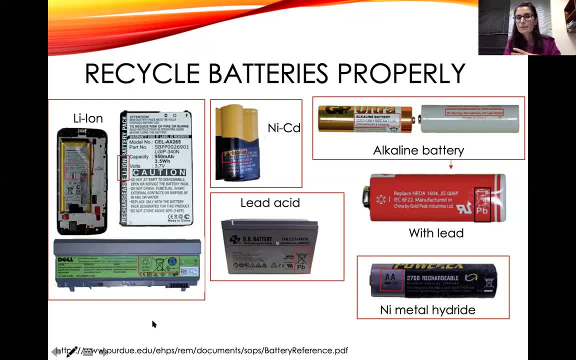 I've just given you a few examples here. You know cadmium is toxic. you know lead is toxic. you know acidic conditions are not good for the soil. you know alkaline conditions can be bad for the soil. So when you know all of this, and then you know that you're using certain things that would end up being in the soil, 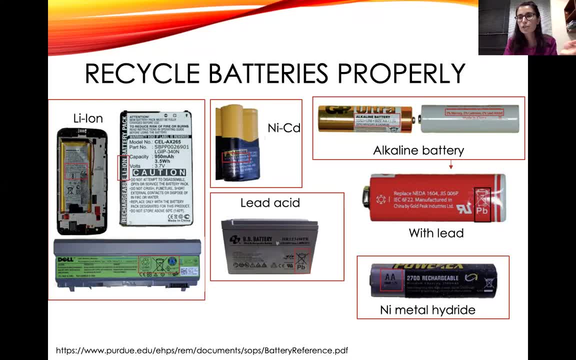 especially in cities like ours, where there's no condition to treat soil, waste, no condition to treat, There's no condition to treat wastewater, then you know what could happen to this. So make sure that this, all of this, should be recycled. 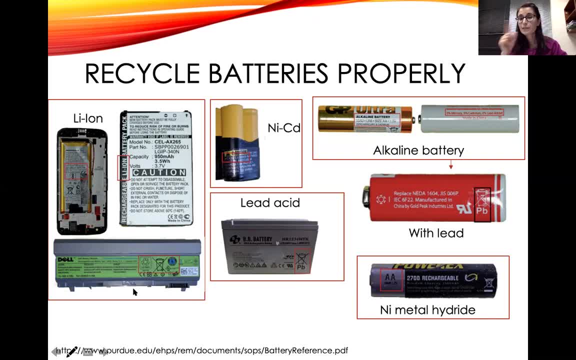 So all the batteries often have this sign that says recycle. It's like: please recycle it, Do not discard it into the environment. Taha, Yeah, ma'am. I just want to add one more type of substance that I read about. 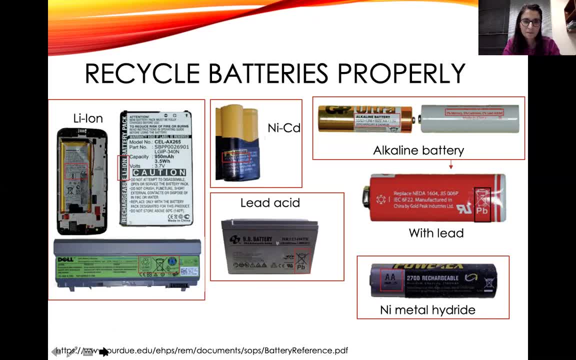 which was brominated, flame retardants which were included in batteries specifically to stop them from combustion for everyday use, And those are also potentially really terrible for the environment. Exactly, Thank you, Taha. So basically, the more good it is for our use, the worst it would be in composition. 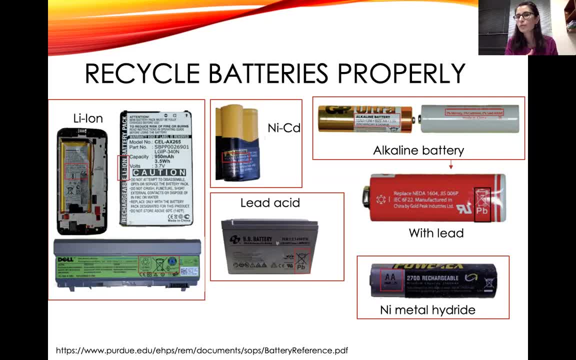 So you're making it flame retardant, you're making it, you know, waterproof. Whatever you're doing, you're adding more and more chemicals to it, You're adding more and more things to it. you know that could simply be avoided by just keeping it into the room. 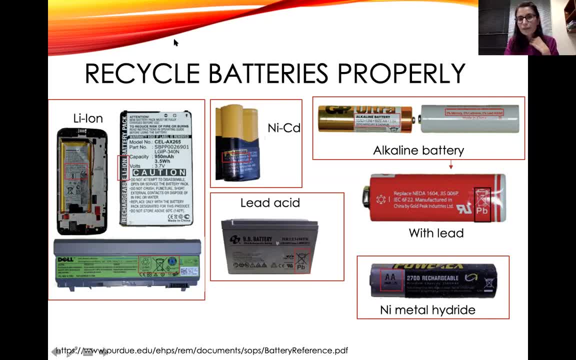 So, or keeping it safe. So you know, these again are just a few examples of the kind of batteries, And you've already known that they're not good for your health or for the health of the environment. It's just, I think, again coming back to, like I said, being conscious and doing, making those small changes in your life. 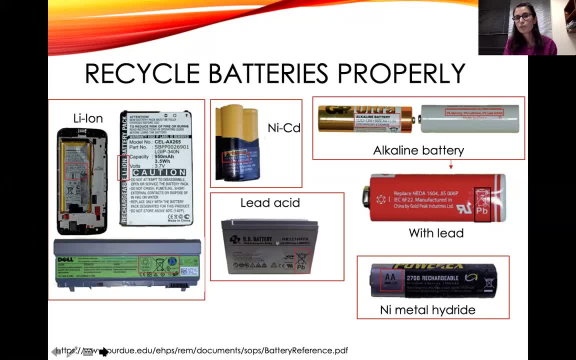 So if you have something running on a battery and you're just changing the battery, for the sake of it, I would say, just not have it in the house. You know, of course, in academia, in other institutions, you have to have them. 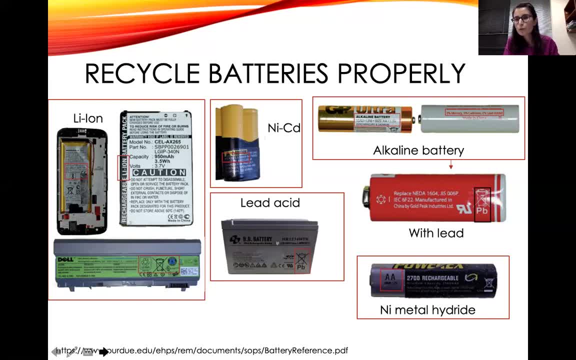 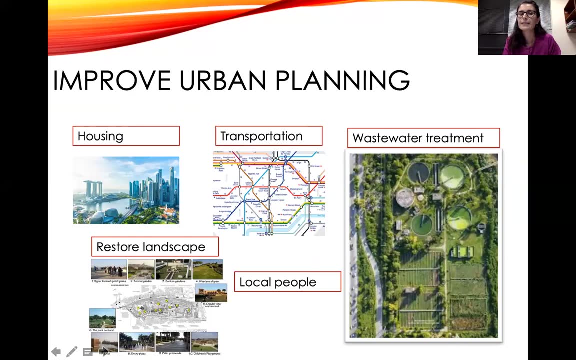 So you use it, But whenever it's not needed, Don't use it. And whatever you're using it, make sure the battery- things like batteries that have all of these toxic chemicals- are recycled. So yeah, And the next thing- and I think this you guys can talk about as well- is the improvement in urban planning. 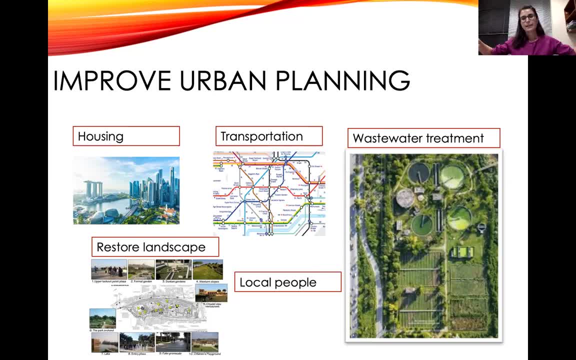 What are we doing to Lahore? We're expanding it literally, horizontally, or whatever the direction is, And then you know it's. we're claiming all the villages From all across, Expanding the city, And guess what? The city doesn't have a wastewater treatment plant. 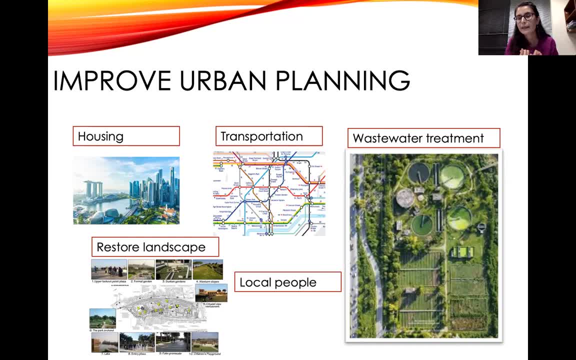 The city doesn't have a clean water supply assessment, So there isn't one single parent company that provides clean water to you. So WASA, if you ever speak to them, would say that this is the official boundary of Lahore that we serve to, because all the other boundary is not Lahore. 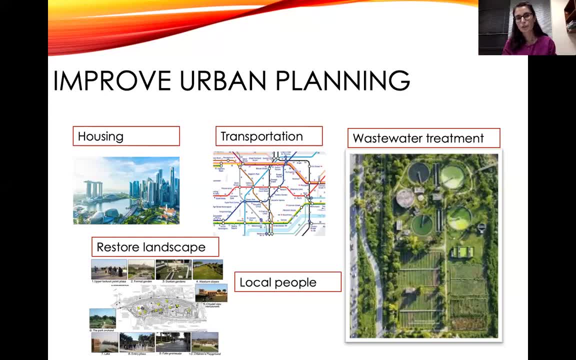 It's something that has expanded And we do not provide services to this. Then these housing societies have their own water provision and wastewater, you know like they take care of it themselves. So having a central body to make central decisions and making it useful for the environment just becomes so difficult. 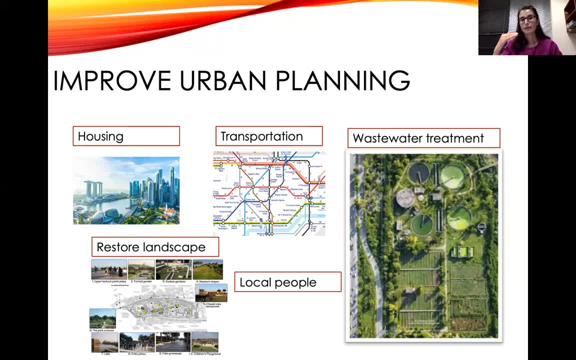 And therefore I think urbanization in particular had the most role to play in maintaining soil quality. And someone rightly mentioned that flooding is important. It's been increased. Flooding in urban areas has increased 100 times because we have reduced green spaces. 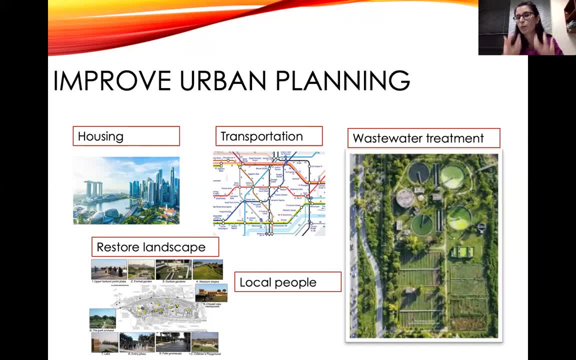 We haven't left those kind of sponges in the soil where water could be infiltrated and floods could be avoided. So all of those things, I think, are because of improper planning And they result in: if you're not, if you haven't designed for your city to treat wastewater, then your city, all your city, will have is gandanalas. 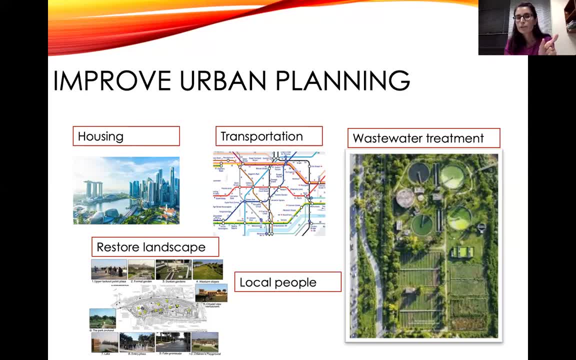 If you don't design your city, If you don't design your city for public transportation. I put the picture, the map for London tube in there because it literally connects the entire city to all the stations. So maybe the remotest of places, like even a village outside of London, you could simply go to, because past that tube line there would be a bus. 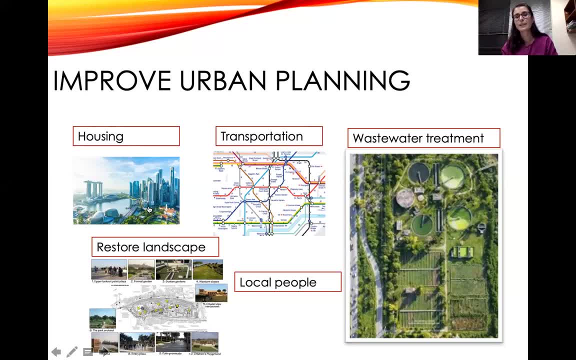 Even if it goes once a day, it would be there for you to be connected to the city, which means you don't always need to drive your car. Unfortunately, the cities here have been designed to for cars. They haven't been designed for people who want to walk. 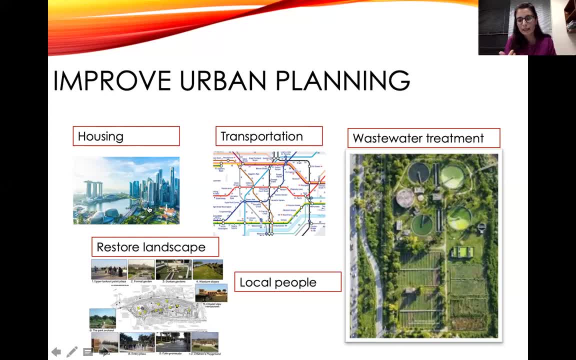 They haven't been designed for people who want to cycle. There are no cycling, There are no biking lanes. There are no walking lanes. Where in DHA do you see walking lanes for people who are walking? You just have to save themselves from accidents and walk. 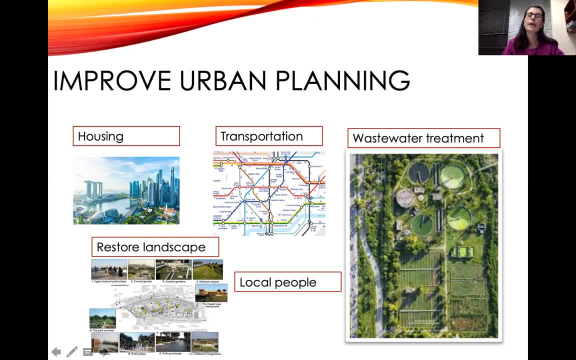 So I think a lot of the soil pollution and water pollution and air pollution has to do with improper urbanization Or just everyone running Right Or rushing to the cities because there are more opportunities in the cities. What should we do? Of course we should have plans for wastewater treatment, which we will be talking about in a while. 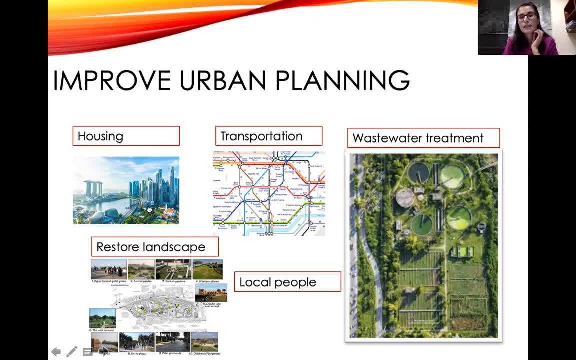 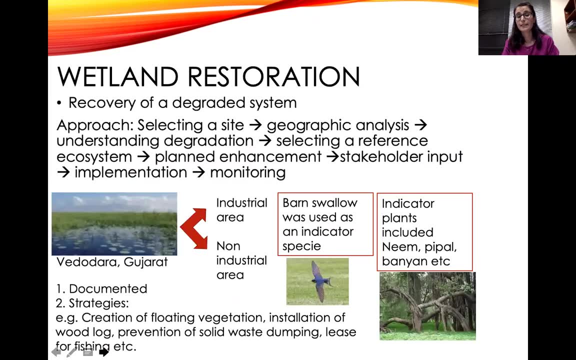 We have very little time, And then, wherever we can, we should restore our landscape, Give cities those green spaces that they need- And again, I'm using a few examples- And people who want to talk about anything, just raise your hands. 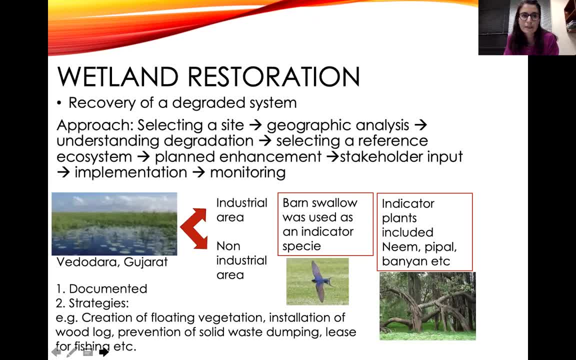 You're more than welcome because I would want you to be active in the classroom. Wetlands were mentioned in the class again and again. This particular wetland is in India, Gujarat, where they basically monitored sites. It was yes, Taha. 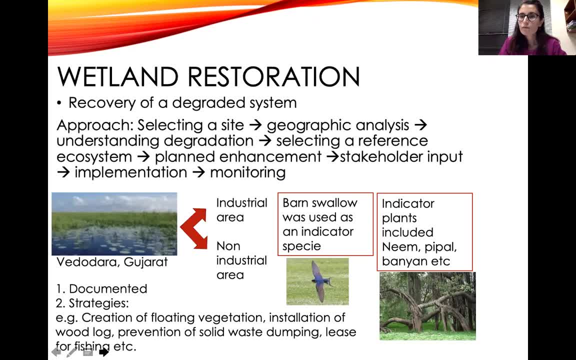 Ma'am, I had a question about somewhat a thing we talked about a while ago, which was the first case example where in the Ivory Coast, the land was contaminated Right. So in that regard, you also mentioned that contaminated land can very often contaminate the groundwater underneath that land as well. 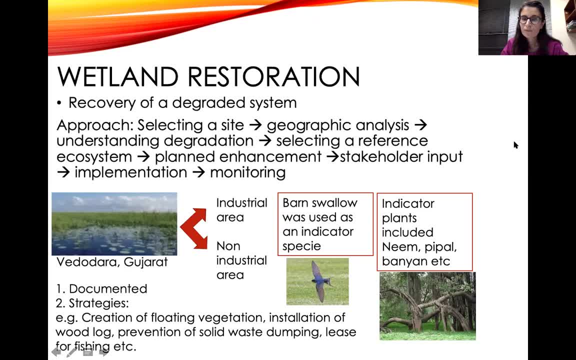 So in that regard, like how land is restored using methods such as all those you talked about, how would you deal with the water that's underneath that land, The water that's underneath the contaminated land? Yeah, So like I said in the beginning, oftentimes if the soil is contaminated, the underground water is also contaminated alongside it. 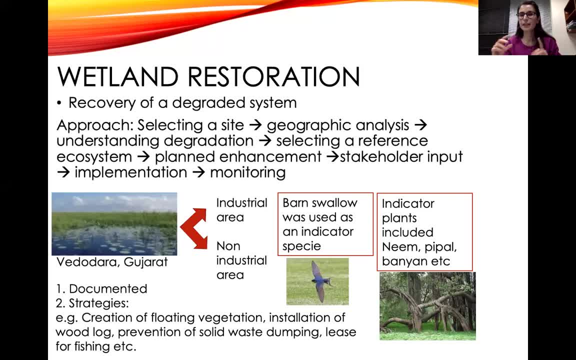 So when you say wash pump and treat, it refers to that particular system where you're washing all of it from the soil, extracting all the groundwater, bringing it to the surface, treating it there, because it's difficult to treat contamination in groundwater. 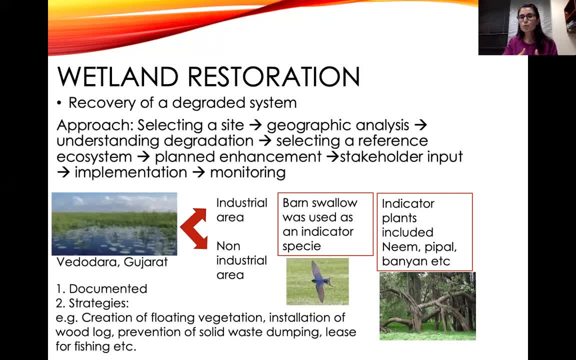 And then you would use the same method, right, Right, So you would use the same method, right Yeah, So you would use the same method, right Yes, So you would then put it back. You would also use certain tools. So, for example, the electroplating method, right. So you know that it would be difficult for you to, for example, go down and see what's going on. I think I put a term for you to Google, which is a machine that has the ability to go there, not only extract samples, but also treat it and monitor it. So there are those commercial mechanisms available for you to see what's going on in a particular area, But you would basically, as I said, you would use the same method to treat contamination. You would also use the same method to, for example, the electroplating method, right? 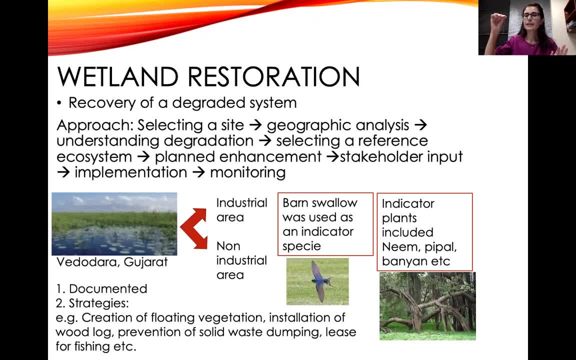 Yeah Right, a machine that has the ability to go there not only extract samples but also treat it and monitor it. so there are those commercial uh mechanisms available for you to see what's going on in a particular area, but you basically whatever method you're using, and it depends on what you choose. 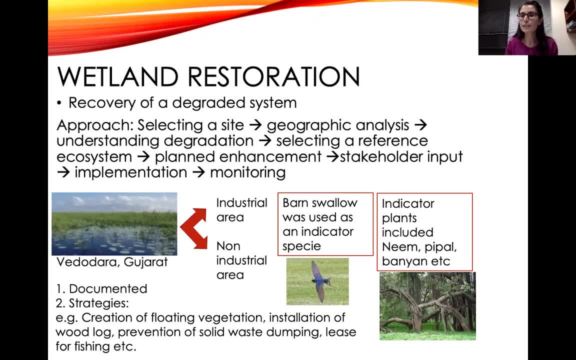 and what's the contamination there? and and how difficult is that? if it's a, if it's an aquifer, if you've contaminated here and then that aquifer just moves and the next time that you will have to trace the pollutant and treat it few miles away from the city, downstream somewhere, and that 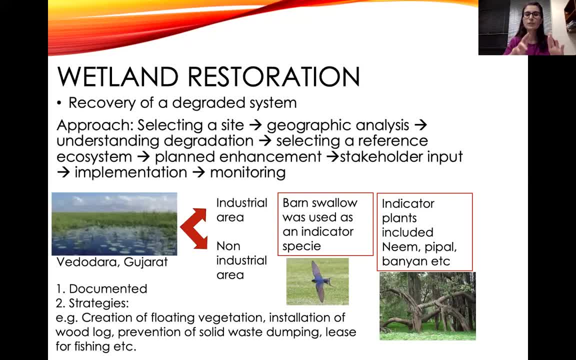 depends on the flow of groundwater. right that means that you will treat this particular part of soil separately, monitor that groundwater pollutant, extract it to at a certain other point, because if it's going somewhere else, specifically if you're extracting groundwater for um drinking, so let's 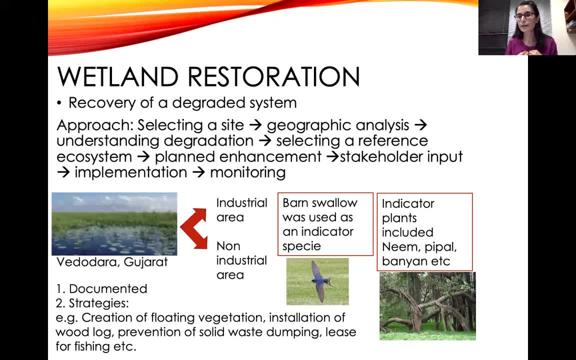 say, if i'm, we have installed a well here and we are drinking water here and a pollutant was thrown away from it because we're extracting water. that pollutant would come towards the drinking water source, which is why your drinking water sources should also be monitored. 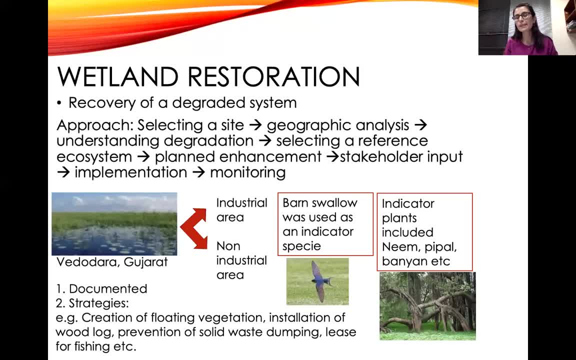 because if they're close to industrial sites, that means that you're prone to these chemicals as well. so it's, it's. it's quite complicated, but generally these soil remediation techniques have are kind of coupled with groundwater remediation techniques as well. so, um, yeah, i mean that's as simply as i can. 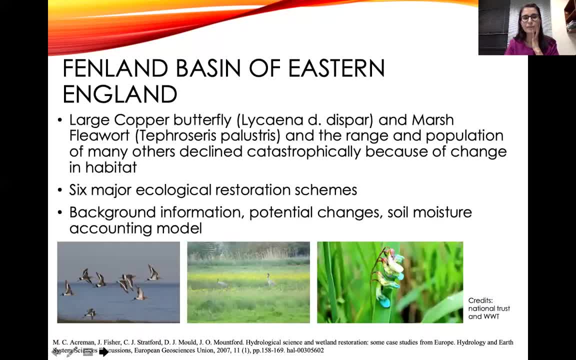 uh, okay, so so, for example, i'll just leave this one, let's just go to another one. so basically, wetlands, we know, are those corridors for, for species. they were neglected in a lot of spaces, but now people are restoring it back um and and wetlands can be both natural and artificial. 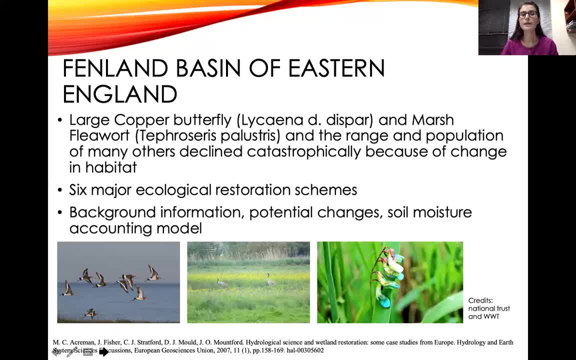 some wetlands are built artificially to treat wastewater. here i've quoted examples of two sites, both india and england, where they were naturally swamped marshes and wetlands. but when the species started disappearing, that's when again they were alarmed and that's when they started monitoring it. they started making the the environment friendly for. 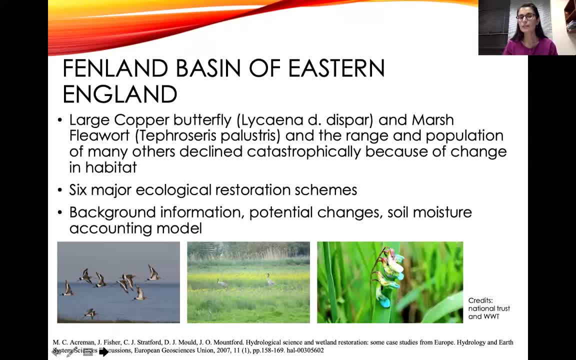 wildlife again stopped certain activities, put in all the local plants and grasses and shrubs, and then, you know, looked at, monitored it and saw it to recover again. and, like i said, these are not one year, two year, three year projects. these could be one decade, two decade, three decade projects. so imagine what would happen to our 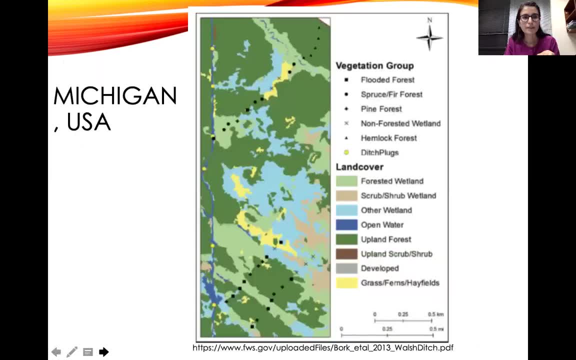 country when we start remediating it, probably five, six, seven decades anyways. so people had talked about um geographical information system. i mentioned it somewhere. um, this again is a rgis map where it kind of tells you that in a particular wetland, what kind of wetland are you referring to? so then the monitoring and control becomes easy. okay, this. 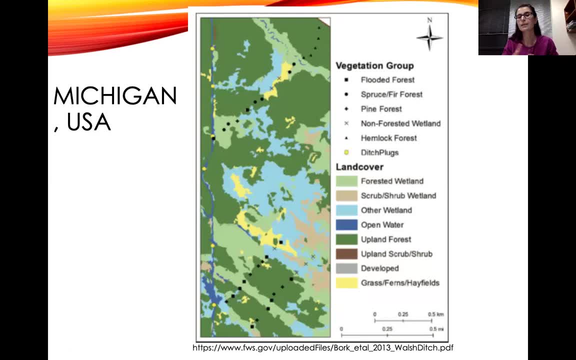 is a really simple way to monitor flora, so you can see the spread of the water in the area, uh, and you can see a little bit of the smallелен species. it has some um ETA and, as i mentioned, there's a lot of inhibitions, if you're looking for. 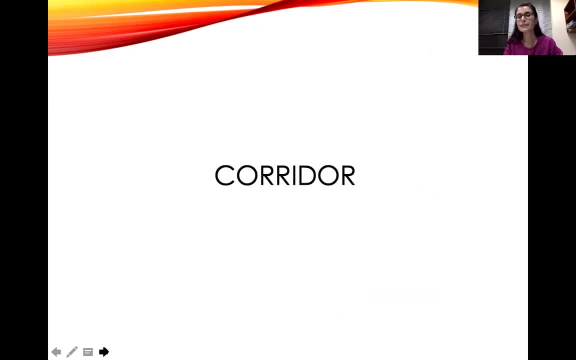 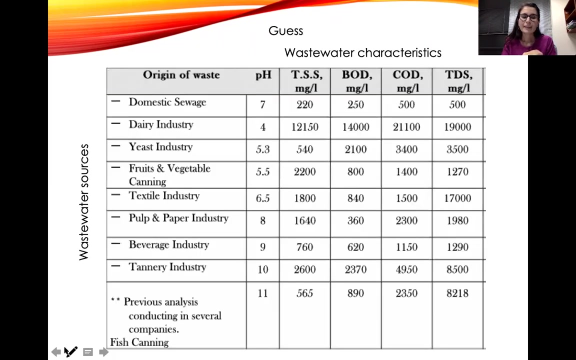 um, systemic affects for much of this area, especially if you're looking for, uh, the early summer season. so that means the PI system, which is really important, and we can also monitor the habitat of some of the wild birds, which is what you see here. save our species. so i just wanted to put that word in. 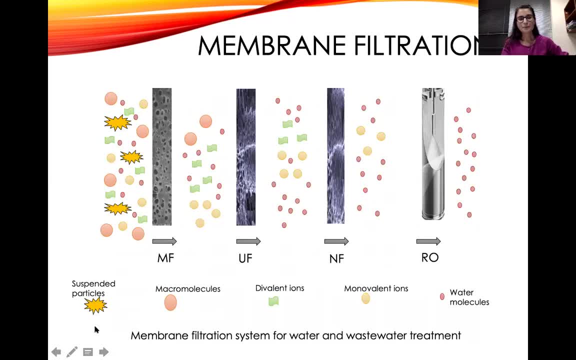 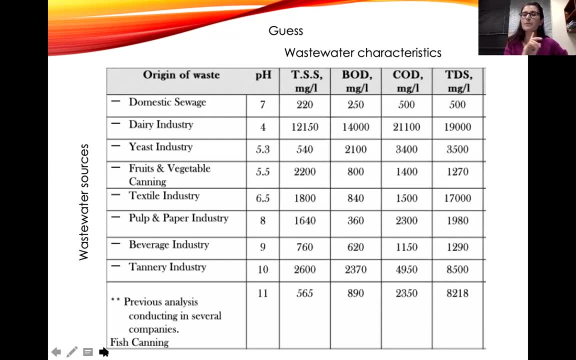 now we are coming back to basic filtration techniques, because i have taught this to you and this i will not talk about it. i'll. it's again coming back to what we had looked at when we were looking at um chemicals that could be present in wastewater: the national environmental quality. 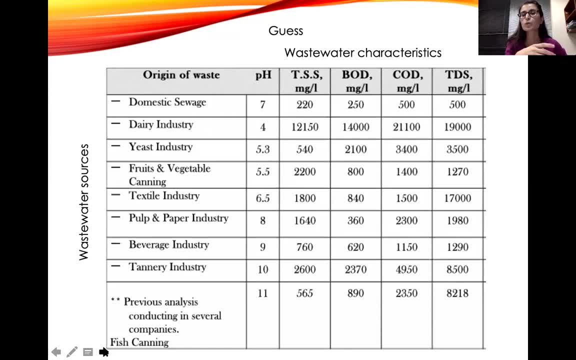 standards. why is it important to have a standard? because we do not want to lose the natural habitats, such as wetlands and soil, and we do not want that kind of degradation where we end up having just barren lands or or deserted lands around us around us and, you know, be hit by even square poverty. 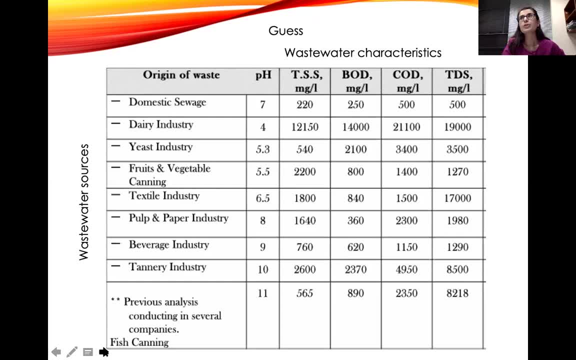 so this particular slide i shared with you in one of the lectures and i told you to reflect on how the bod, cod and tss- total suspended solids- is the turbidity of how many solids are there. so that's i'm moving my hands and thinking about. as hans comments, i'll stop moving. 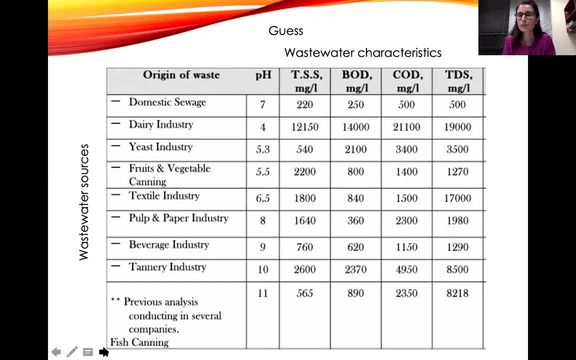 my hands. but basically the tss is the total suspended solids that are um that are there in the in the wastewater and um and based on that you know. for example, if the wastewater has a lot of tss or suspended solid, it would be difficult to treat it using light. so, for example, if the water body requires light, 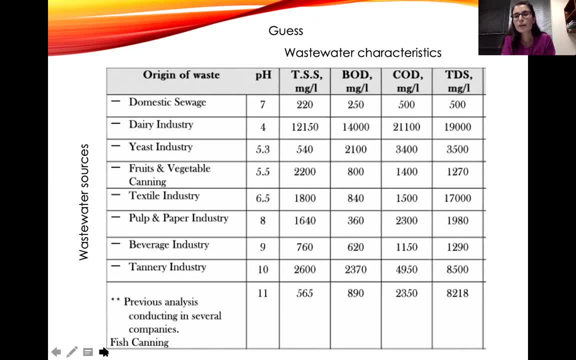 and there's a lot of tss in it. uh, if the might be microorganisms in there require light, that means that the tss would stop light from getting in there. so what would you do? the suspended solids are the ones that cannot settle, so if they're big enough, they should technically settle. 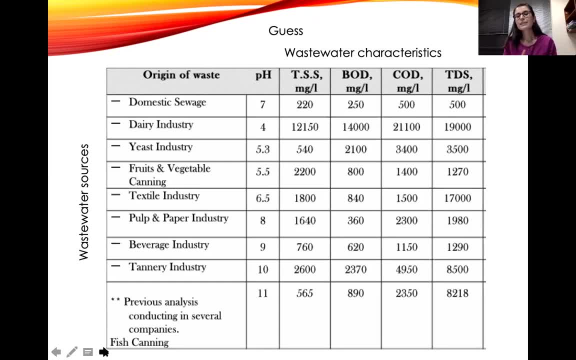 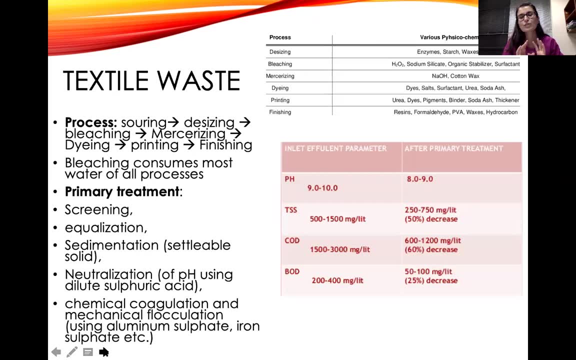 and then you will take that one out first and then whatever is in suspension, you'll think of ways to treat it so as an example. and i hope this is fun, because just just try and enjoy this example. i know it's complicated, but i'll try and make. i'll. 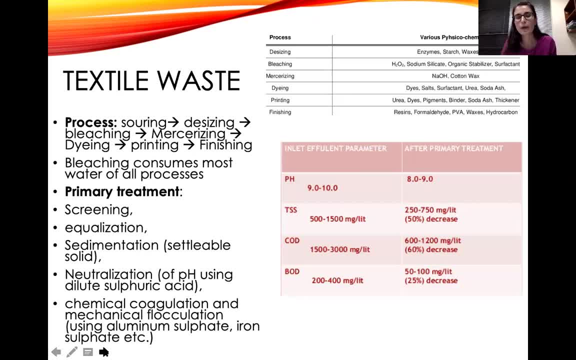 try and simplify it. we're all wearing clothes we enjoy wearing, wearing colorful clothes. i was thinking about which particular industry to bring in when i'm thinking of ways to treat the wastewater of that particular industry, and because we are a country that grows cotton, you know our textile has, has had a good reputation- i thought to 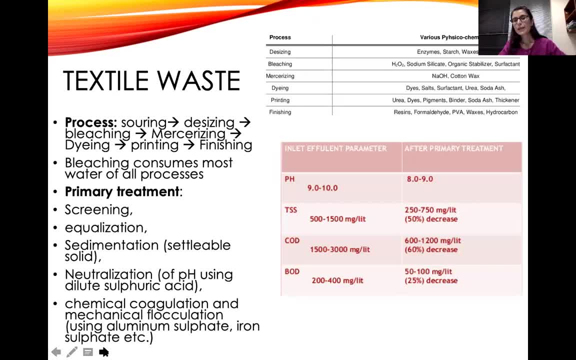 to bring this forward as well. so of course, every industry has a processing. that processing has a certain kind of pollutants associated with it. the treatment process depends on what kind of pollutants are present in the processing or in the raw material or in the final product that you. 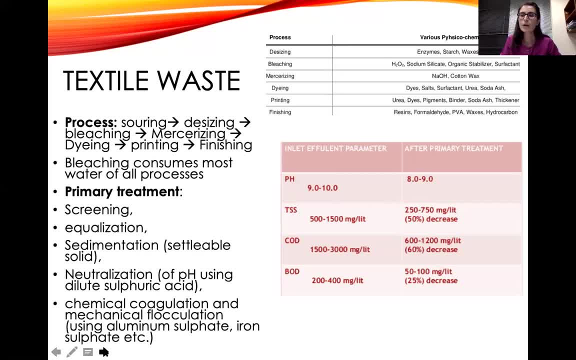 take out of a certain industry. so in the industry we are making a fabric, but in the process of making the fabric we are bringing in cotton, we're bringing in plastic, we're washing them, we're using certain chemicals such as bleaching. so if we bleach it then we'll definitely have hydrogen. 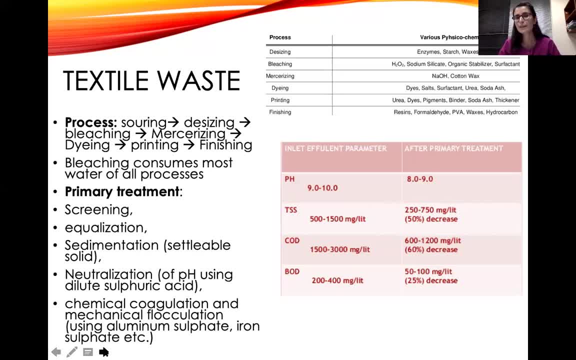 peroxide. you know, you don't need to be a scientist to know this. everyone knows that bleaching has um h2o2 or two in it and it's not that good. so if you put it on on a cloth it would just decolorize it right. so when you know, 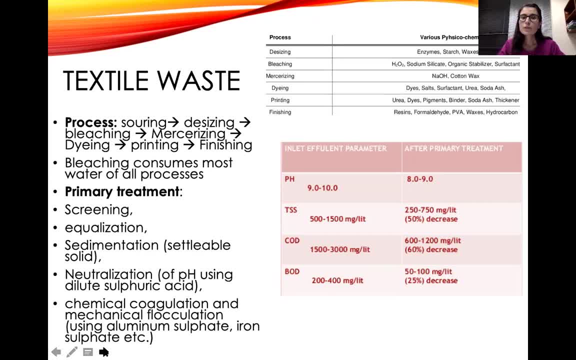 that a certain chemical has that kind of ability, then you want to make sure that this chemical doesn't end up going into the environment and for that matter you have to treat it. oftentimes industries are put in what you call industrial zone, where they have a combined 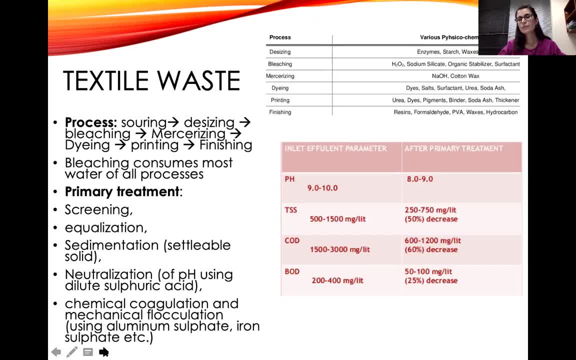 a wastewater treatment plant so that they can take all of these things out and then send it to the city's wastewater treatment plant. very few industries in pakistan treat their wastewater, but if they could treat their wastewater, how would they treat it? so even for municipal wastewater and 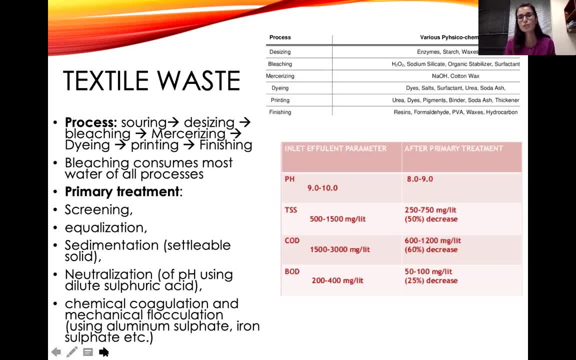 industrial wastewater. the first process is to screen it. so it simply use a sieve, you know something with, with pores bigger to to retain all the plastic, the trash, anything else that is available to treat that puree, the moisture that was that actually produced, that came with with it. 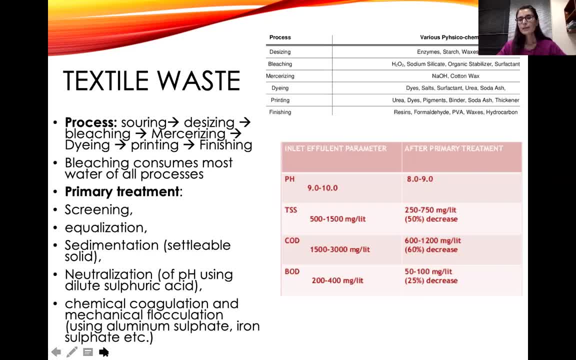 then you would allow for it. so the equalization tank is basically like the source tank, where you put all, all the liquid in. then there is sedimentation. like i said, if it has suspended solids they will settle and whatever is on top is claimed and taken to the next step. 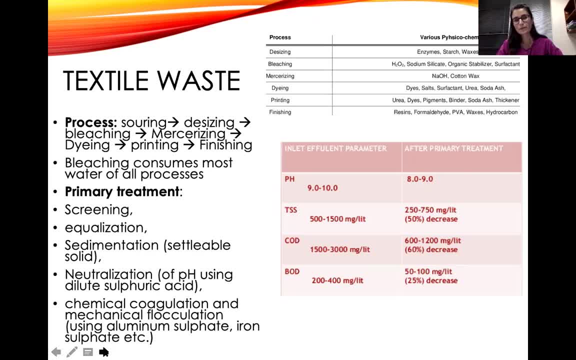 you neutralize the ph. if it's acidic, you add base to it, if it's basic, you add acid to it, and then called coagulation or flocculation, where you so: okay, now this: the ones that could settle have settled and the ones that couldn't settle are suspended. so what would you do to this? and 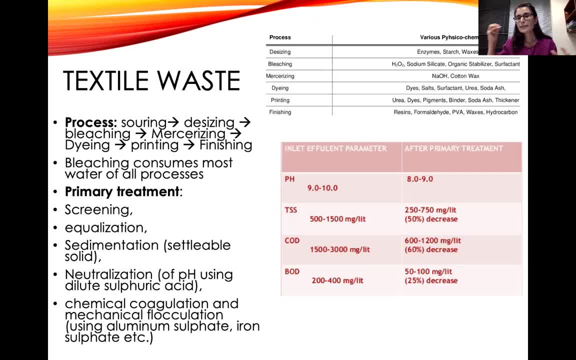 suspended, you would either filter it or you would add a certain kind of chemical that would bring it together and coagulate it or make bigger flocks of it. so that's what you do in the next process. so these are primary treatment, because in this you can't take as much suspended solid as much. 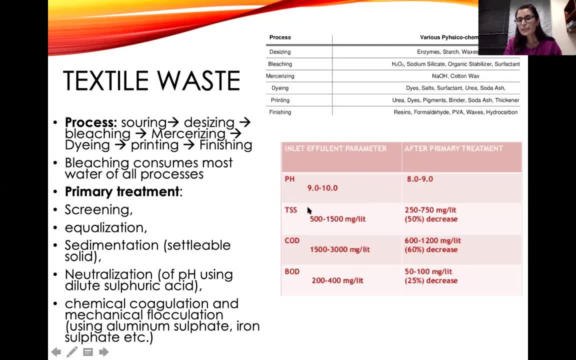 chemicals away as you can, but if you look at this table where, after it has been primary treated, a lot of things have been reduced down to half, so some people who do you know who have, who are sending their waste to a secondary treatment plant, the, the treatment plant of a city might. 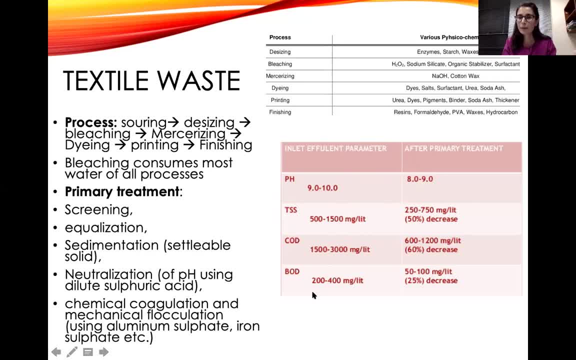 just send it with these conditions so they may just introduce primary treatment at the industry and then after that they would. they would think, okay, now it matches the municipal waste or or another waste, and then we can send it to the conventional treatment plant for the city. they can do that here. if you look at it, the BOD is still high. it has only been reduced by 25. 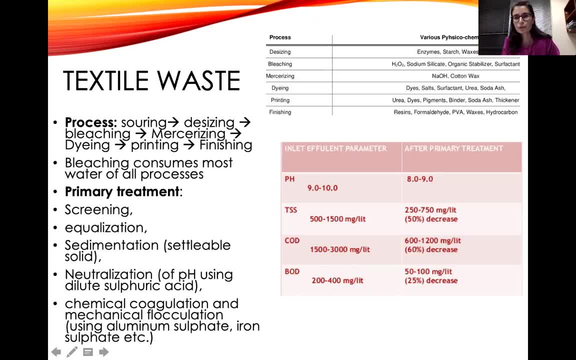 percent. the rest of them have been reduced, but the beauty hasn't been reduced. so what do you do then? you now use the microorganisms or the life protozoans- anything else, algae, fungi- to utilize the nutrients. right? so that's what happens in this secondary treatment process. 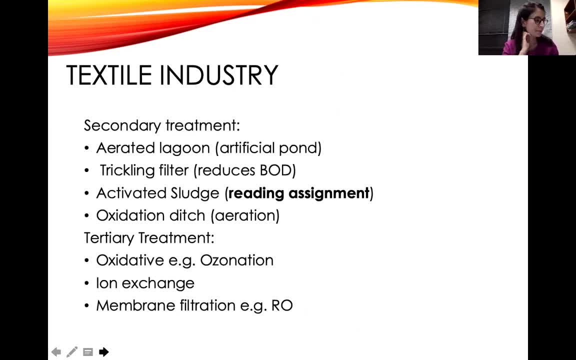 where it's. yes, rapid ma'am, can't you just do reverse osmosis filter, get through school, push curdling the? I was waiting for someone to say this. yes, you can, but you know what happens. this is kind of solids, can form a very thick film outside, and sometimes do it because 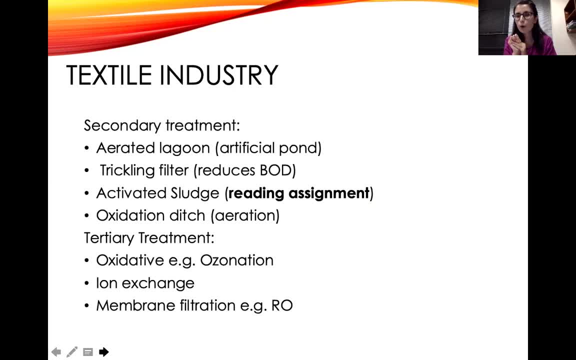 what happens is there is a film growing on the, on the wall of the filtration. so your pressure it's. it's a high pressure filtration system, which means you're applying, applying a lot of pressure on this membrane, reverse osmosis membrane to take all the clean water out, which is possible, I mean. 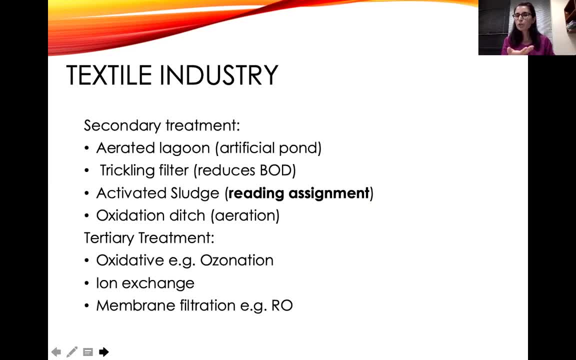 you can reduce the pressure and and clean the membrane continuously to make sure you do that. but that's you know that increases the work for you and it's expensive because it uses a lot of power. so what they would do is they'll. so what they then do is you know they don't use it because 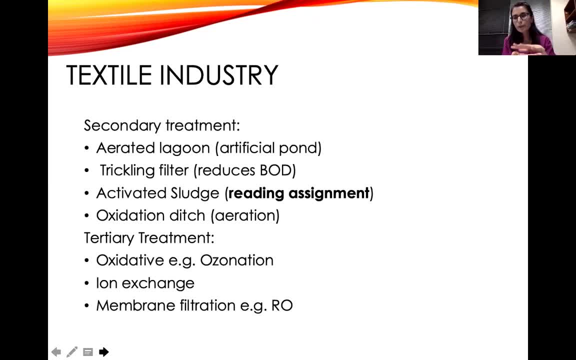 the more film grows on it or the more things settle on the wall on the membrane, the higher pressure they have to apply. and if they keep applying the pressure, then the membrane can just tear down. and that's exactly what happened when I went to Jordan. they had basically installed a 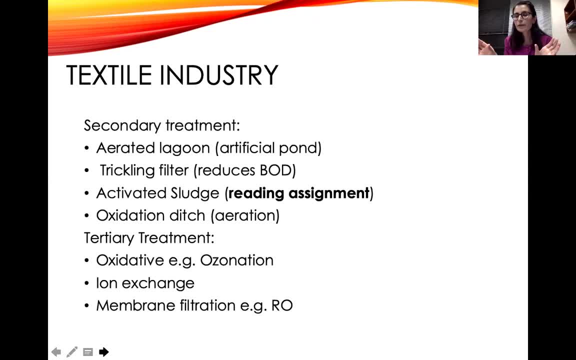 micro filtration, not reverse osmosis, a micro filtration for membrane bioreactor. but because the strength of the wastewater was really high, it had very high COD, very high VOD, you know, and all kinds of way things in them, suspended in there they were continuously using. 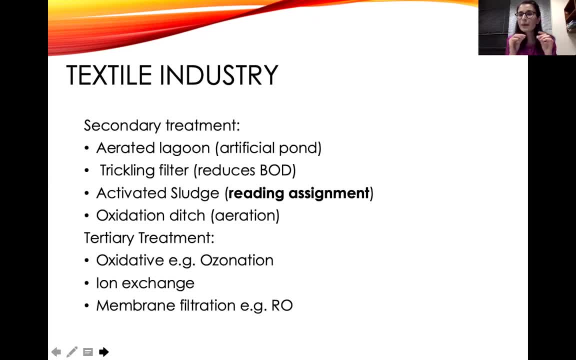 it and and what happened was, within a year, the membrane clogged or the pores clogged, and the administration and had an issue that you know it shouldn't clog in a year, because they told us that the year the membrane will work for 10 years, and then I had to go down and explain the design. 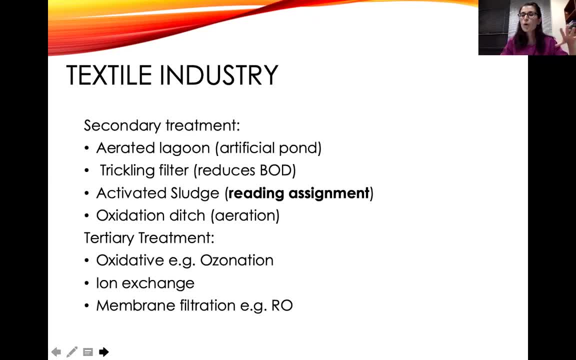 principle to them and tell them that this is exactly what happens when you do not operate a wastewater treatment plant for the design conditions that you set, because they hadn't designed for the treatment plant to operate at such high concentrations. so, yes, you can and no, you cannot. it depends. so if there's anything, yeah, like a clogs in a year maintenance, and you like, 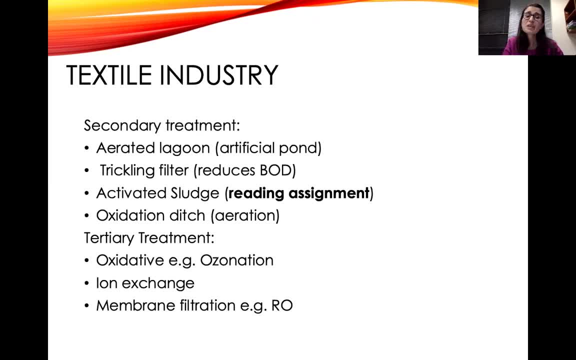 change your uh filter after like a week, uh, nine months or so. you can't. you can't change the filter and clean it. for example, with my PhD study, what I did was I was also continuously cleaning the membrane with acid-based Solutions, basic solutions. I think I was continuously cleaning it to make sure. 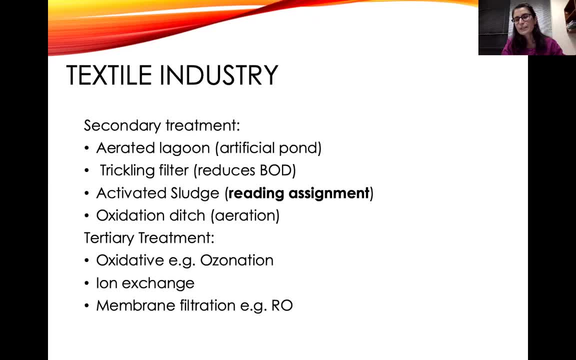 that every time I run a process or every time I run a filtration setup, I have the membranes completely clean. so then you know the pressure, the cake doesn't. so let's call it cake. so the cake doesn't build on it. but for textile I think it's just the acidic chemical, so it depends on the 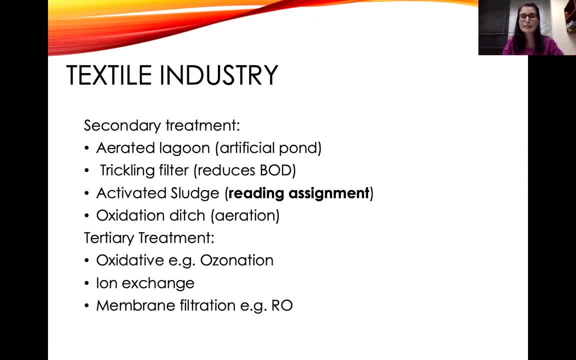 chemicals. if the chemicals can damage the membrane, then you would use something else. but to be honest, you know that's what I would think, because I'm pro filtration side also. I like the suggestion, uh, and then you know. so all of these are basically just having septic tanks in the open air. so 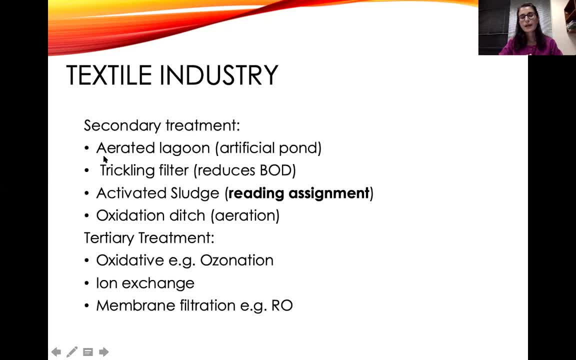 erected Lagoon is just having that tank there. the trickling filter is a bed. we've discussed this before. you're just using a medium again for wastewater to go through their bacterias there and they eat the nutrients slowly. the water passes through and it has basically reduced the BOD remarkably. 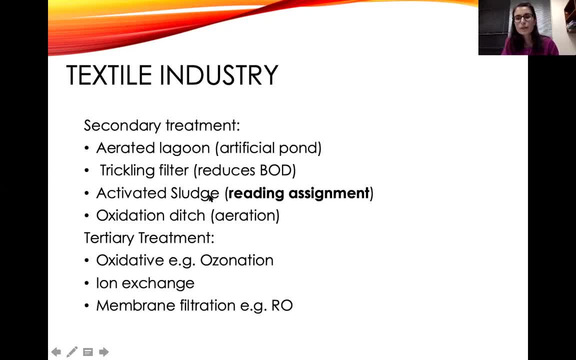 and activated sludge. it's in your books. this is the mechanism that's used for municipal wastewater treatment, so conventional wastewater treatment. I think I'll give this to you as the reading assignment. go back to your reference books and read what this process is. it's fairly simple and 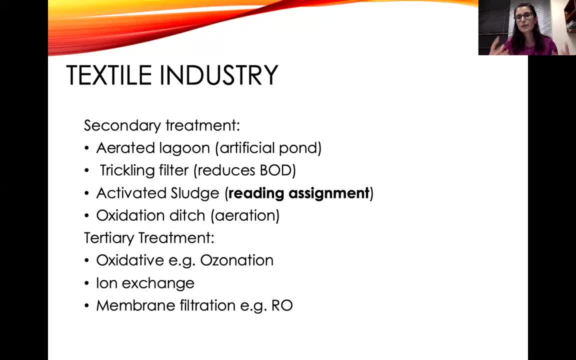 oxidation. ditch again is something where you aerate it yourself to make sure that bacterias quickly degrade the chemical. now- because last time I didn't mention I hadn't mentioned water vapors- I realized that ozone is also used for as a tertiary treatment. so the last step if you really want clean, clean, clean water in. 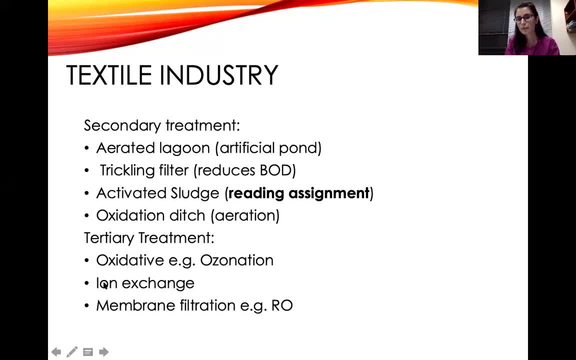 the environment. the last step is using things like membrane filtration. so because now the initial load is really low, the water is mostly clean. you can now use things like arrow, because then you don't need to apply a lot of pressure. you can do take clean water with light pressure as well, but ozone is. 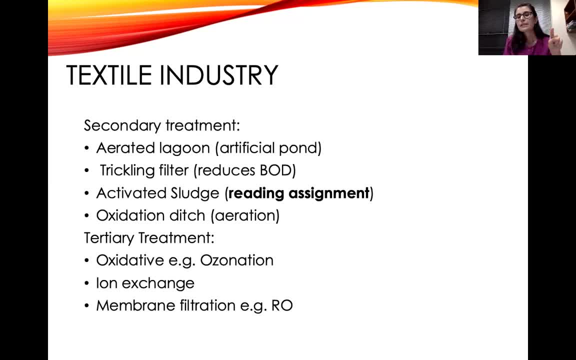 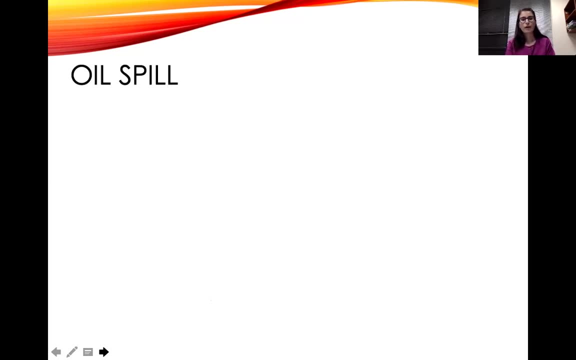 very reactive and because of that ability it is used in the tertiary treatment to treat water. so anything, any chemical that's remaining in the water still, people use ozonation to to treat it. so I just wanted to mention it here before I leave you guys and two more examples, and then we'll 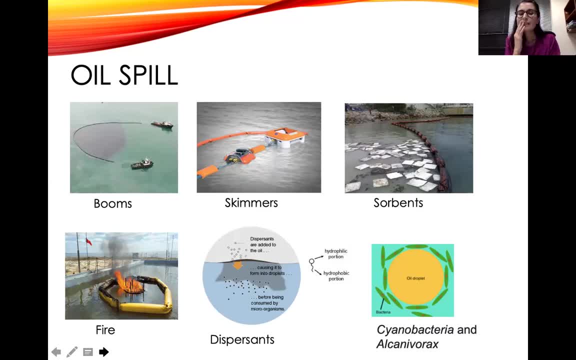 finish. how much time do I have no time at all. so oil spill. does anyone want to just guess quickly what's happening here? basically, oil is light, it stays on top. yes, uh, no, roughly. no, you've already spoken, someone else needs to speak. so oil is light, it stays on the surface, and then you can skim it and, uh, treat it so you. 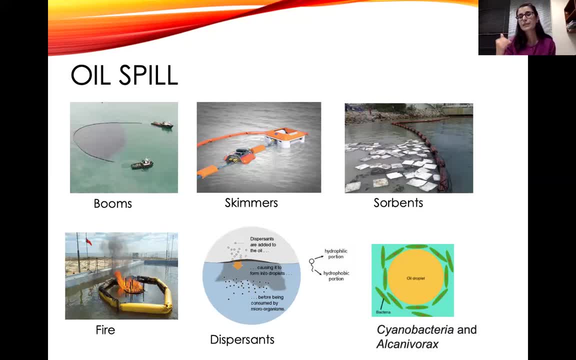 extract it, you treat it there, you can burn it, you can use certain chemicals, such as surfactant, to disperse it, because you don't want the birds and everything else who are dipping into to get all that oil. um, or you can use microorganisms or absorbents or certain kind of sorbents to take that chemical out. 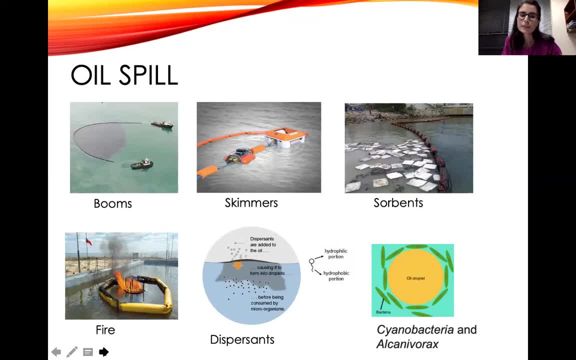 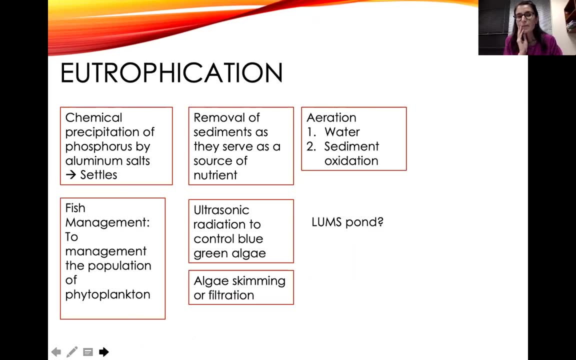 from the environmental uh system as soon as possible. so you know this is another example that you looked at. for eutrophication, again with a topic that many of you like, there are many ways to treat it. one simple way could be continuously taking the algae out until the nutrients go down. 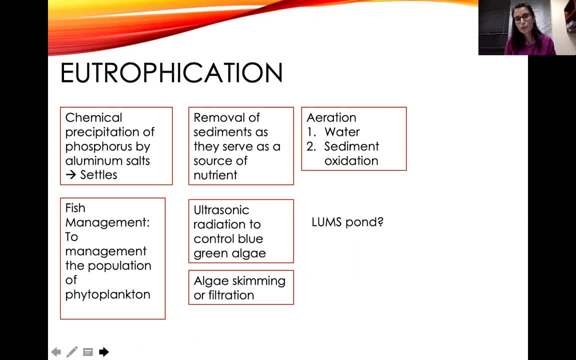 the other would be to treat wastewater, make sure nutrients don't get into the water body. another could be using ultrasonic radiations to to control the algae that that causes eutrophication, or harvesting fishes, or putting fishes in there after skipping the algae to make sure that they eat the phytoplanktons and then there are no. 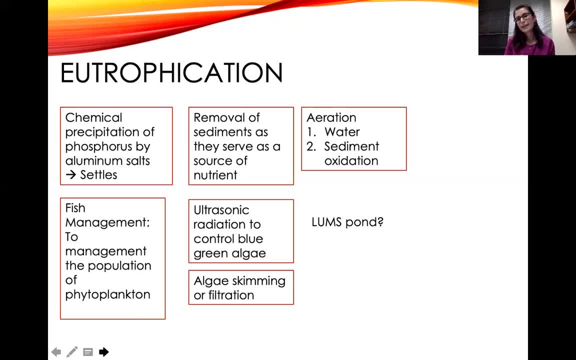 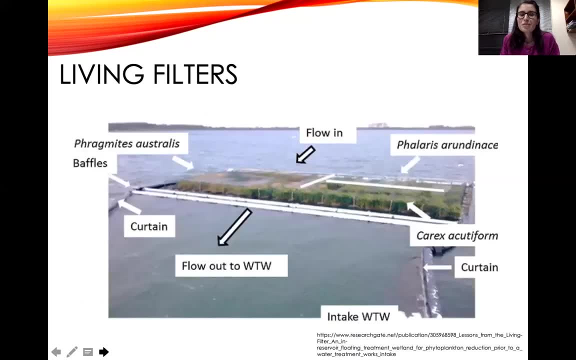 phytoplanktons remaining for algae, who also need to feed on this, and then kind of stopping the process of eutrophication. should I talk about this? okay, so this is because I've always presented algae as a monster. it's not a monster, it's just utilizing on the nutrients. this is the water supply of Oxford, so basically. 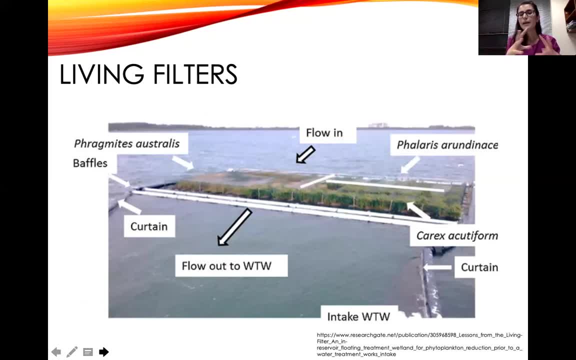 what they've done is used plants and cyanobacteria as a living filter to feed on any nutrients that are there. the water is generally clean, but just to make sure that when the water is coming from the watershed and entering this water supply body, so let's say it's travel Lake of um. 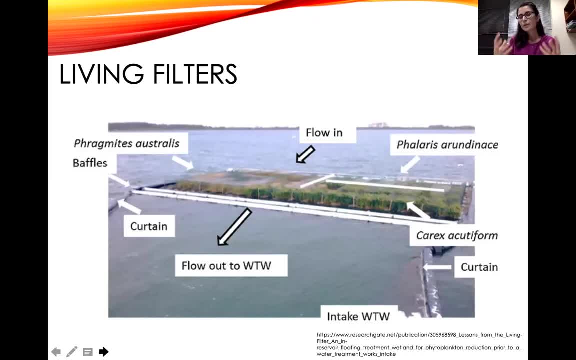 Oxford. then what happens is that they use these plants to feed on those nutrients and make the surrounding water clear and then send it, after a little bit of treatment for drinking, to the city. so bigger plants at the bottom, in close to their roots, there are algae that are going there to. 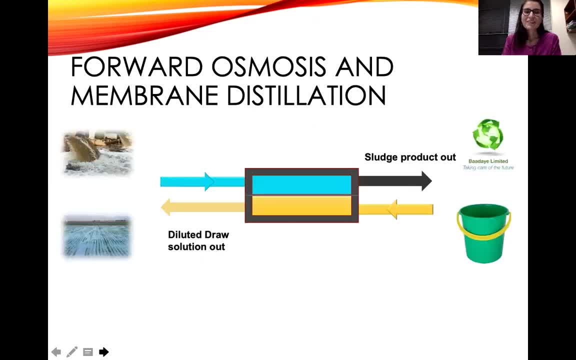 so many slides. why did I make so many slides? okay, right, so this is my PhD research, where I combined two membrane technologies to treat wastewater. so let's say that if there's wastewater or sludge going on the one side- and in this particular case I'm using a, let's say, a fertilizer, because it has 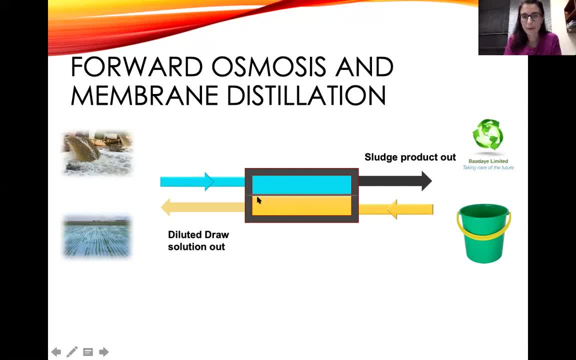 an osmotic potential. I'm using that as a draw suit. there is a membrane in here, so one is passing from one side of the membrane, the other is passing from the other side of the membrane. what I want for want for it to do is for the water in this wastewater to pass through and come here. 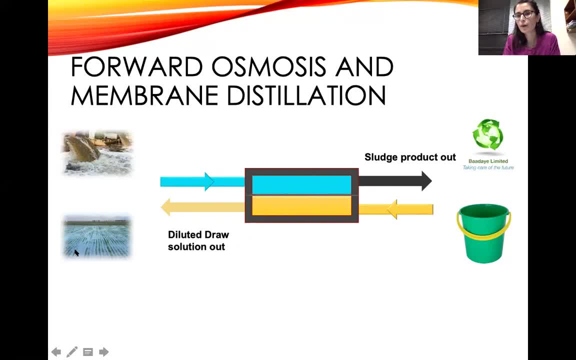 in the fertilizer and then go straight to the farm- not related to what I'm doing right now and in any case not related to my overall PhD, but I just used it as an example. but instead of applying things directly, you just use it in combination and use a certain technology for uh for agriculture. 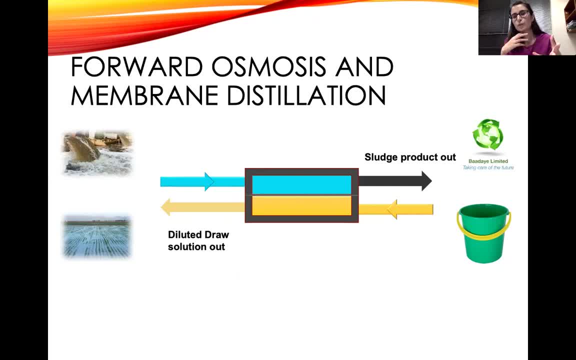 I used surfactants and instead of reverse osmosis worked on the principle of osmosis. so I allowed for these this osmotic potential here. so for the salt, so let's say this is sodium chloride, for the sodium chloride to attract water molecules because of her osmotic potential towards here, and then for only sludge. 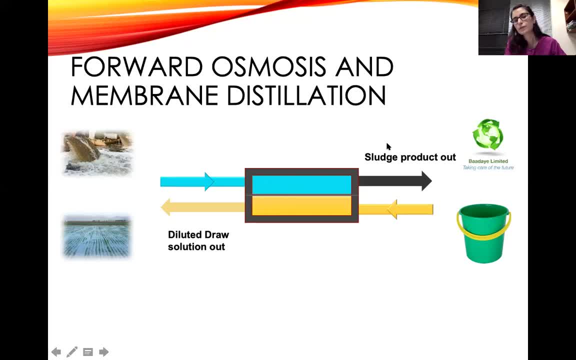 this sludge to concentrate and then be treated and used as fertilizer again, as the um, as the way to uh to extract water from wastewater. so basically, I was just asking for the water to come on the from the wastewater side down to the clean water side where, let's say, I've 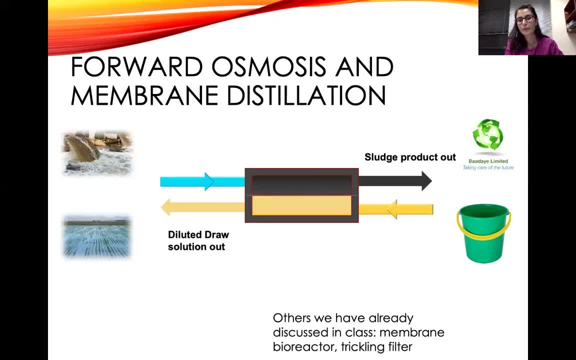 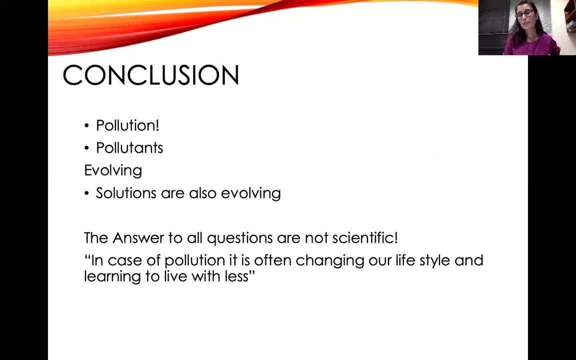 used added sodium chloride and uh, and I'm just going to conclude it here. if if you have any questions, you're more than welcome to ask it. pollutants are evolving, pollution is evolving, their secondary impacts are evolving, the solutions are also evolving and I think there's still a long 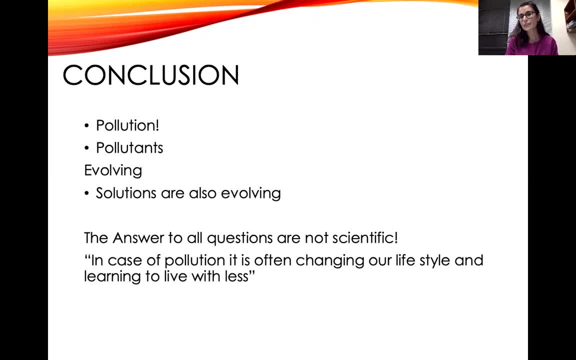 way for us to go. I hope that all of you utilize this knowledge, whatever you've learned. use your voices to you know, to force our governments to to take those strict actions that are required- before you know- we've already messed up with our cities and villages already- but to stop further degradation. 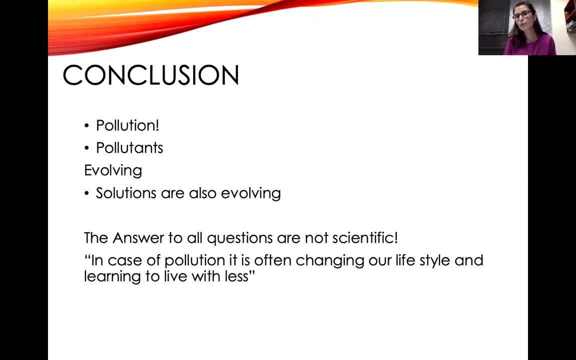 I think we should also stop it and whatever you're doing in your labs, in your small um households, in your practices, just make sure that they are environmentally conscious. and now I can take Rafa's question. sorry for rushing through the last two slides. yes, Rafa, I'm in the second last slide. 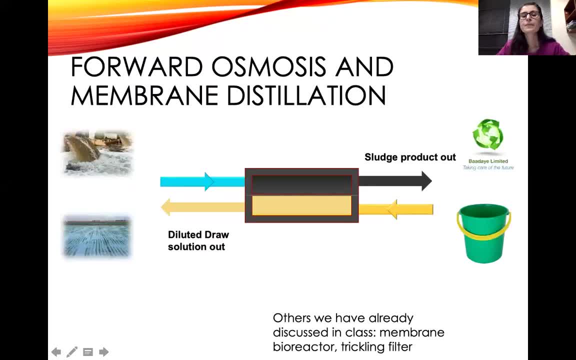 so uh, was your objective to uh use wastewater as fertilizer water? yeah, okay, so I think I'll just okay. so basically my um solution was two prompt. so I was from the sludge, I was taking all the water out, reclaiming the water, because we often say that wastewater is 99.9 percent water, right, 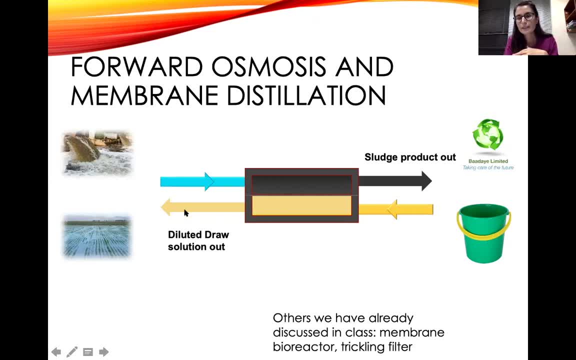 So first step would be to take the water out from this. But instead of the pressure intensive reverse osmosis, I'm using forward osmosis, what we call forward osmosis, where the salt molecules are attracting. you know something we read in childhood: the salt molecules are attracting water molecules from the other side. 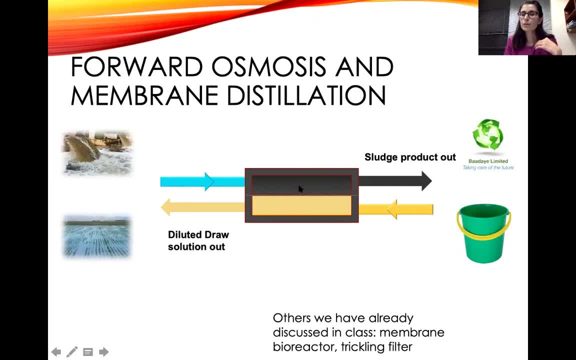 So this highly concentrated salt solution is attracting water molecules from the wastewater and the sludge can be dried out and used, as, for example, this is a company of my friend where they use this as a sludge and fertilizer for agriculture in Kenya, So I just use that example here in the slide. So, yeah, so one part of it is to take as much water out, let that mature and for that to be used as a fertilizer. 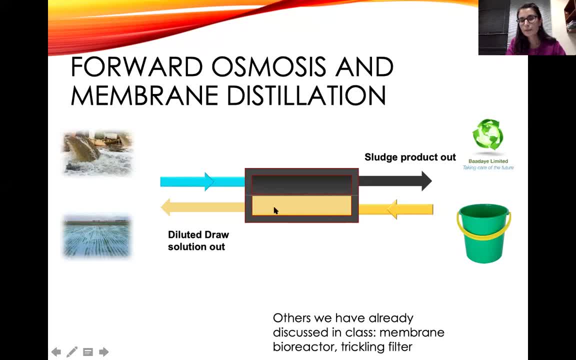 And in the field. And then on the second, Like on the other side of the membrane, I have the salt, which is our osmotic potential, and it's attracting the water molecule. but it was half clean, Right, But because I had in this particular slide, when I prepared it, I was thinking of fertilizers as draw suits. fertilizers can also be used as draw suits, So it's can be used as draw suits. 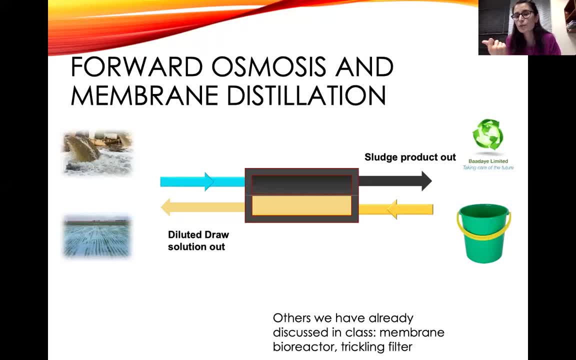 So affectants can be used as draw suits, Polymers can be used as draw suits, and I used all of them. But Once I did this process I had to combine it, because this is half treatment. right now I need to take reclaim this solid out, So for that I added the membrane distillation process. 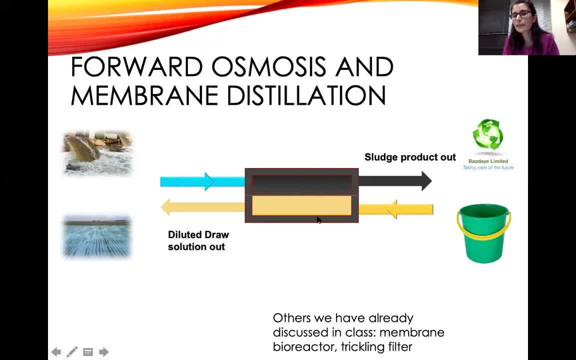 Which basically means that I now, once this is done, then I subject this water to heat, and the water vapors then can go with this memory. So this membrane is water loving, this membrane is water hating, so it's only allowing for water vapors to pass through here. So I'm now, after I do this, I'm heating the stream, And I heat the stream, and fast that I claim all the water in the form of gas. 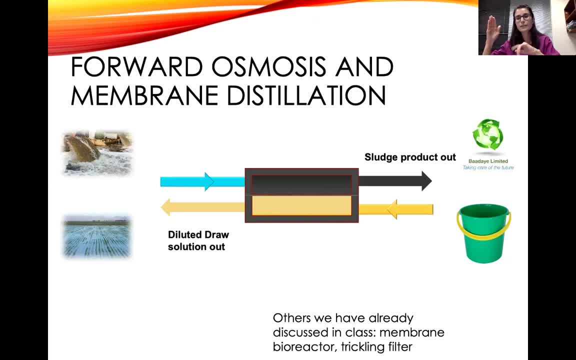 And that goes past the membrane, which wouldn't allow anything else. So sodium chloride is dissolved in it. The temperature: So if this is the membrane, distillation membrane, I have one Feed coming in, so The sodium chloride that was diluted is going here.